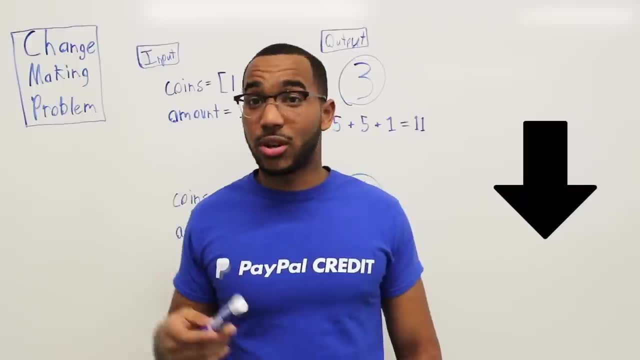 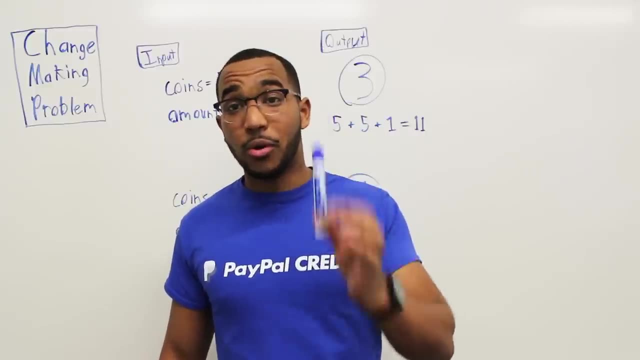 through both and both are in the description. Both code samples are in the description. They're from the LeetCode solutions, but I commented them for clarity so you understand what's going on. So let's walk through both approaches. All right, so we start with the amount 11 and the way we think. 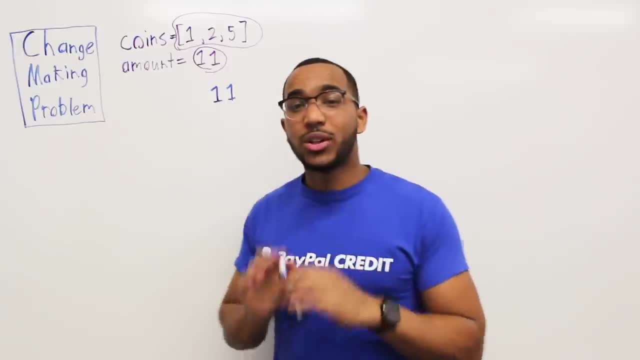 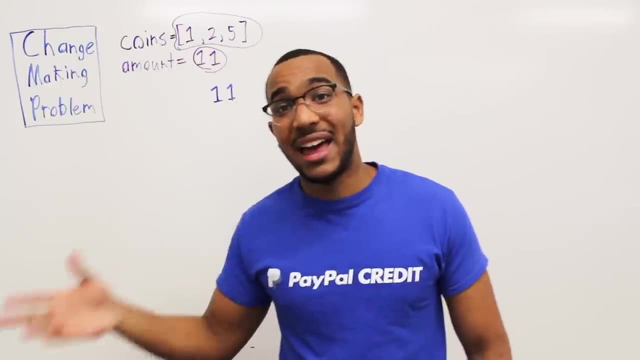 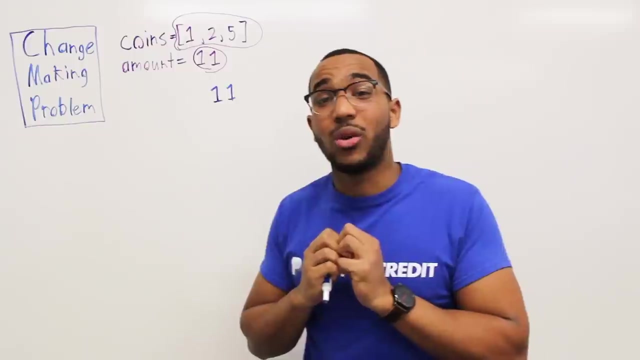 about this problem with dynamic programming is we are going to imagine if five was the last coin that I make change with. I need to make change with whatever is left And the minimum amount of coins would be one plus the amount of ways to make change with whatever is left. So if my last coin I 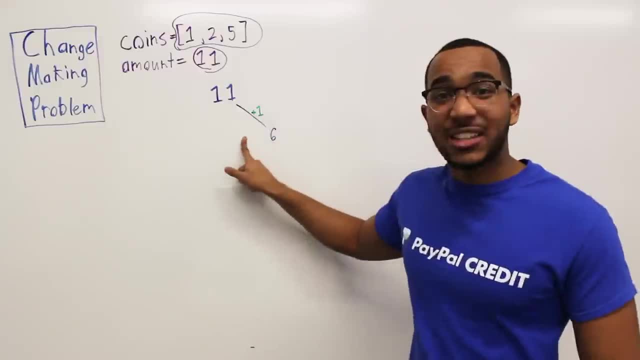 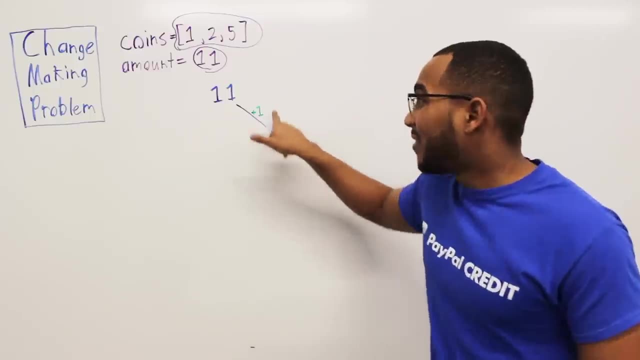 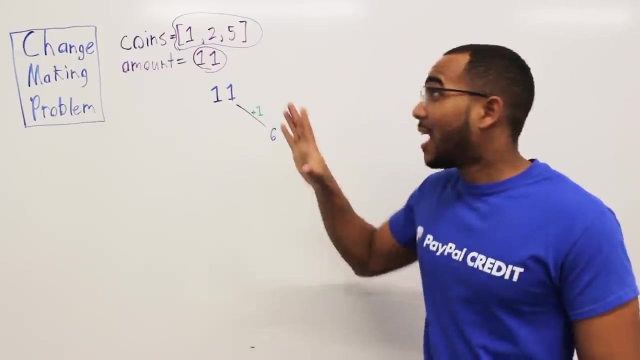 make change with is five. this is what happens. If the last coin that I make change with is five, then that means I subtract five from 11.. 11 minus five is six, And that is one action. I'm picking up the coin I make change with. And now let's pick the two coin to be the last coin we make change with. 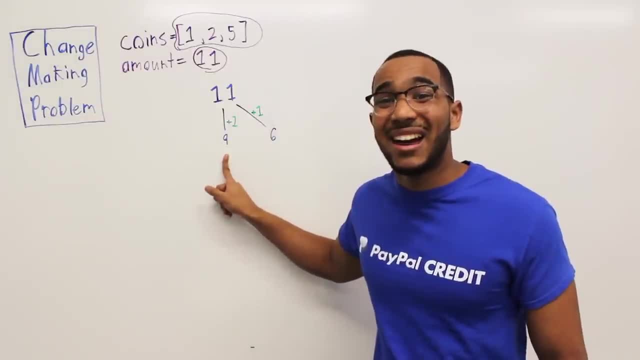 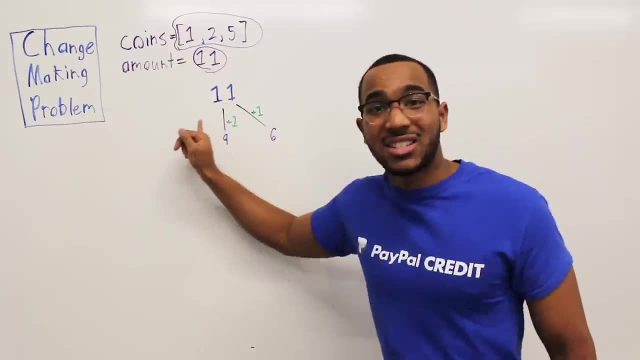 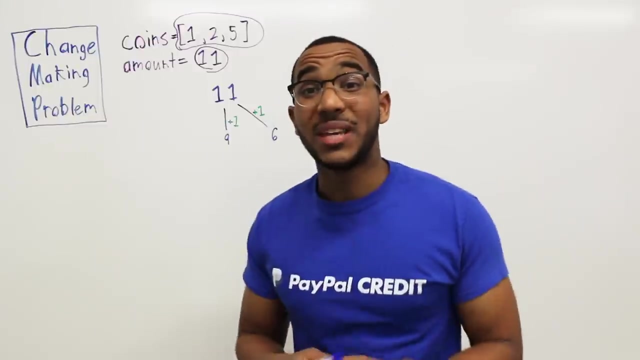 We chose the two coin and you see 11 minus two is nine. So we say one plus the amount of ways we can make change with six, one plus the amount of ways we can make change with nine. This is not how the recursion will do it. The recursion will be doing it depth first And we're going to be caching. 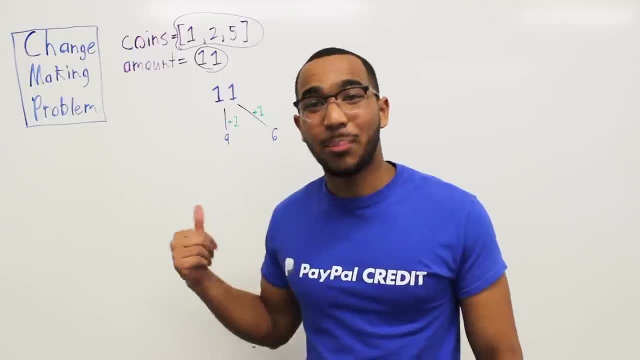 answers along the way, So we remember them. We're going to have duplicate sub problems. It's going to worsen our time complexity. We're going to have duplicate sub problems. And we're going to have duplicate sub problems. And we're going to have duplicate sub problems, So we need to use dynamic. 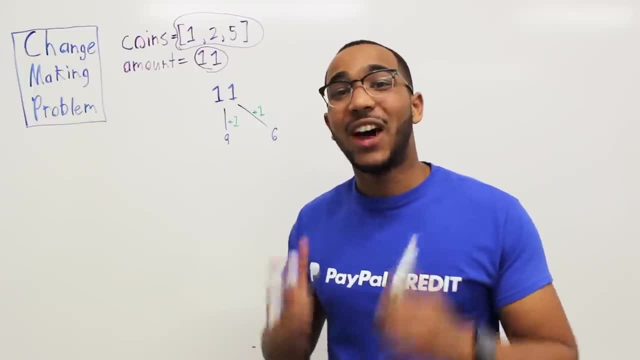 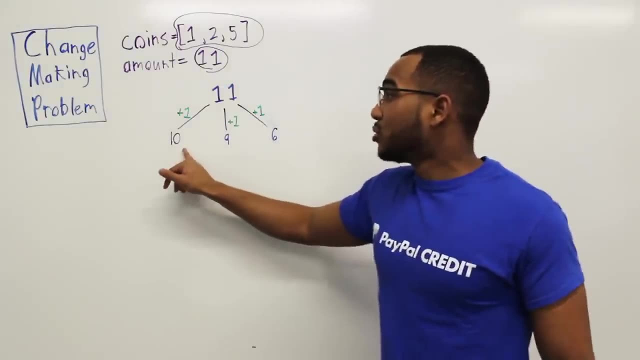 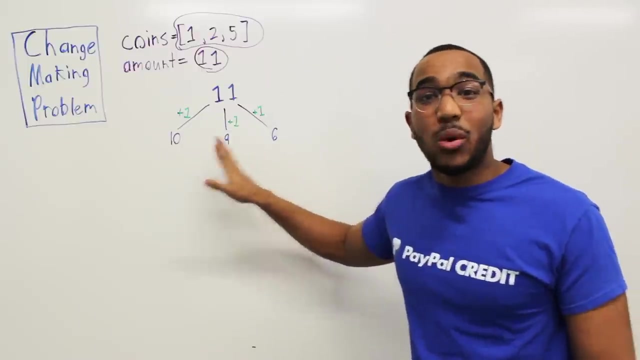 programming to remember those answers. So now, let's try the final coin. Let's try the one as the last coin we make change with. So now do you see, if I use the one as the last coin, if I use the two as the last coin, if I use the five as the last coin, this is what the 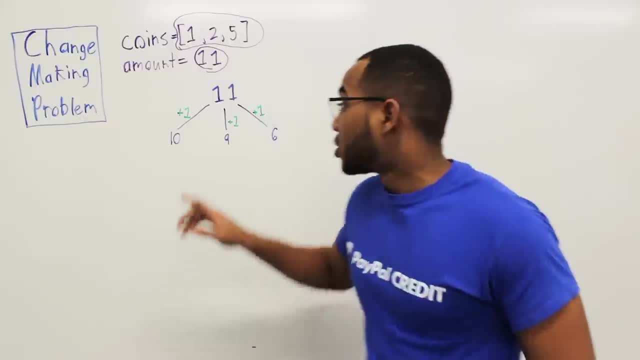 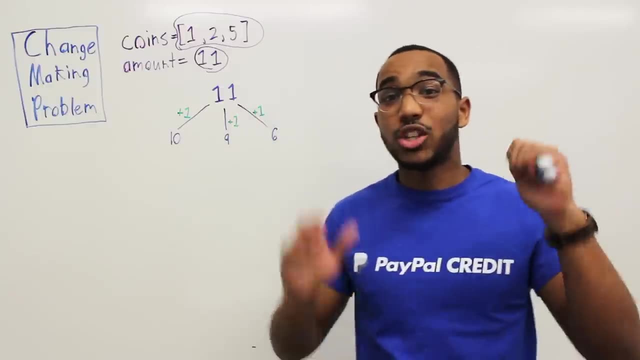 paths will look like. Some of them will not pan out. I might not be able to make change for nine. I might not be able to make change for 10.. Each of these paths will have a length. We want the shortest path that is valid, That is going to yield us a path that makes change with the minimum. 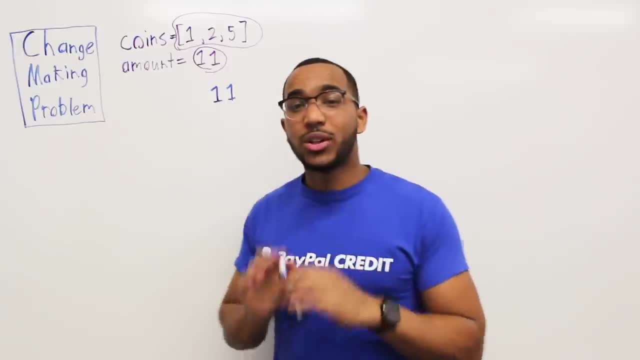 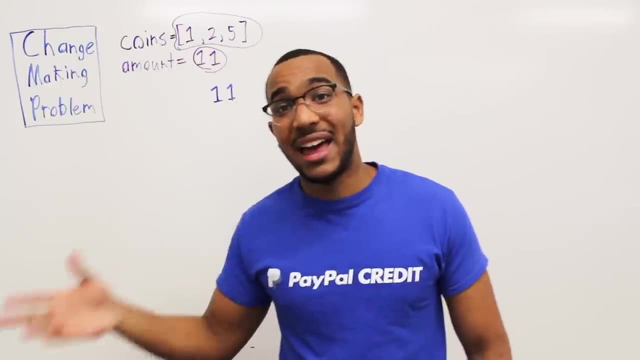 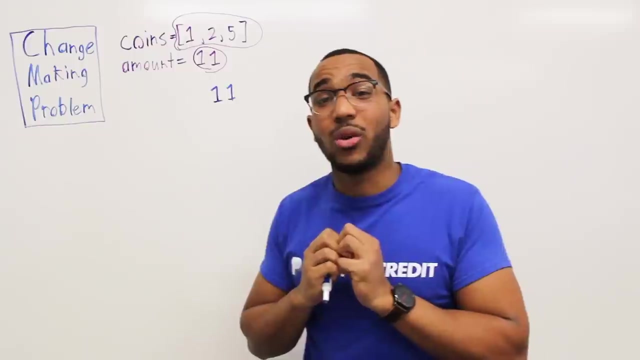 about this problem with dynamic programming is we are going to imagine if five was the last coin that I make change with. I need to make change with whatever is left and the minimum amount of coins would be one plus the amount of ways to make change with whatever is left. So if my last coin I 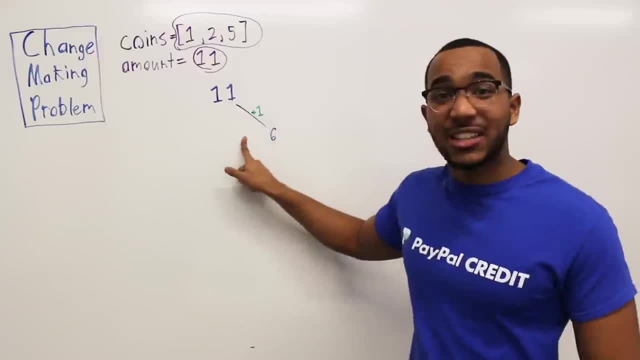 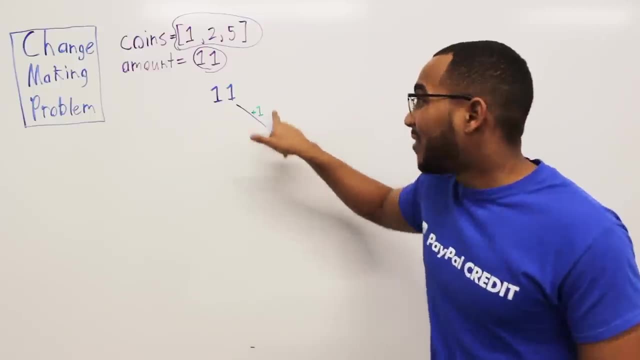 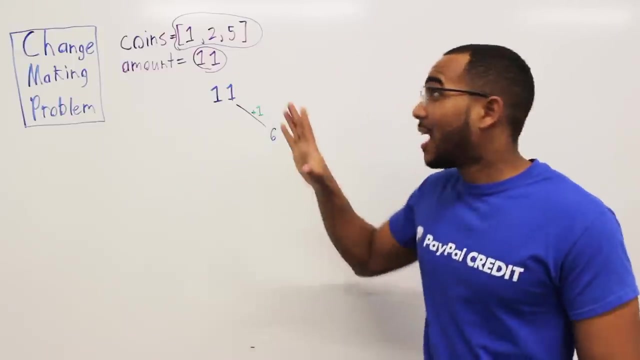 make change with is five. this is what happens. If the last coin that I make change with is five, then that means I subtract five from 11.. 11 minus five is six, and that is one action. I'm picking the coin that I make change with, and now let's pick the two coin to be the last coin we make. 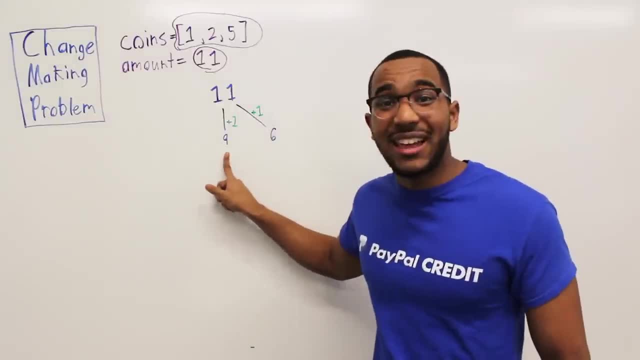 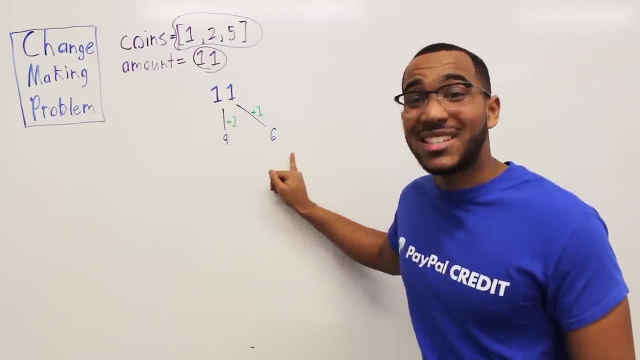 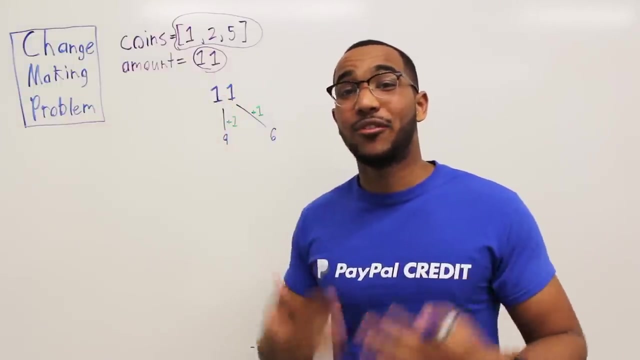 change with. We chose the two coin and you see 11 minus two is nine. So we say one plus the amount of ways we can make change with six, one plus the amount of ways we can make change with nine. This is not how the recursion will do it. The recursion will be doing it depth first, and we're going to be 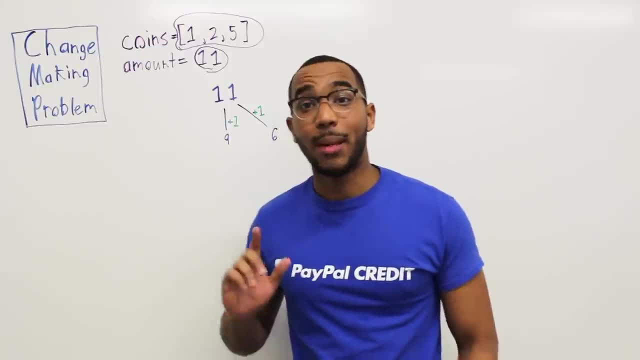 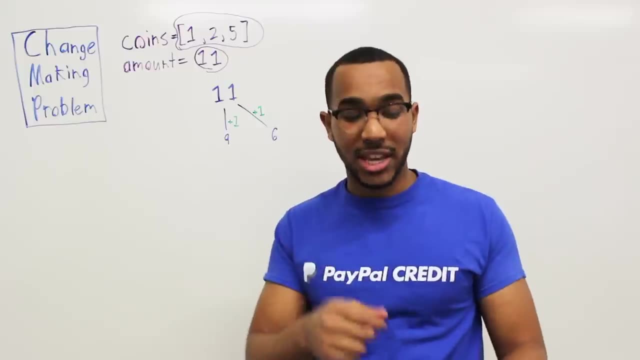 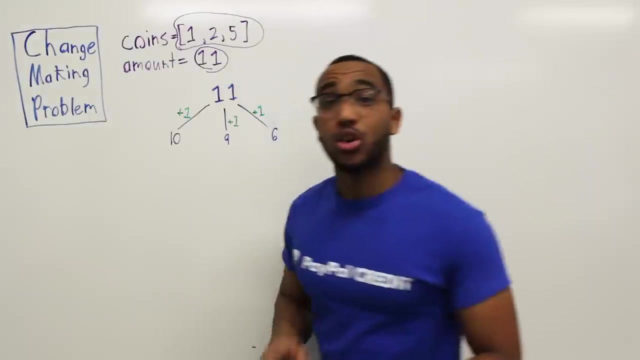 caching answers along the way So we remember them. We're going to have duplicate sub problems. It's going to worsen our time complexity, So we need to use dynamic programming to remember those answers. So now let's try the final coin. Let's try the one as the last coin We make change with. so now, 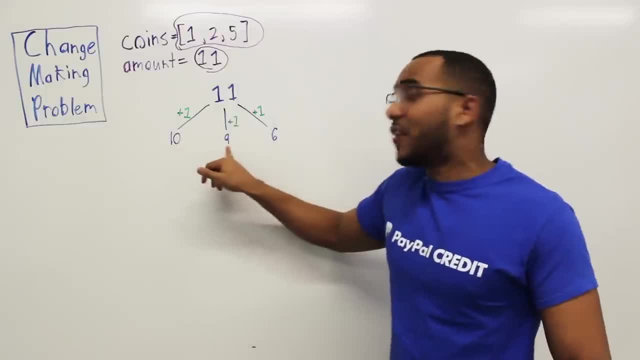 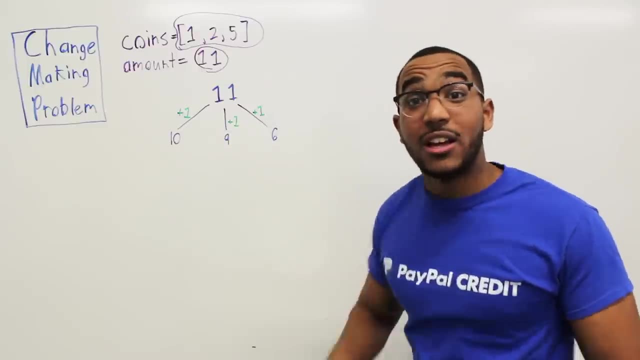 Do you see, if I use The one is the last point, if I use the two as the last point, if I use the five as the last point, This is what the paths will look like. some of them will not pan out. I might not be able to make change for nine. 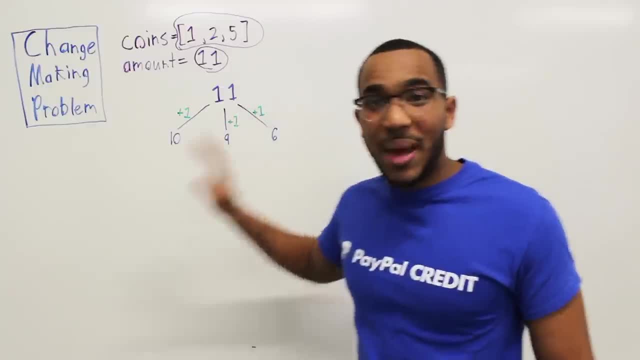 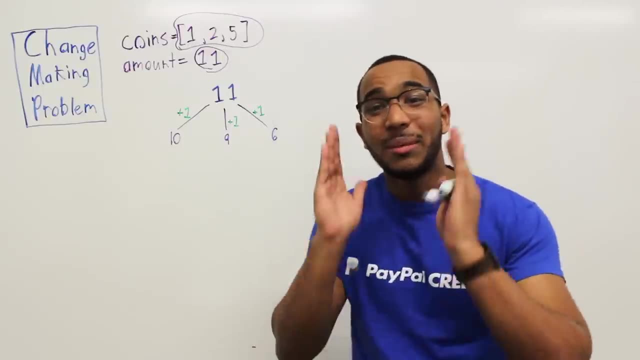 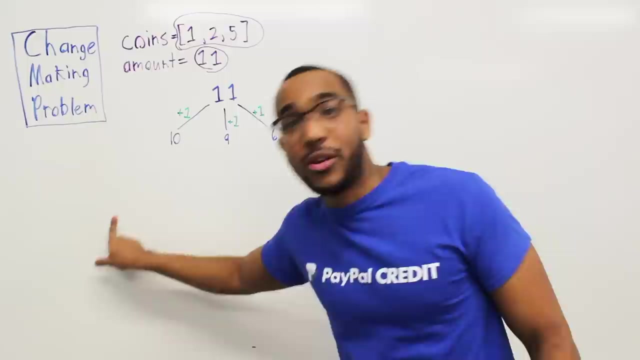 I might not be able to make change for ten. each of these paths will have a length. We want the shortest path that is valid, that is going to yield us a path that makes change with the minimum amount of coins. As you can tell, we're going to be going very deep on this path because subtract one from ten, subtract one from ten, subtract one. 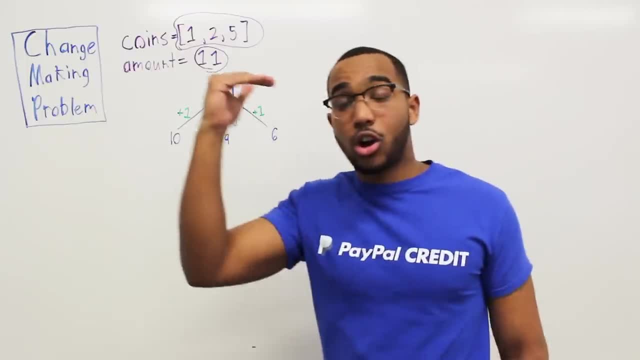 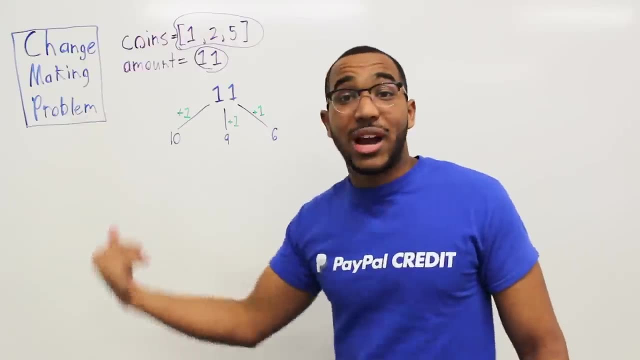 From ten. we'll do that eleven times, And that's why our call stack will have a depth of O of n, Because n is the amount. and then we're going to have to go that deep if we just have to subtract ones every time. But let's do that again. 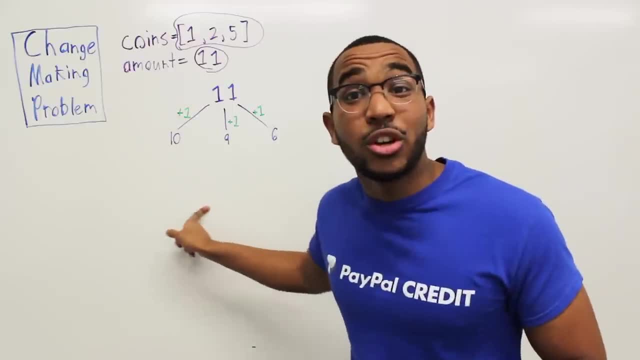 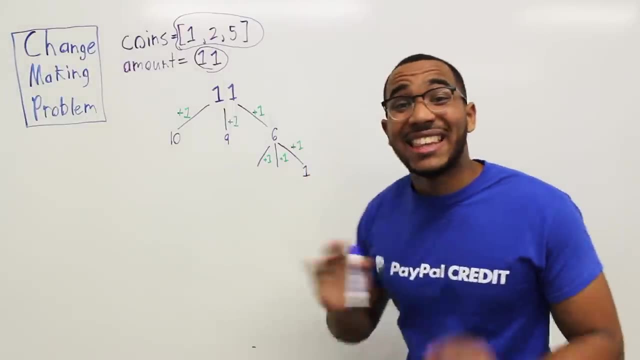 Let's see how we can make change from each one Of these new points, each one of these new sub problems. So, as you can see here, I subtracted five from six. if the last coin I make change with for six is five, Then I subtract five from six and I get one now. 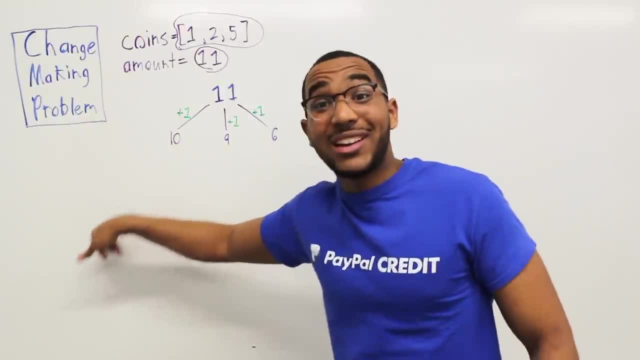 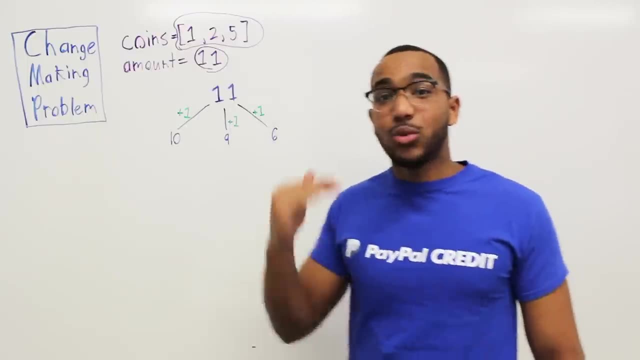 amount of coins. As you can tell, we're going to be going very deep on this path, because subtract one from 10,, subtract one from 10,, subtract one from 10.. We'll do that 11 times, And that's why. 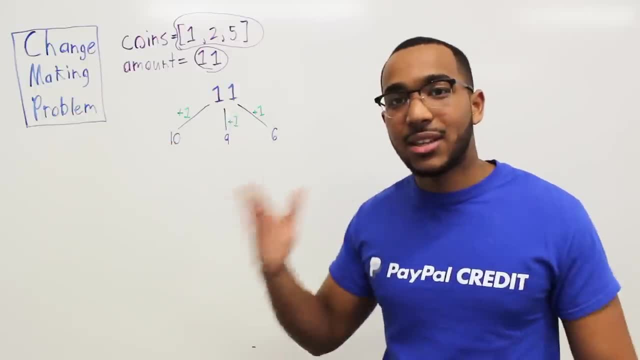 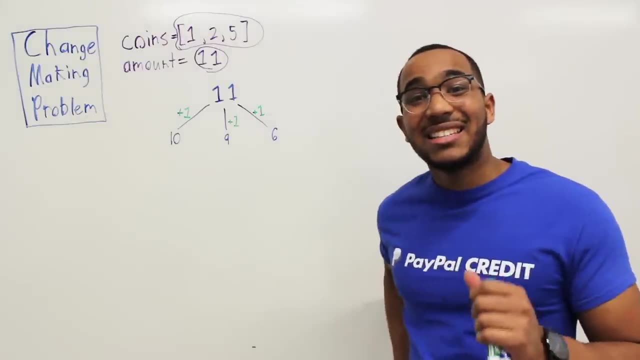 our call stack, will have a depth of O, of N, because N is the amount, And then we're going to have to go that deep if we just have to subtract ones every time. But let's do that again. Let's see how we can make change from each one of these. 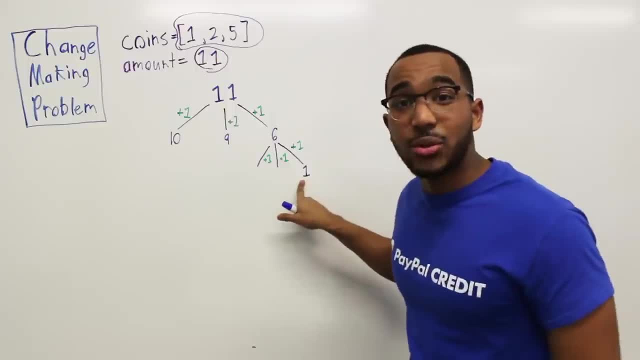 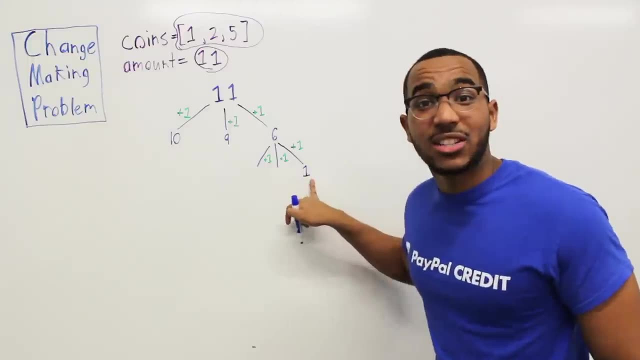 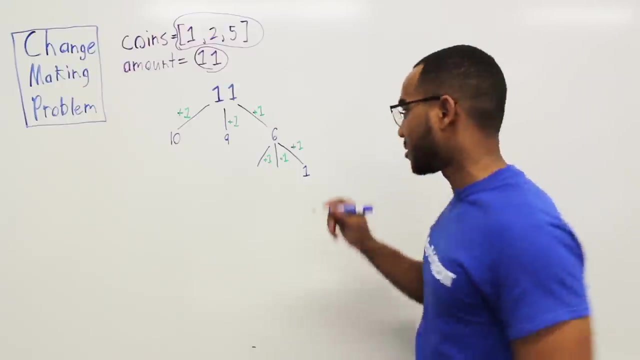 New points, each one of these new sub problems. So, as you can see here, I subtracted five from six. If the last coin I make change with for six is five, then I subtract five from six and I get one. Now let's try the two coin as the last coin to make change for six. And now we have four left. 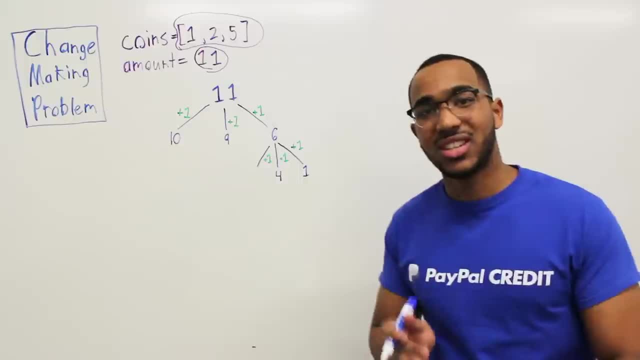 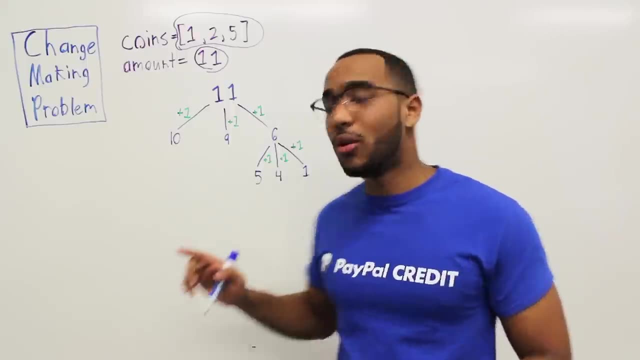 Now let's try one as the last coin. we make change for six And now we have five And notice, these are our new sub problems. Our winning subtree is going to be over here. If I solve the sub problem, how many ways are there to make change for one? 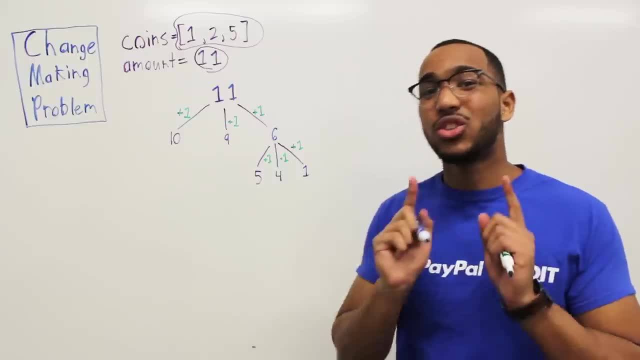 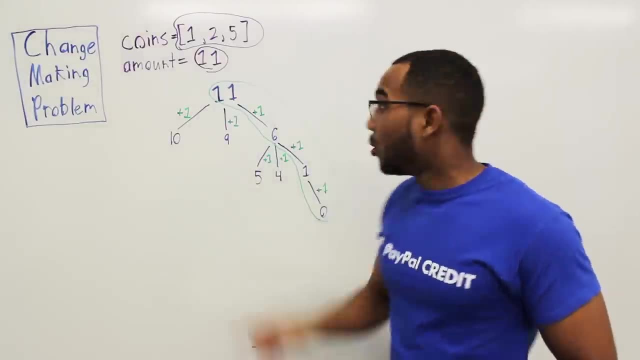 With the coins we have, I only can use the one coin. Let's use the one coin. And now I want you to see: this is the winning sub problem, This is the winning path. We do one, one, one, three coins. 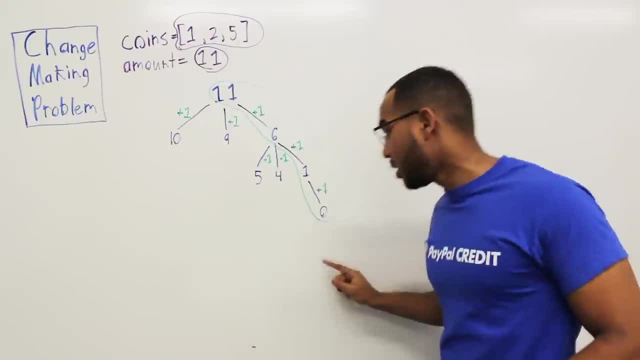 We used a five, We used a five, We used a one And now we have reached zero. That means we made change. It was a valid path, And now we know that we're going to make change for six, And now we're. 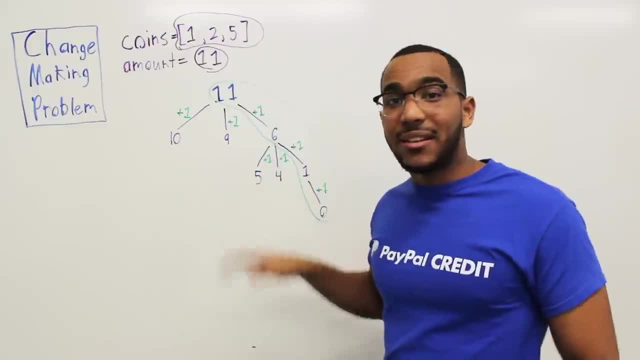 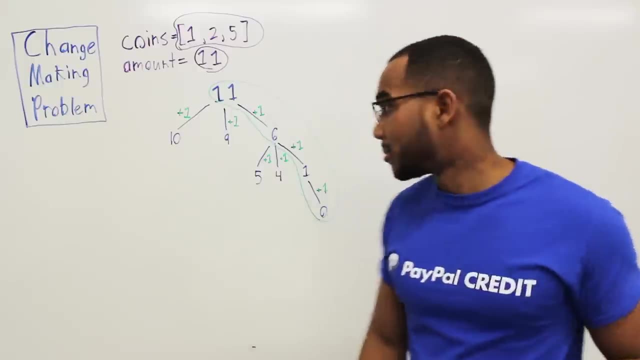 going to know. the minimum way to make change is going to be three. There's other paths we could take, So let's keep enumerating the paths. So I want you to see how we're going to duplicate sub problems. So now let's branch from the nine Again. this is not how the code would do it. 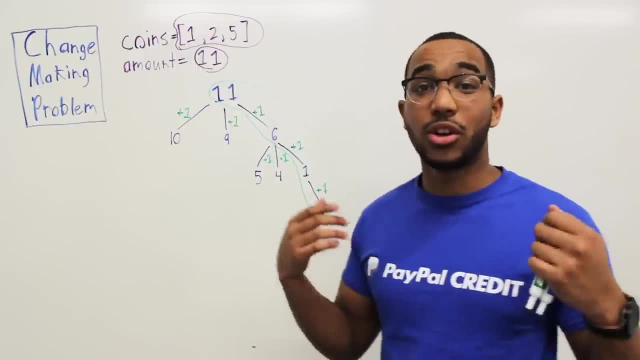 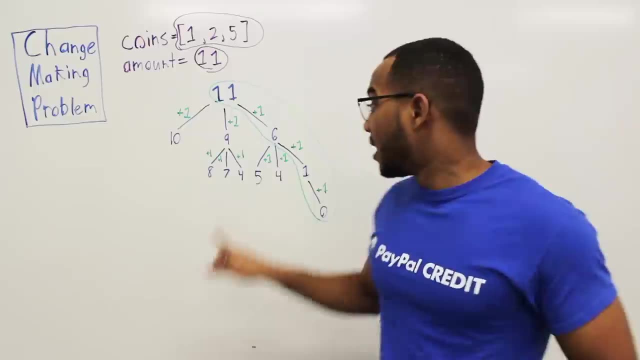 I just want you to see how this tree looks before you even look at the code, so it can be helpful. So do you see here, if I use five as the last coin to make change for nine, I will have four left. If I use two as the last coin to make change for nine, 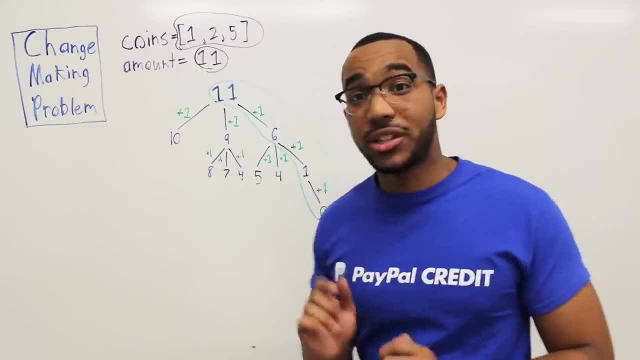 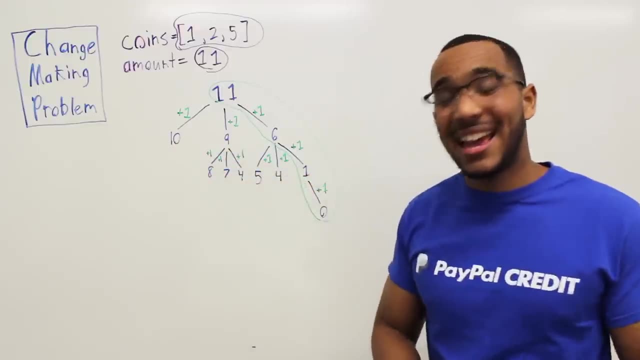 I have seven left. If I use one as the last coin to make change for nine, I have eight left. And now let's branch one more time for 10.. Let's see the branching for 10.. We see if we use five. 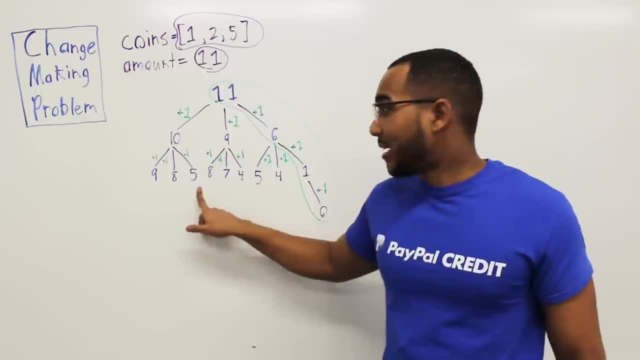 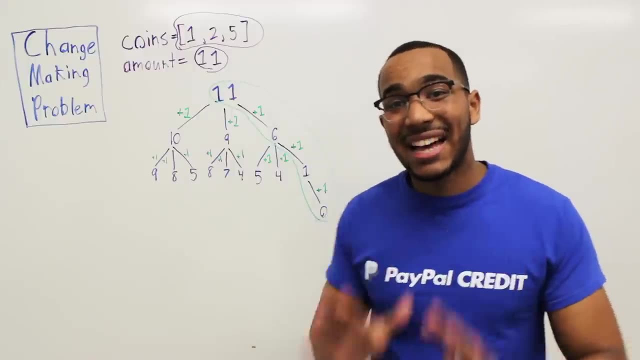 as the last coin to make change for 10,, we'll have five left. If we use two as the last coin to make change for 10,, we'll have eight left If we use one as the last coin to make change for 10,. 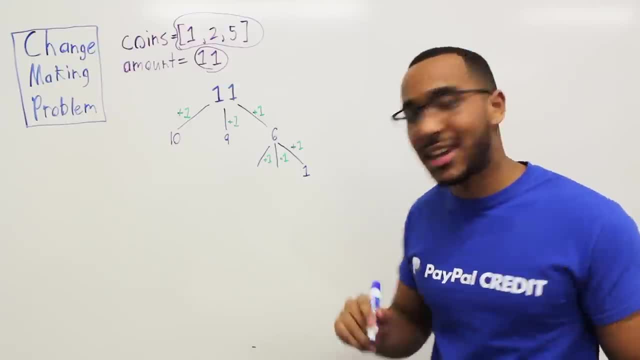 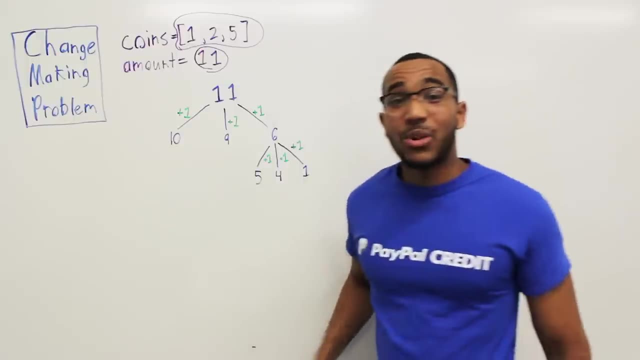 Let's try the two coin as the last coin to make change for six, and now we have four left. now Let's try one as the last coin we make change for six, and now we have five. and notice, These are our new sub problems, our winning sub tree. 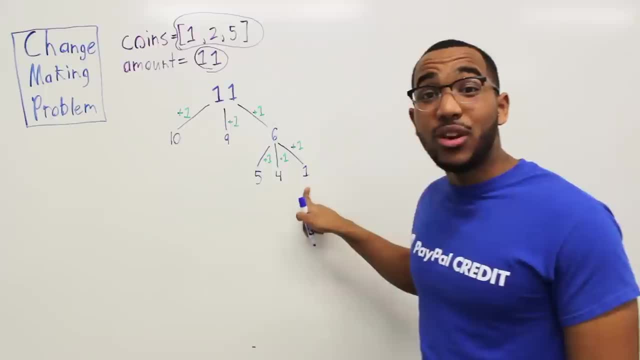 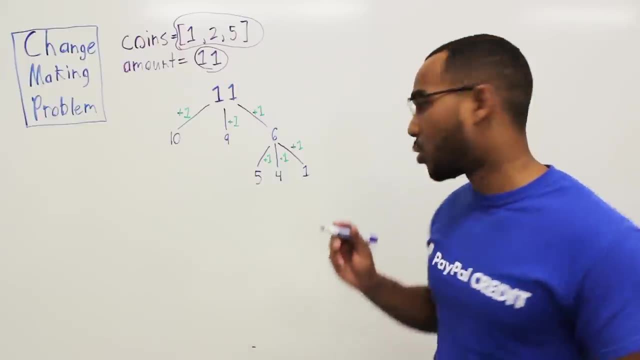 Is going to be over here if I solve the sub problem. How many ways are there to make change for one with the coins we have? I only can use the one coin. Let's use the one coin. and now I want you to see: this is the winning sub problem. 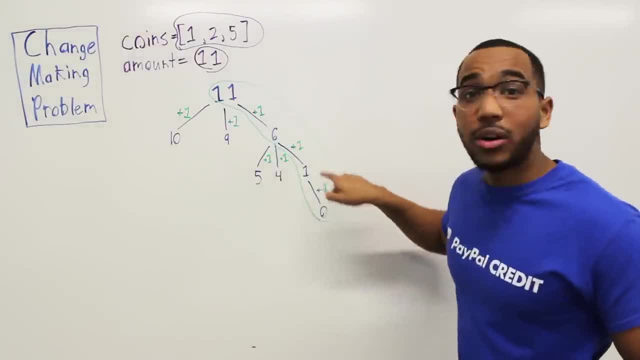 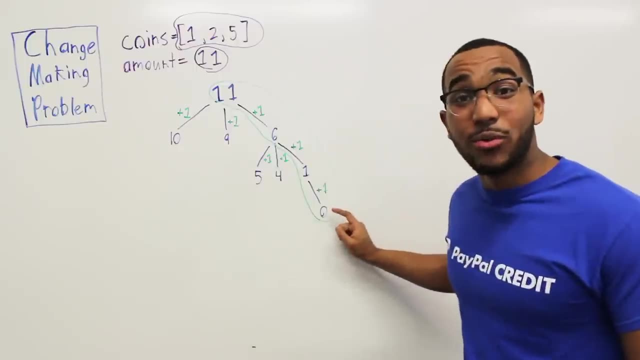 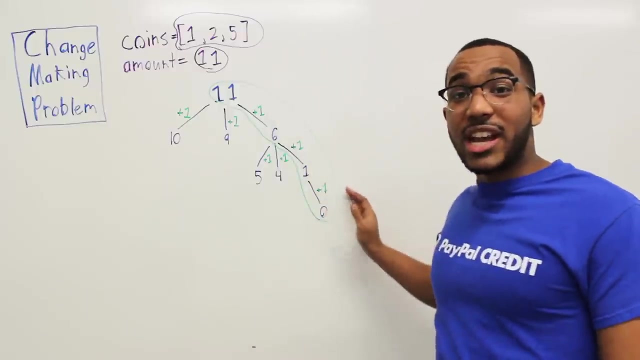 This is the winning path. we do one, one, one, three coins. we used a five, we used a five, we used a one and Now we have reached zero. that means we made change. it was a valid path And now we know the minimum way to make change is going to be three. 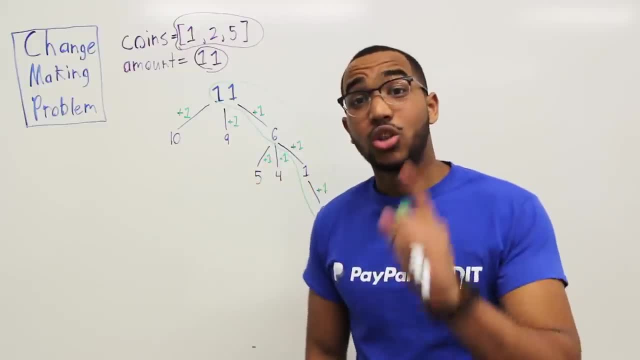 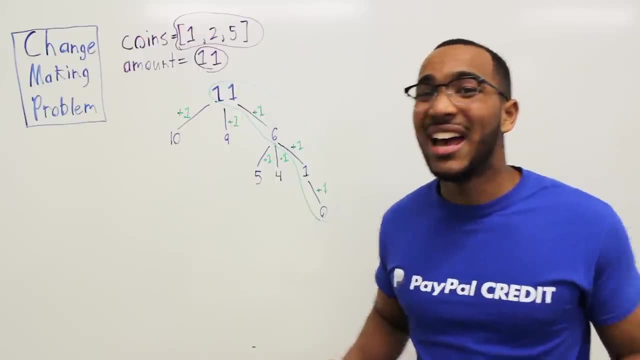 There's other paths we could take. So let's keep enumerating the paths. So I want you to see how we're going to have duplicate sub-problems. So now let's branch from the nine Again. this is not how the code would do it. 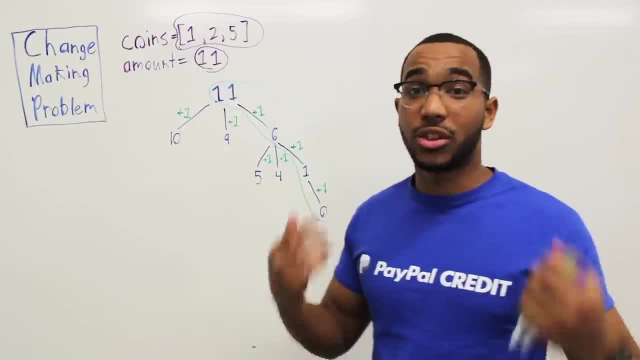 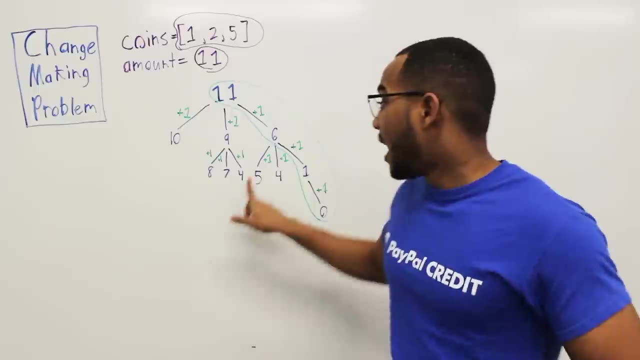 I just want you to see how this tree looks before you even look at the code, so it can be helpful. So do you see here, If I use five as the last coin to make change for nine, I will have four left. If I use two as the last coin to make change for nine, 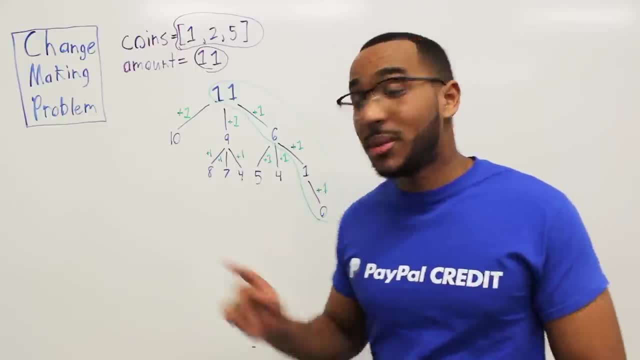 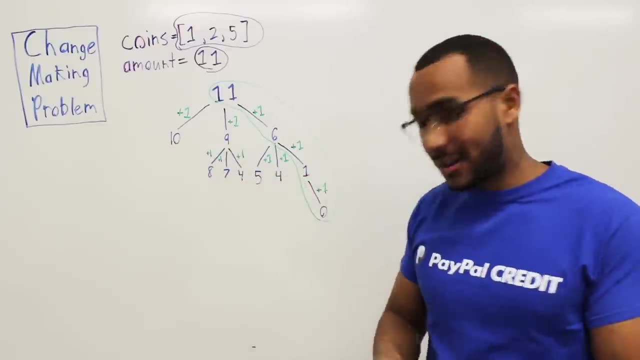 I have seven left. If I use one as the last coin to make change for nine, I have eight left. And now let's branch one more time for 10.. Let's see the branching for 10.. We see if we use five as the last coin. 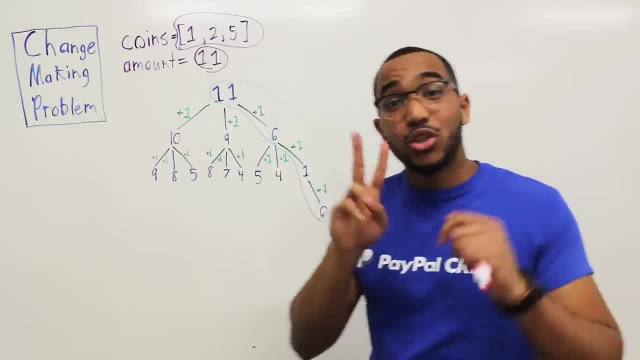 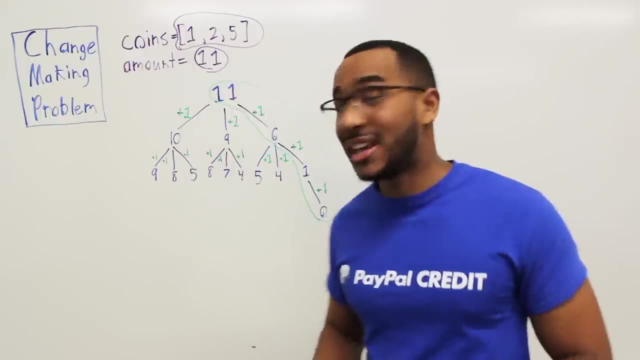 to make change for 10, we'll have five left. If we use two as the last coin to make change for 10, we'll have eight left. If we use one as the last coin to make change for 10, we will have nine left. 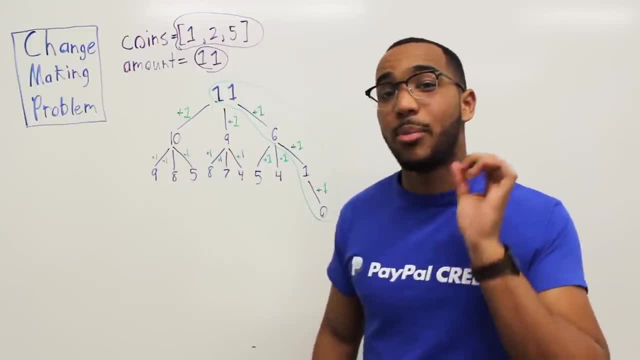 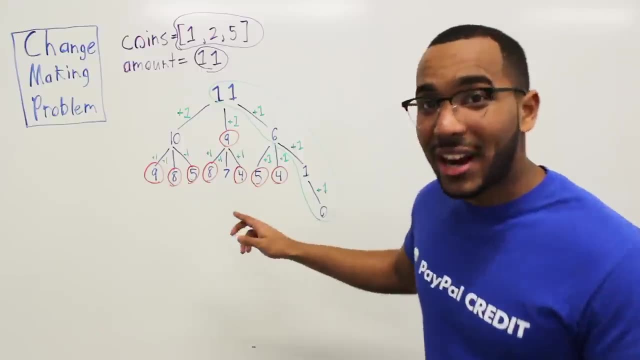 I want you to notice something. Here's why this problem is dynamic programming. We haven't even finished our recursion tree, We haven't even gotten halfway through it and we see: do you see all the red? I circled. Do you see all of these duplicate sub-problems? 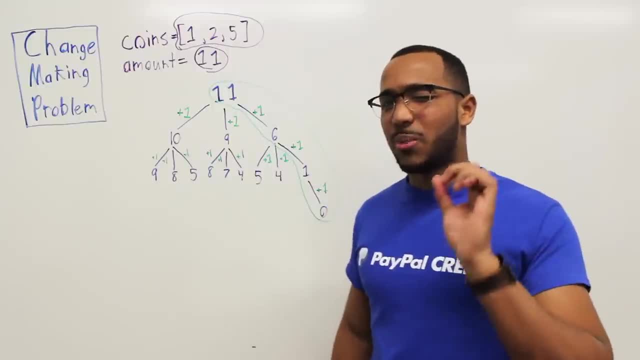 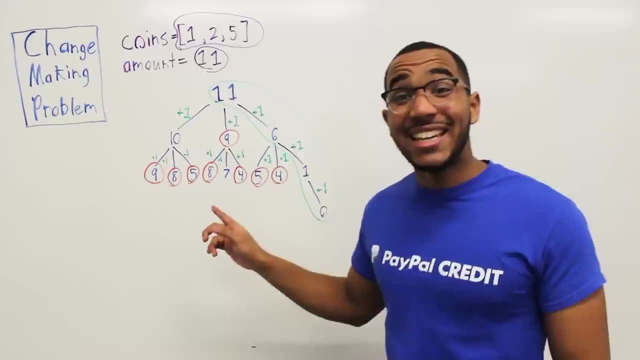 we will have nine left. I want you to notice something. Here's why this problem is dynamic programming. We haven't even finished our recursion tree, We haven't even gotten halfway through it And we see, do you see all the red? I circled. Do you see all of these duplicate? 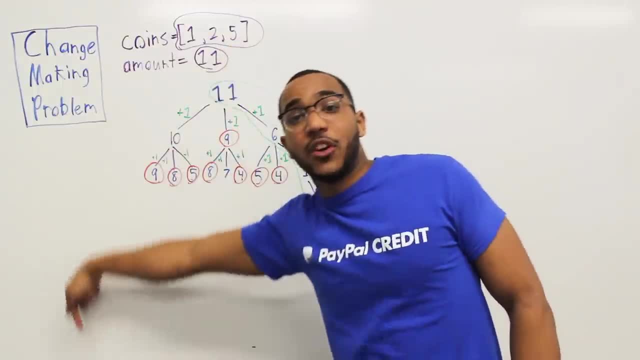 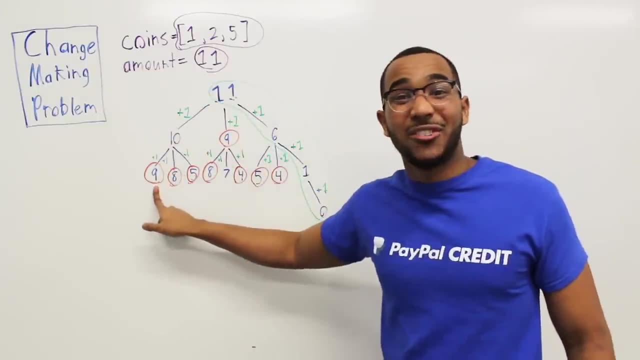 sub-problems When we do our recursion. we're going to go depth first down this way. This part is going to come near the end, but we're going to go depth first down this way. We'll already have the answer for nine. Why am I solving it over here? We will already have the answer for eight. 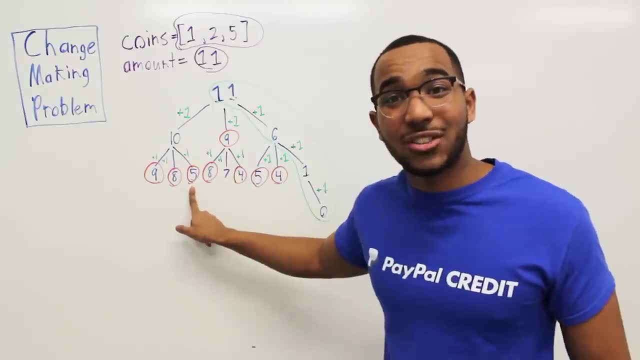 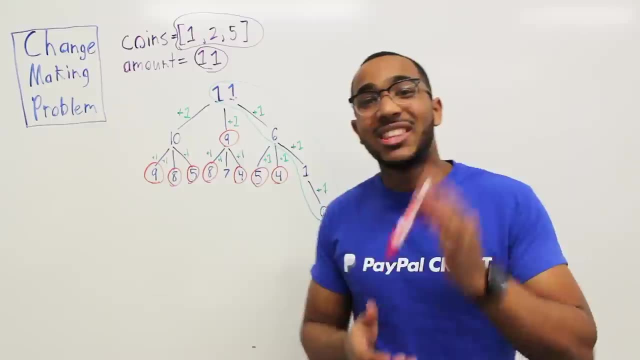 Why am I solving it over here? We will already have the answer for five. Why am I solving the ways to make change for five, when I will already know the answer? This is why this is dynamic programming. This is the top down approach. We start from the top. Say, if I use this, 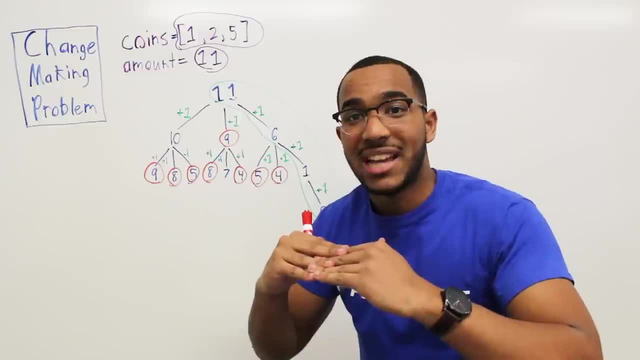 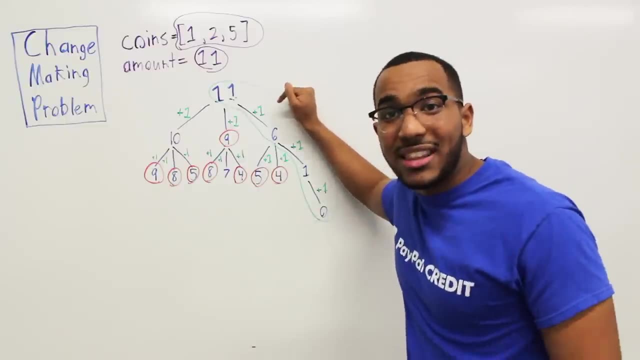 this, this coin. how many ways can I make change going downwards If I use this, this, this coin from those nodes? how many ways to make change And the path that is the shortest, the path that has the shortest length, is going to win The fewest coins to make change from a certain? 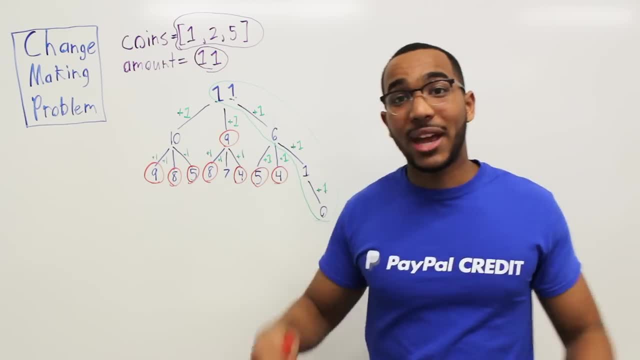 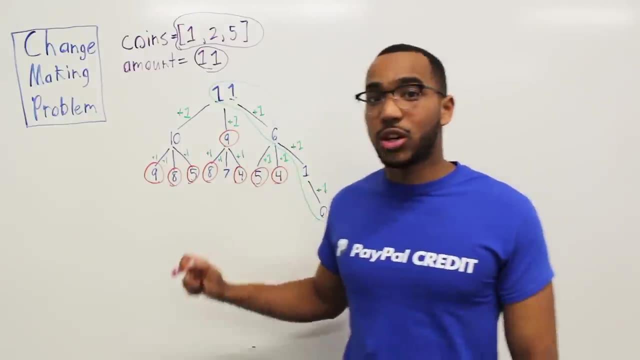 node is going to win and that answer is going to bubble up and we are going to have our notary public loan bank by now. Answer At the top level. this is the top down approach. you can finish. tracing this recursion tree is very simple. We only try the coins that we actually can use as 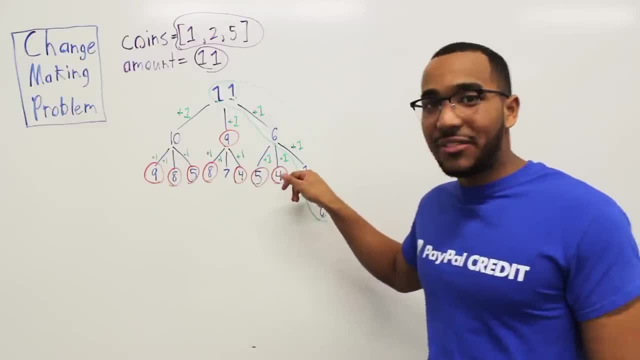 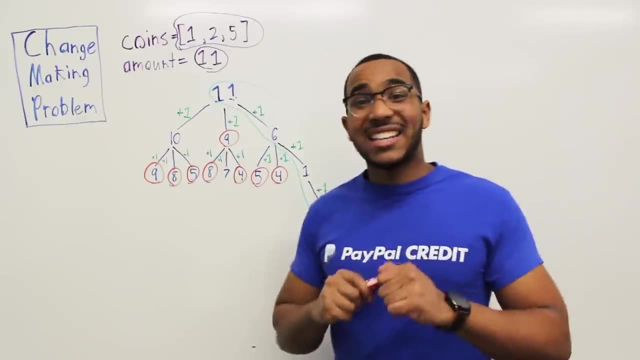 the last coin. For example, I won't be able to use the coin 5 here, because making change for one, I can't use five, making change for four, I can not use the five point. So that is how this problem works. It's about branching, exploring all possibilities to deputy but the disadvantages of not using 5, I don't use five. If I made change to 4 in this, which I didn't channel, so why can I use that for four right And can't use it on all? I do that with my counting with 5 and 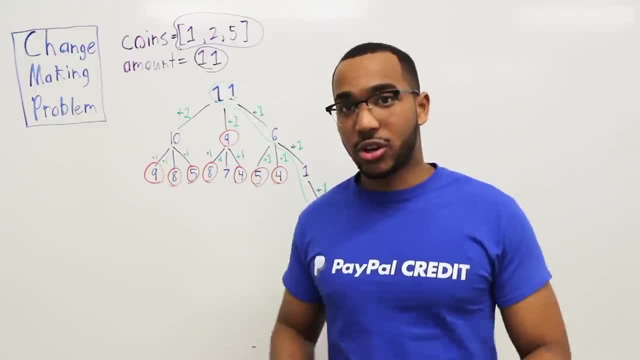 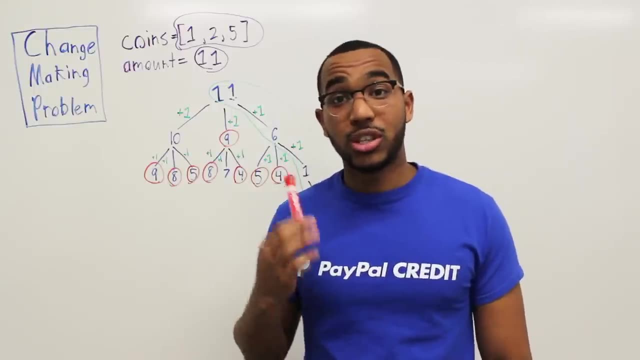 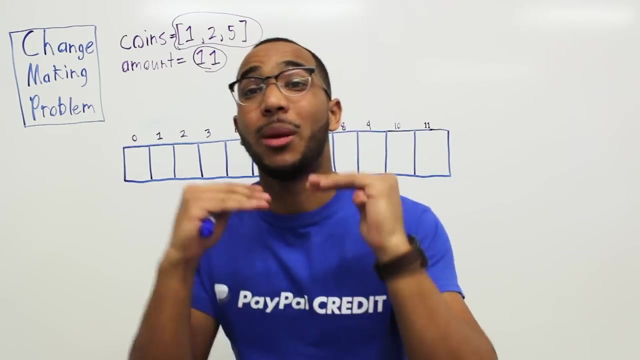 exploring all our possibilities, remembering the answers and then finding the globally optimal solution. Now let's look at the bottom-up approach to this problem. This is top-down And, again, both of these are in the description for you to look at, fully commented. So here is the bottom-up approach. We are not 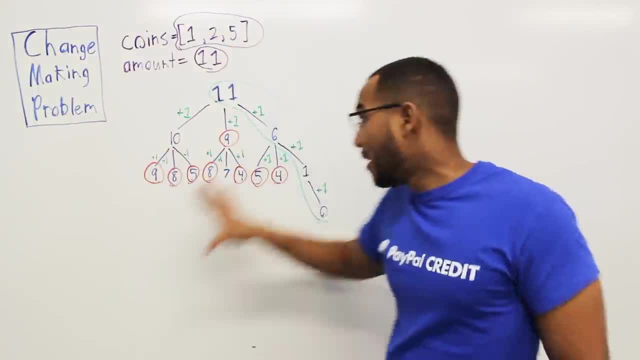 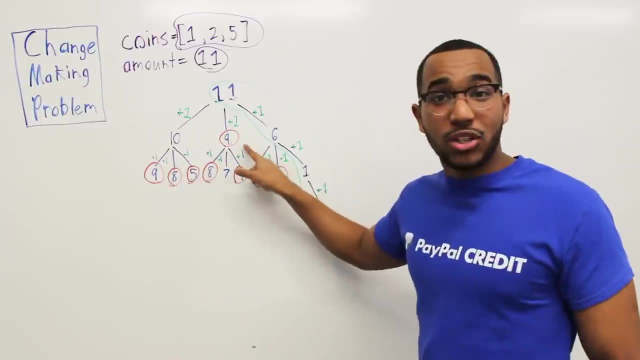 When we do our recursion. we're going to go depth first down this way. This part is going to come near the end, but we're going to go depth first down. this way, We'll already have the answer for nine. Why am I solving it over here? We will already have the answer for eight. 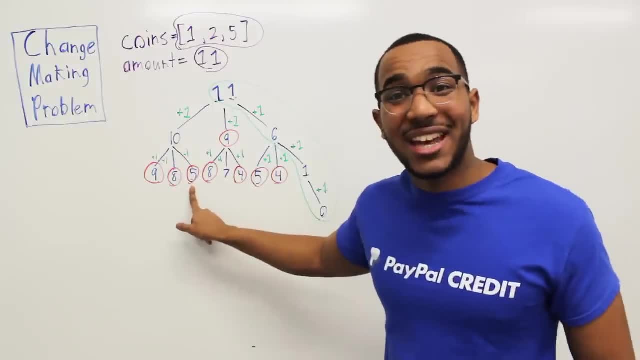 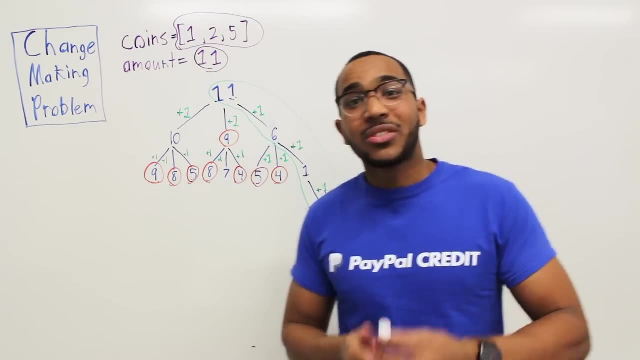 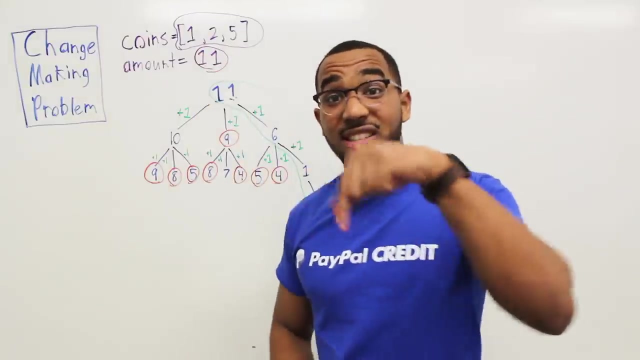 Why am I solving it over here? We will already have the answer for five. Why am I solving the ways to make change for five, when I will already know the answer? This is why this is dynamic programming. This is the top down approach. We start from the top. Say, if I use this, this: 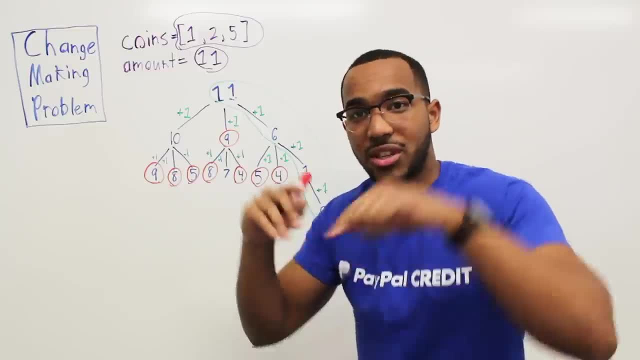 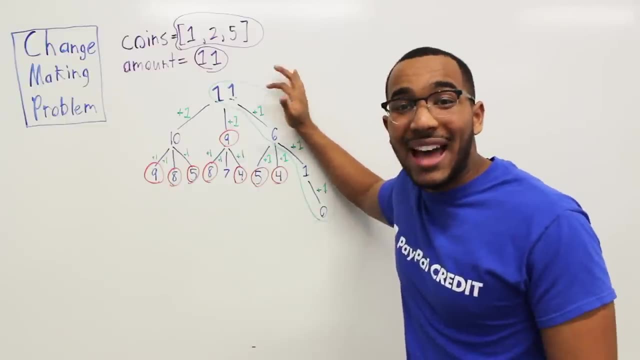 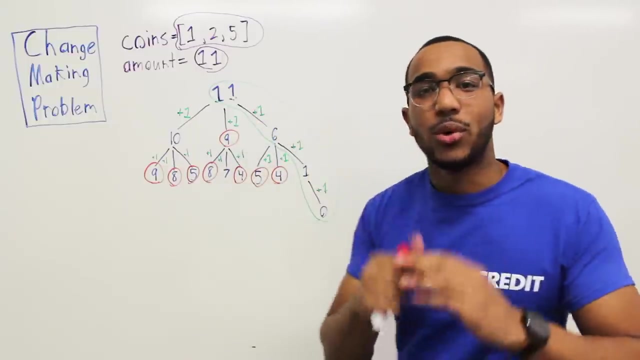 this coin. how many ways can I make change going downwards If I use this, this, this coin from those nodes? how many ways to make change And the path that is the shortest, the path that has the shortest length, is going to win, The fewest coins to make change from a certain node is going to win And that 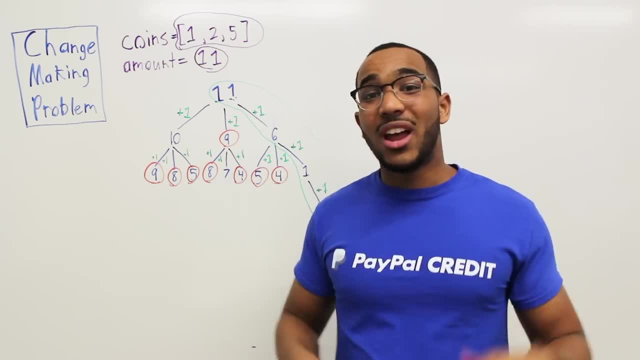 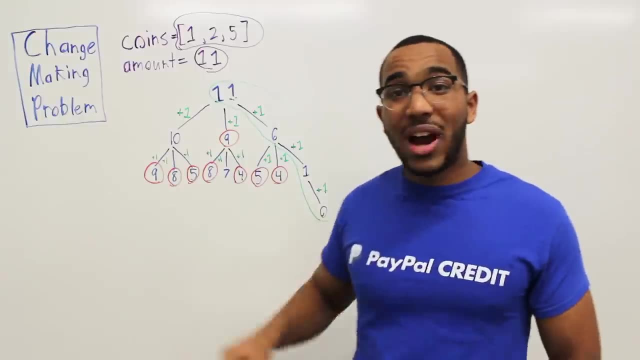 answer is going to bubble up and we are going to have our answer at the top level. This is the top down approach. You can finish tracing this recursion tree. It's very simple. We only try the coins that we actually can use. at the last coin, For example, I won't be able to use the coin five. 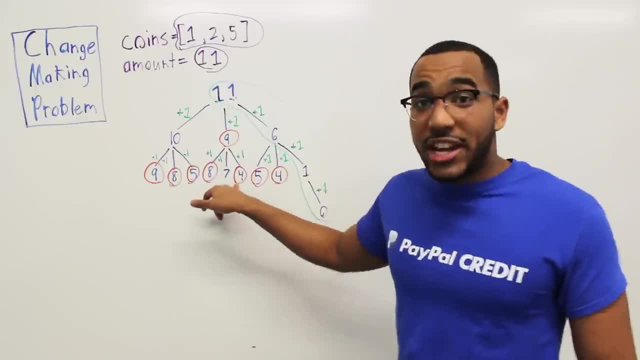 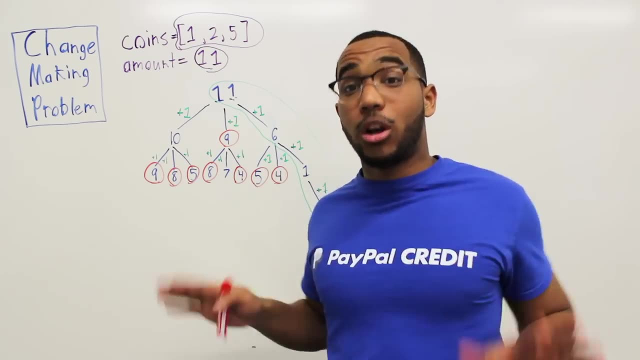 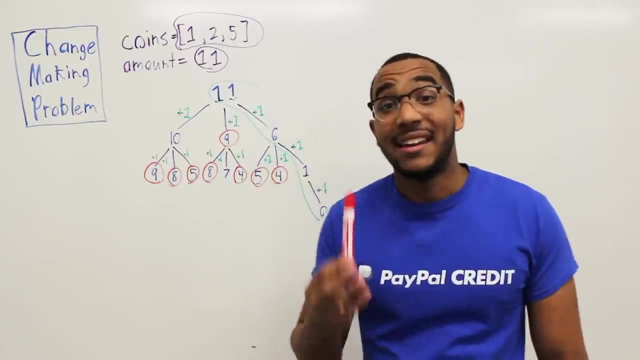 here, because making change for one, I can't use five. Making change for four, I cannot use the coin five. So that is how this problem works. It's about branching, exploring all our possibilities, remembering the answers and then finding the globally optimal solution. Now let's look at the 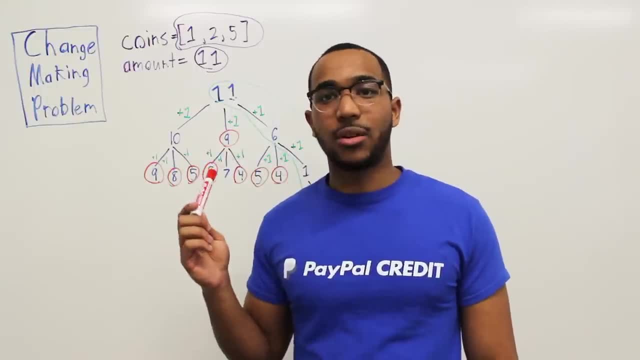 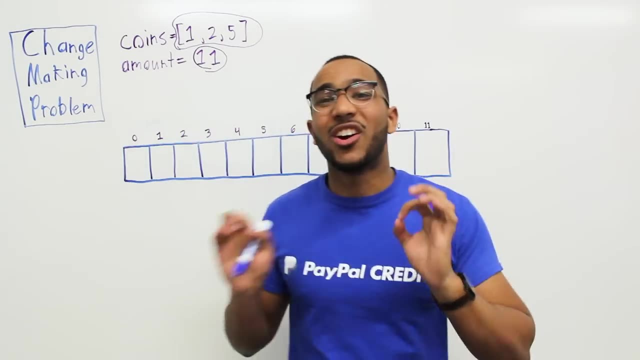 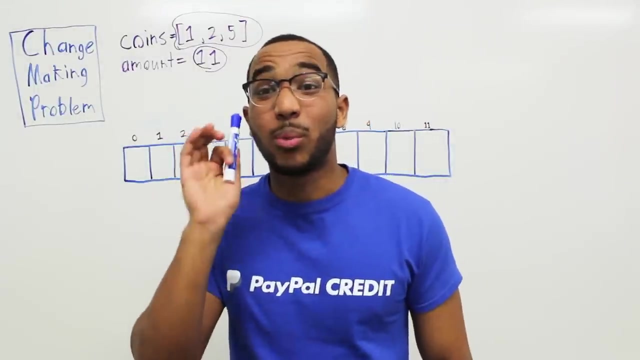 bottom up approach to this problem. This is top down And again, both of these are in the description for you to look at, fully commented. So here is the bottom up approach. We are not changing our psychology. We are not changing how we think about this problem. We are changing the way we approach. 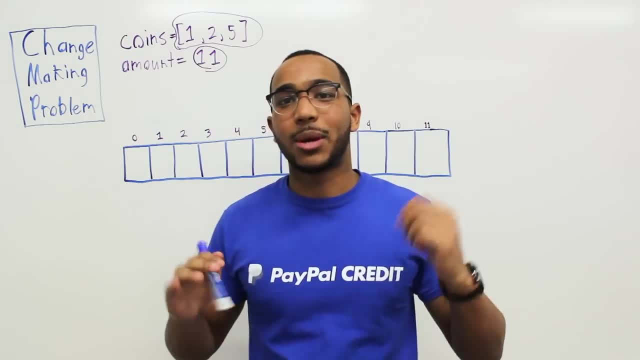 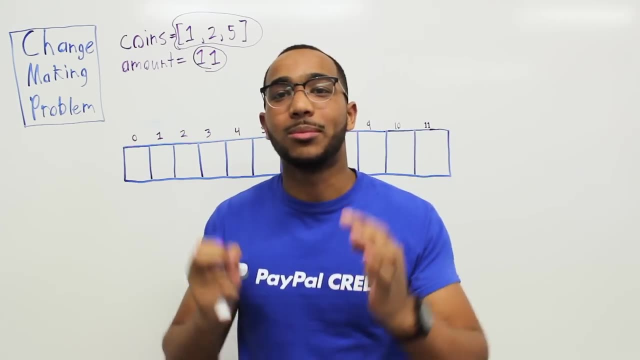 this problem. If there is one thing I ask of you doing these dynamic programming questions: do not memorize the table, Do not memorize the way these relate. Know these sub-problems, Think about what is going on. Understand each of these cells is asking a question. It is asking us a. 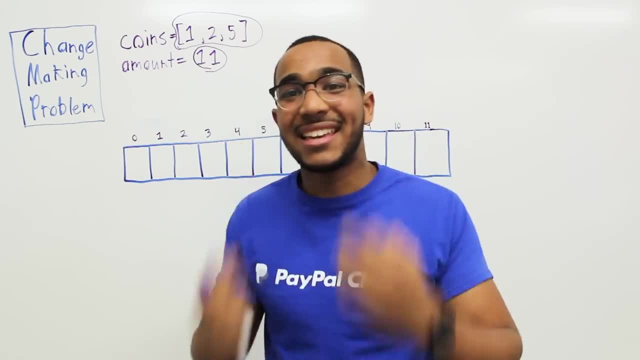 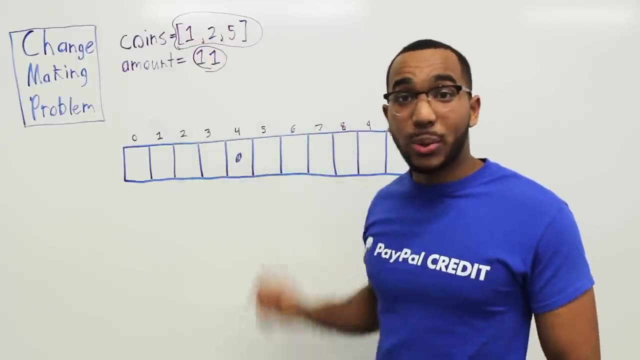 question that we will know previous answers to. That is the key to this. So, when I'm at here, my question is: if I have the amount four and I have the coins one, two and five, what is the minimum amount of coins that I have? What is the minimum amount of coins that I have? What is the 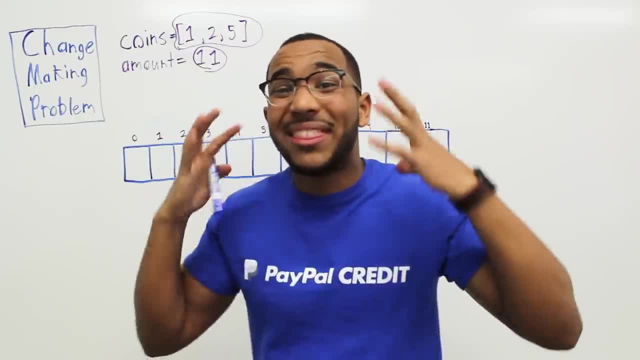 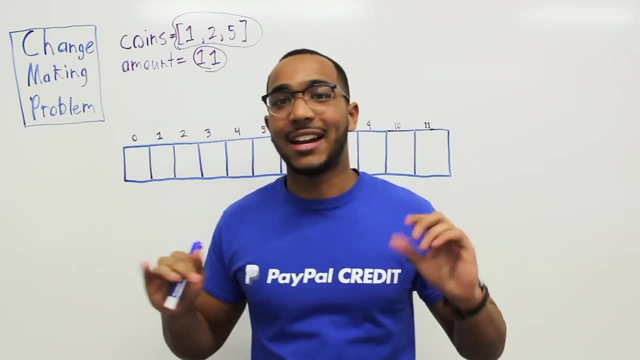 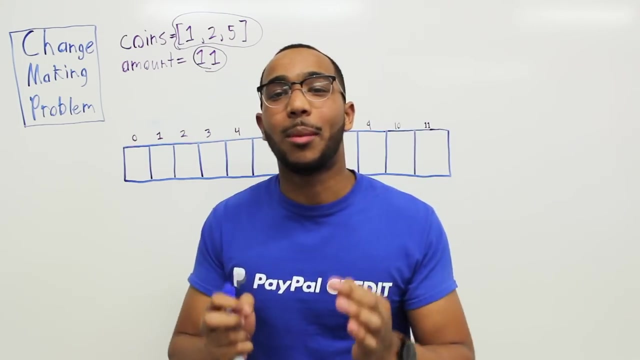 changing our psychology. We are not changing how we think about this problem. We are changing the way we approach this problem. If there is one thing I ask of you doing these Dynamic Programming questions: do not memorize the table, Do not memorize the ways these relate. Know the sub problems. Think about what is. 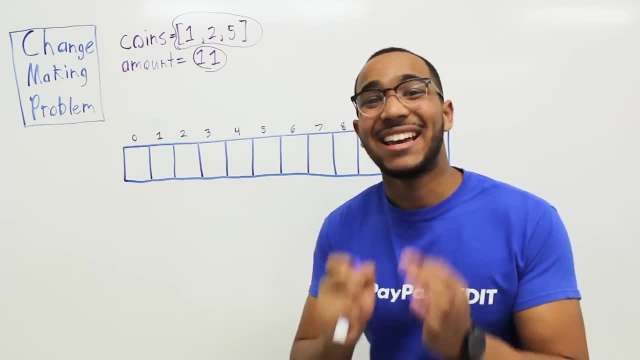 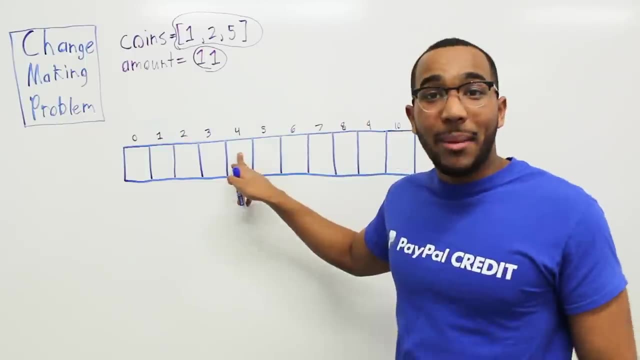 going on. Understand. each of these cells is asking a question. It is asking us a question that we will know previous answers to. That is the key to this. So what I'm at here, my question is if I have the amount four and I have the coins one, two and five. what is the minimum amount of coins I need to make change? When I am there, I am asking myself if I have the amount 7 and I have the coins 1,, 2, and 5, what is the minimum amount of coins I need to make change? 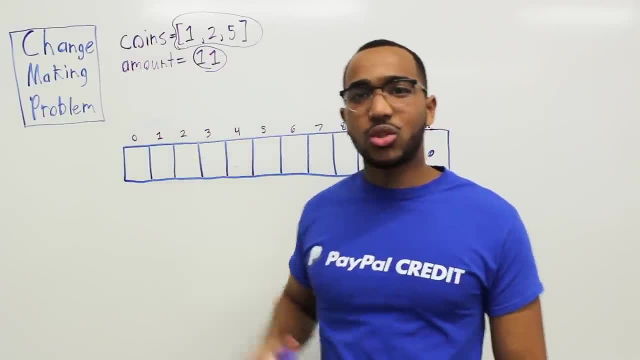 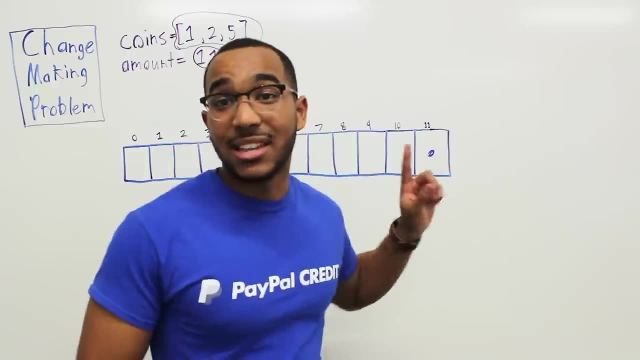 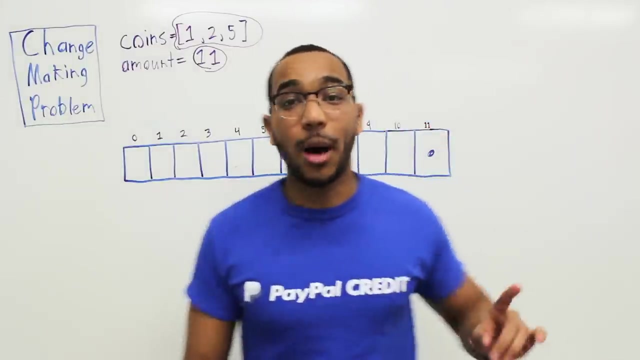 When I am here. wait, this is our original question. This is what we wanted to know all along. So that is the key. The key to the bottom-up tables we use is: we want this, We want this answer, But we need the answer to all of these previous questions so we can build a globally optimal answer which sits right there. 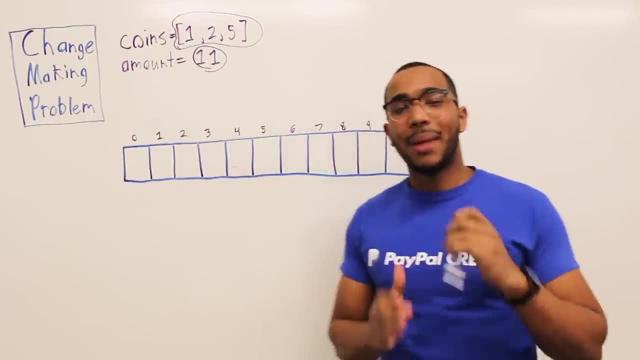 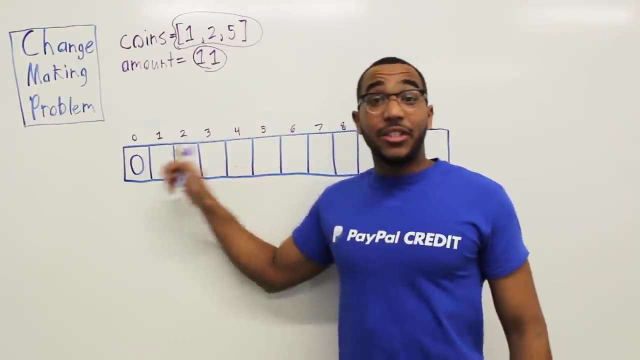 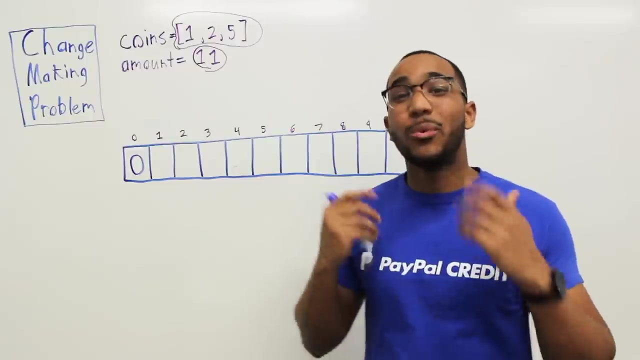 So what we will do is we fill the first cell the minimum amount of coins we need to use to make change for 0. No matter what coins we get, the answer is 0.. And then the rest of these cells, we fill them with an arbitrarily large value or some placeholder value, so that we know it's an empty state. 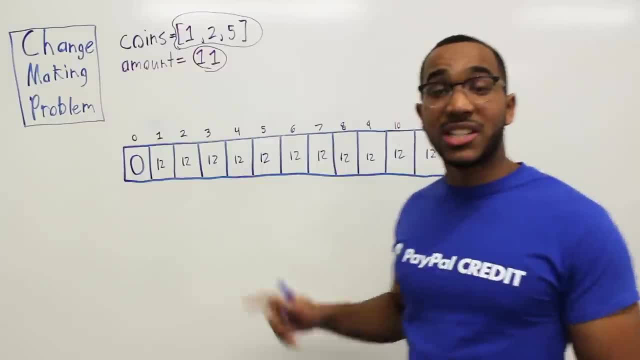 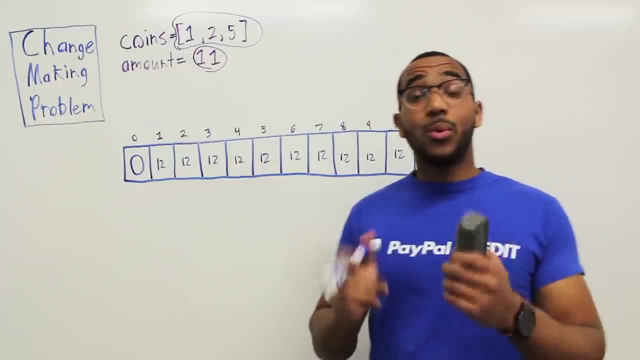 We can just fill it with amount plus 1.. All right, so, as you can see, we filled each cell with the value 12.. This is just an arbitrary placeholder as we solve these subproblems. So what we will do, we will solve every subproblem, from 1 to 11.. 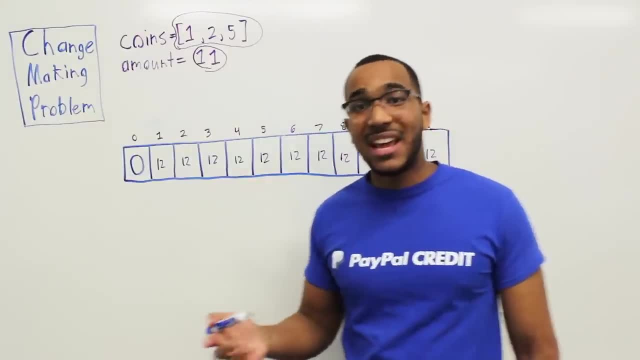 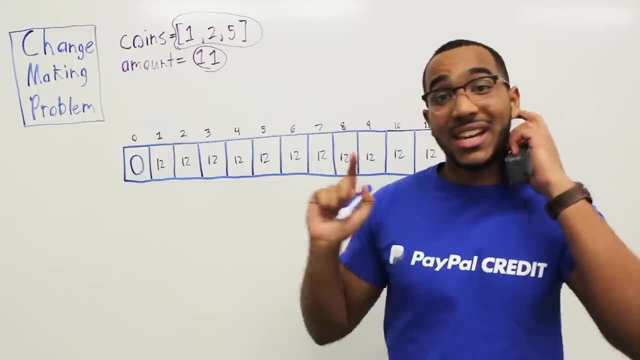 We're going to solve every subproblem from 1 to n- the amount. Our answer is going to be right here. The subproblem we want is this, But we're going to answer every subproblem leading up to it. If I have the amount 1, what is the minimum way I can make change? 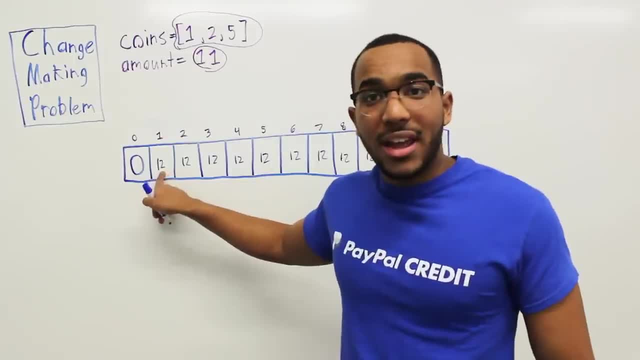 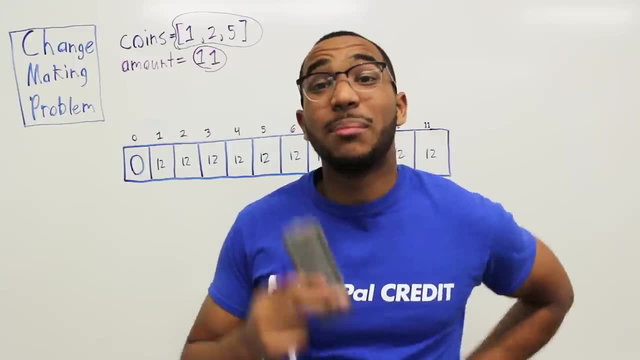 I'm going to try every coin. I'm going to try every coin against 1, and I'm going to add 1 to the value in the cell over here because, remember, each of these boxes are the minimum answer to the question. So we just add 1 to that because we're using a coin. 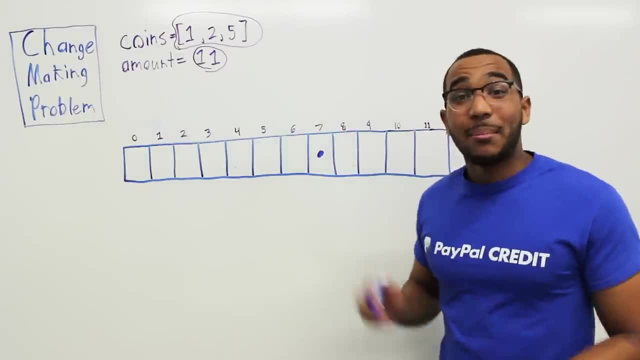 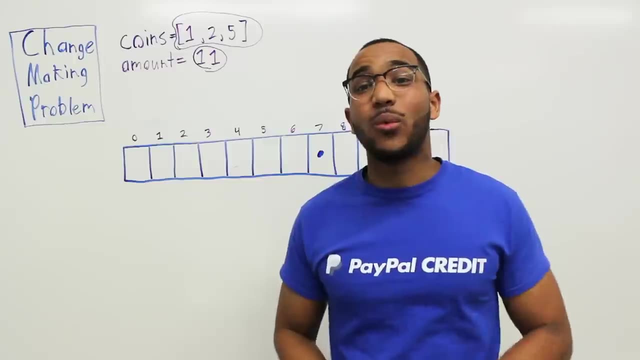 minimum amount of coins that I have. What is the minimum amount of coins that I have? What is the minimum amount of coins that I need to make change? When I am there, I am asking myself if I have the amount seven and I have the coins one, two and five. what is the minimum amount of coins? 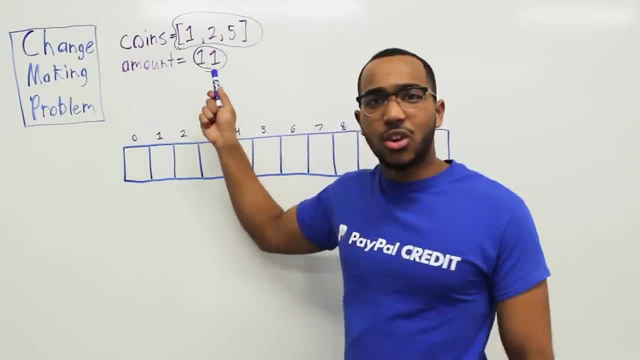 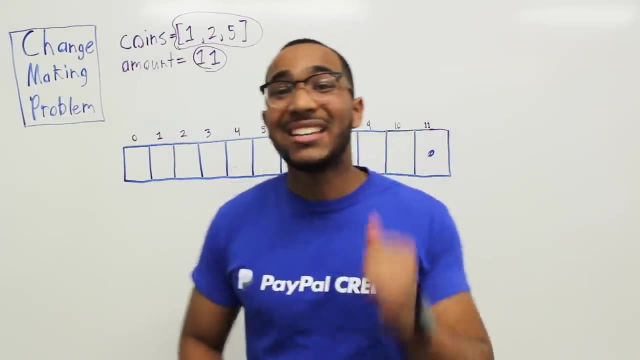 I need to make change When I am here. wait, this is our original question. This is what we wanted to know all along. So that is the key. The key to the bottom up tables we use is: we want this, We want this answer, but we need the answer to all of these previous questions. So 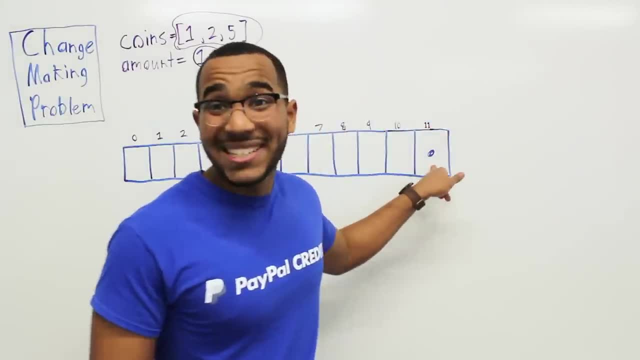 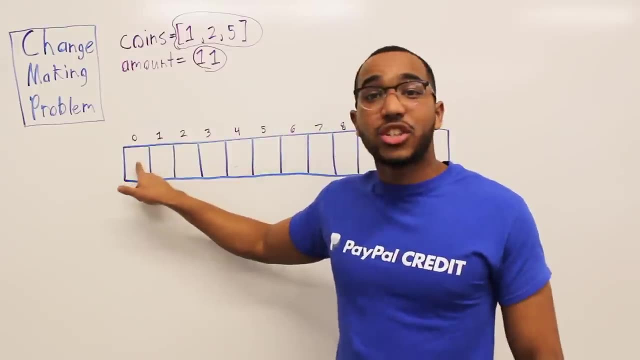 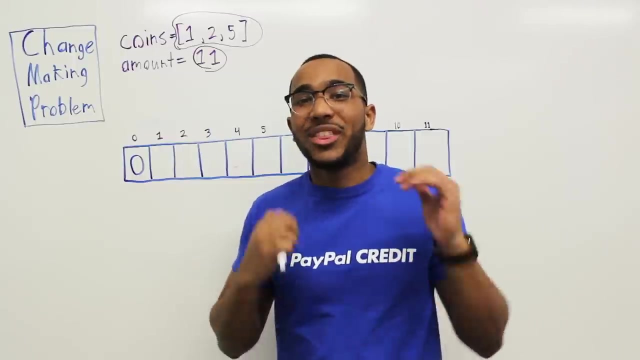 we can build a globally optimal answer which sits right there. So what we will do is we fill the first cell- the minimum amount of coins we need to use to make change- for zero. No matter what coins we get, the answer is zero. And then the rest of these cells, we fill them with an. 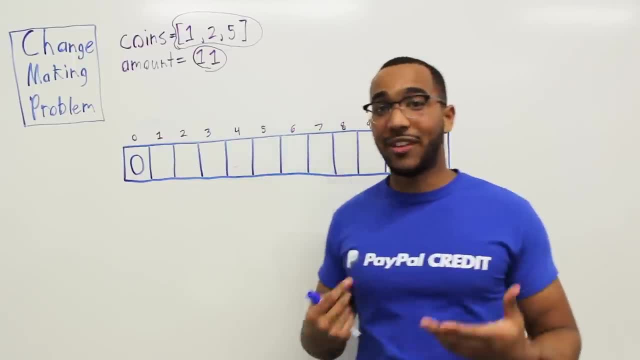 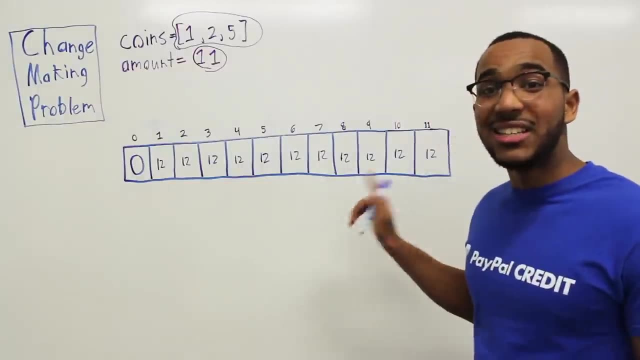 arbitrarily large value or some placeholder value, so that we know it's an empty state. We can just fill it with amount plus one, All right. So, as you can see, we filled each cell with the value 12.. This is just an arbitrary placeholder as we solve these subproblems. So what we will do, 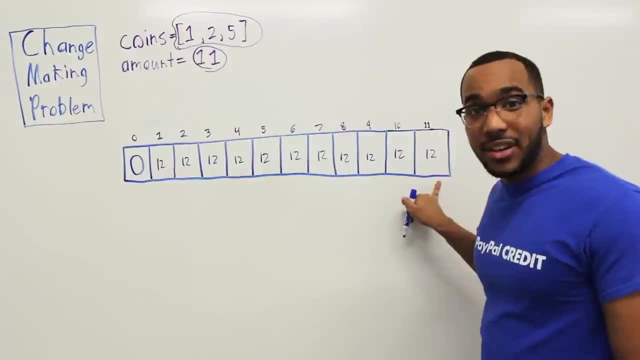 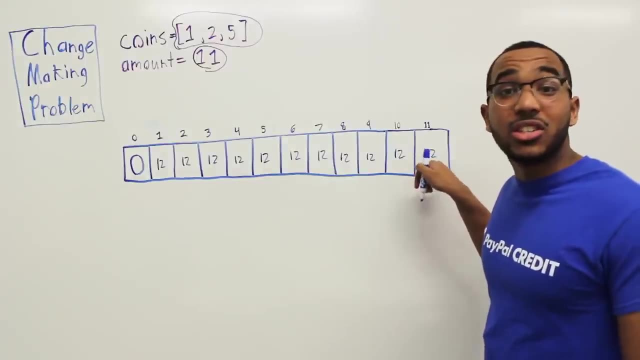 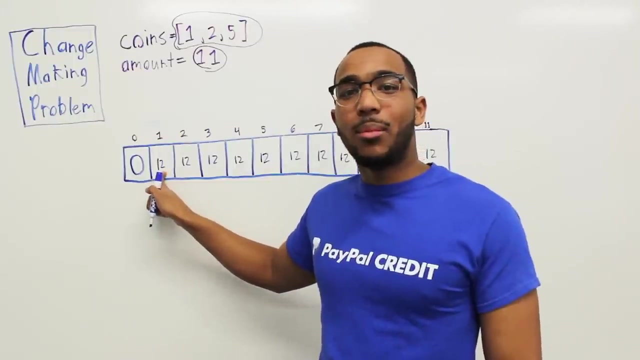 we will solve every subproblem from one to 11.. We're going to solve every subproblem from one to n. the amount. Our answer is going to be right here. The subproblem we want is this, but we're going to answer every subproblem leading up to it. If I have the amount one, what is the minimum? 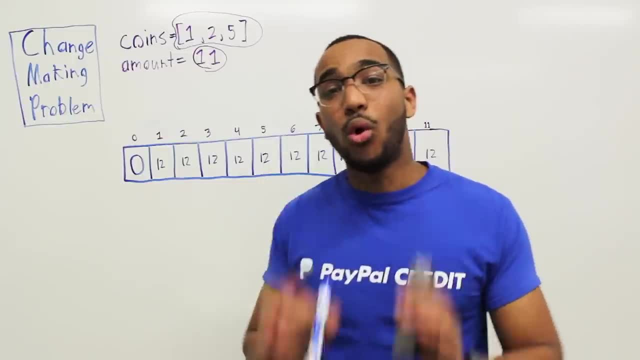 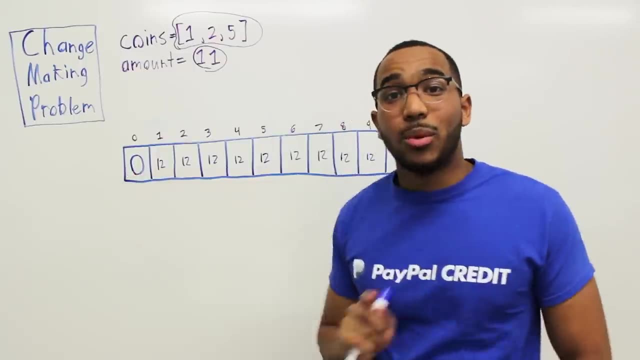 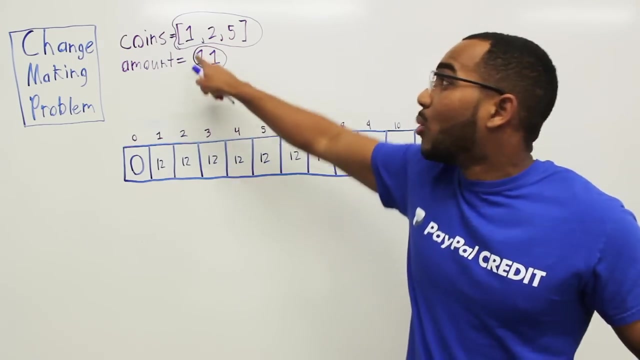 way I can make change. I'm going to try every coin against one and I'm going to add one to the value in the cell over here because, remember, each of these boxes are the minimum answer to the question. So we just add one to that. because we're using a coin, We're acting like one, two. 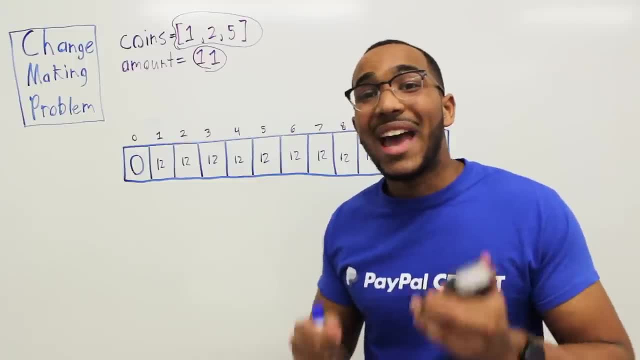 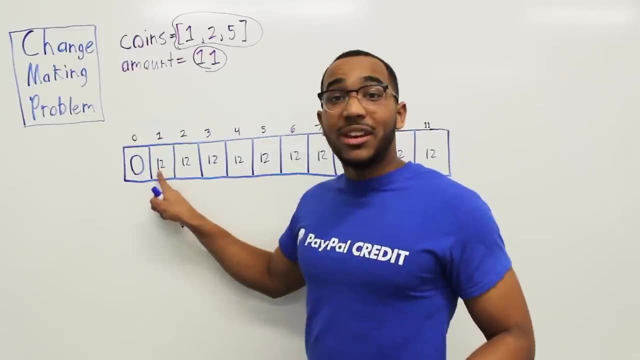 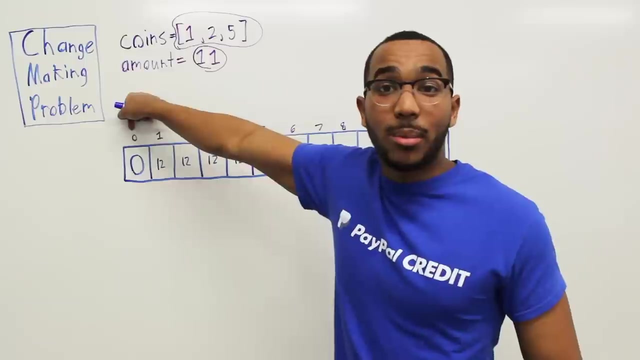 and five. One, two or five are our last coin. We add one to the answer we find subtracted away from that coin. So you'll understand as we walk through this. So what we do here is we have the amount one. The only coin we can use is one. One minus one is zero. So we look at the subproblem. 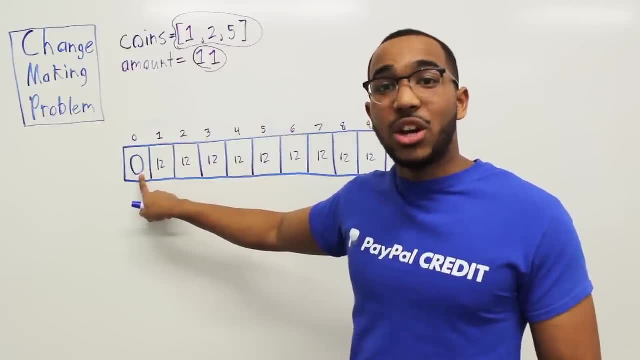 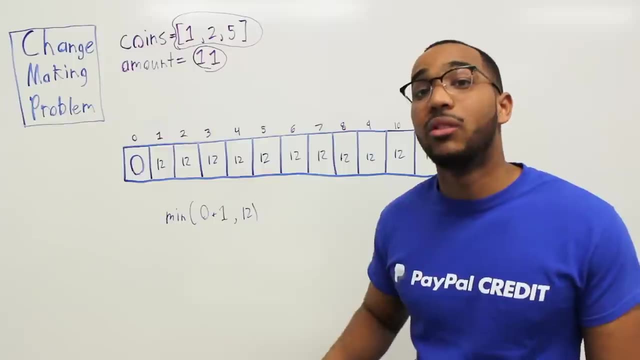 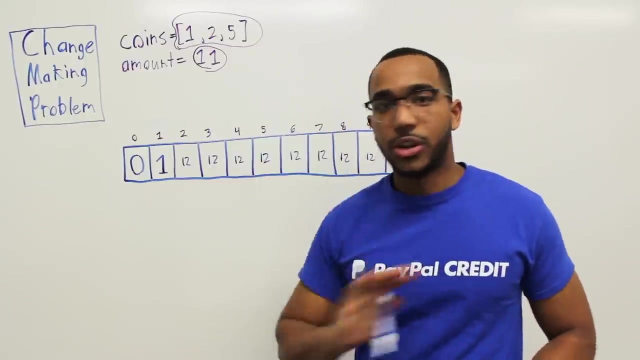 the minimum way to make change is zero. So what we do is we do zero plus one, We do min zero plus one versus twelve. One is less than twelve. One is our new best answer. So one is our new best answer there. Can we use the coin two? No, we can't. 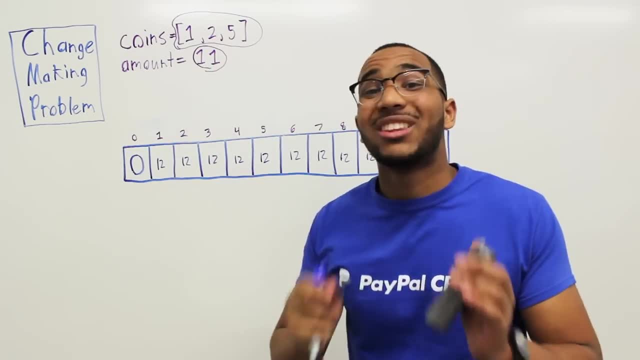 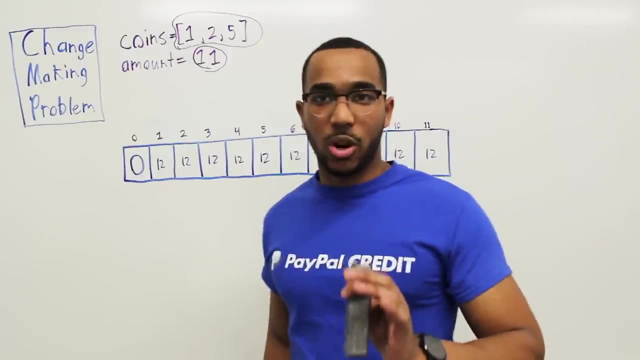 We're acting like 1,, 2, and 5,. 1,, 2, or 5 are our last coin. We add 1 to the answer we find subtracted away from that coin. So you'll understand as we walk through this. 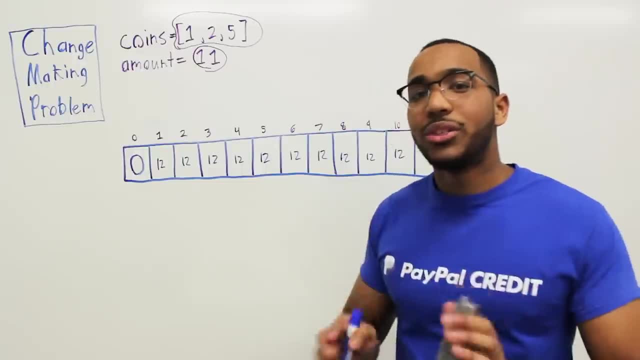 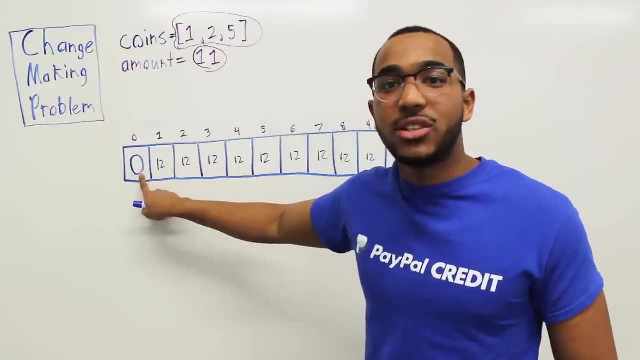 So what we do here is we have the amount 1.. The only coin we can use is 1.. 1 minus 1 is 0. So we look at the subproblem 0. The minimum way to make change is 0.. 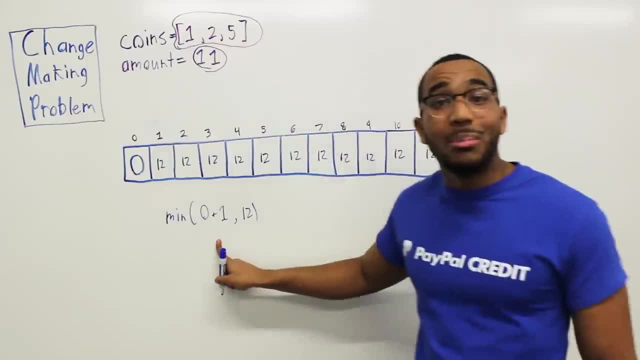 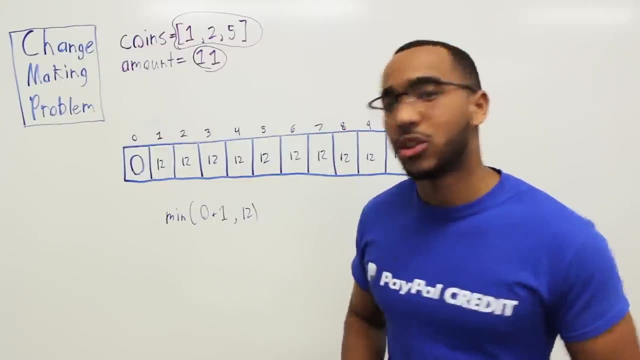 So what we do is we do 0 plus 1.. We do min 0 plus 1 versus 12.. 1 is less than 12.. 1 is our new best answer, So 1 is our new best answer there. 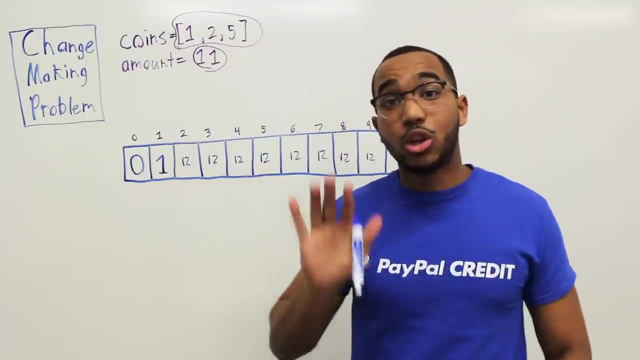 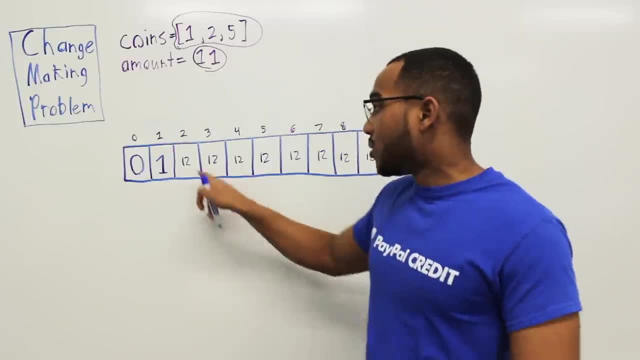 Can we use the coin 2? No, we can't. Can we use the coin 5? No, we can't. So this is our answer. The subproblem for the amount 1, the answer is 1.. So now we move on. 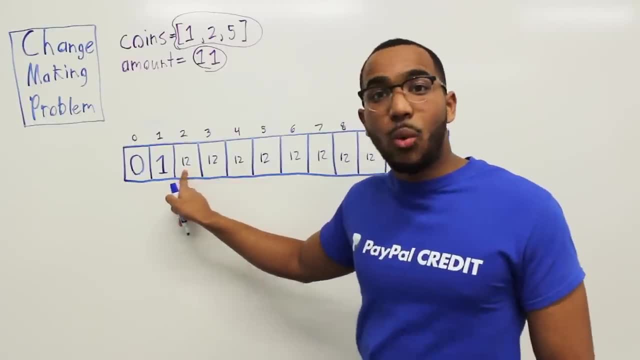 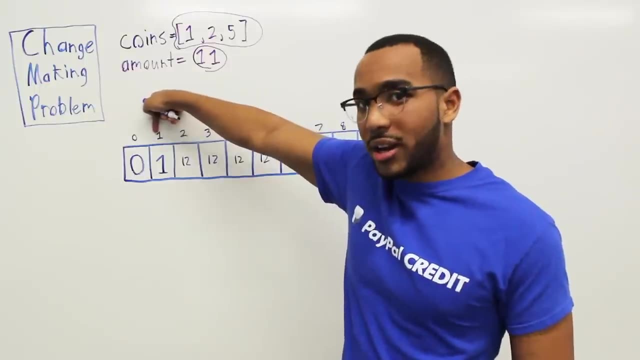 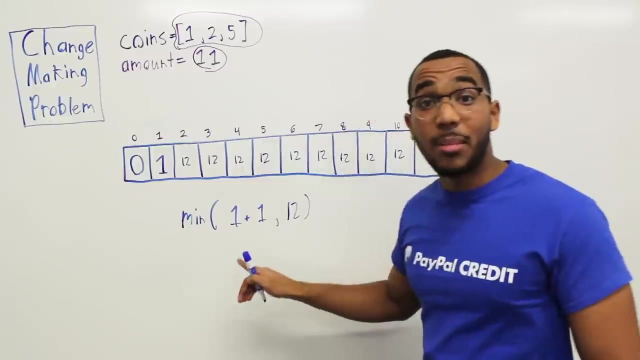 The subproblem for the amount 2.. Can I use the coin 1?? Yes, I can. 2 minus 1 is 1.. Now we say this subproblem: if I use 1, that's using a coin. So I say the answer to this subproblem: plus 1,, 1 plus 1, the minimum of 1 plus 1 and 12.. 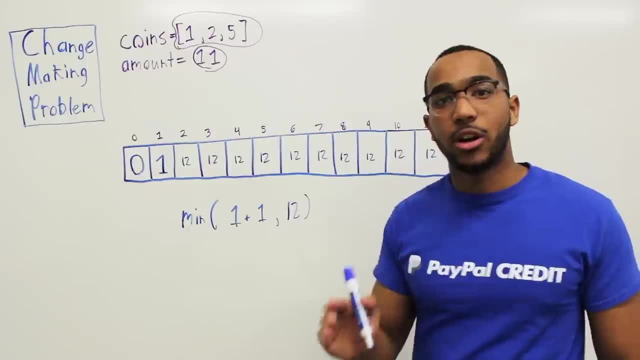 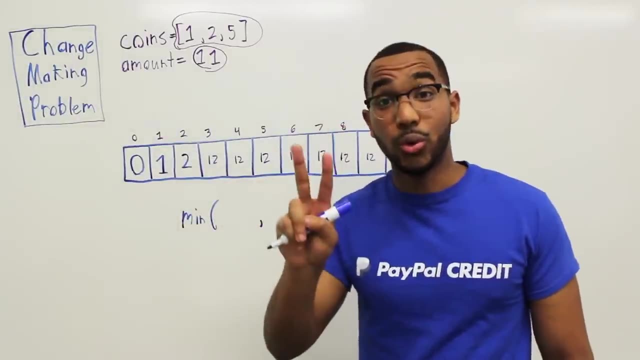 Who wins 2.. 2 is the winner, So that becomes our new best answer. Okay, we tried the 1.. Now we have to try the rest of our coins. If we try 2,, 2 minus 2 is 0.. 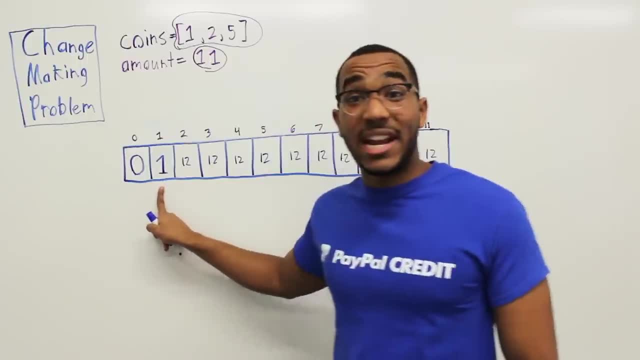 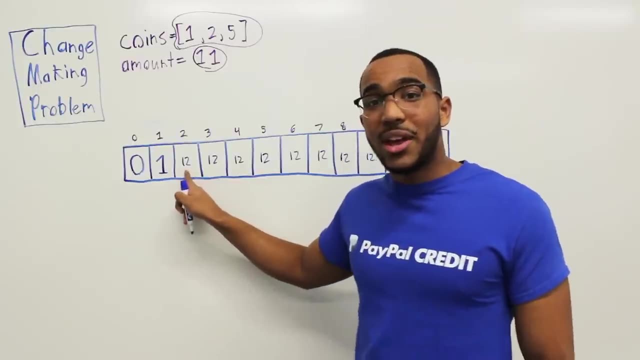 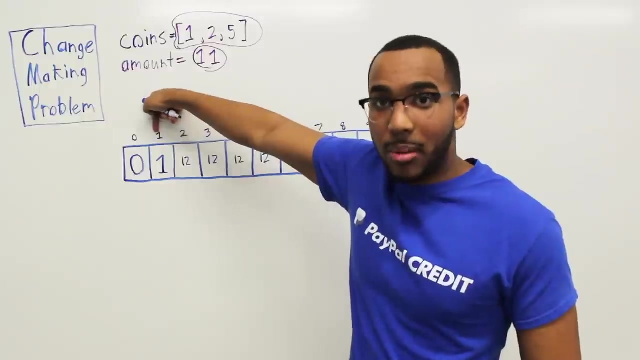 Can we use the coin five? No, we can't. So this is our answer. The subproblem for the amount one: the answer is one. So now we move on. the subproblem for the amount two: can I use 1.. Yes, I can. 2 minus 1 is 1.. Now we say this sub problem: if I use 1, that's using a coin. So I say: 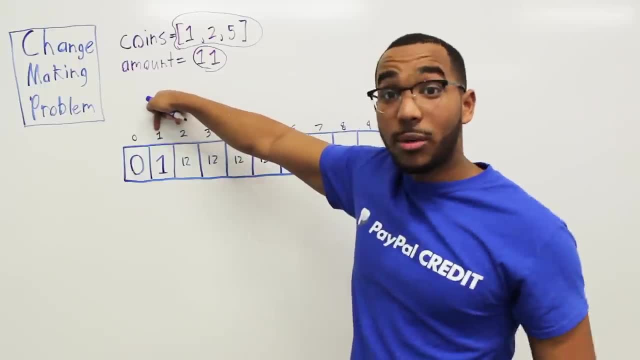 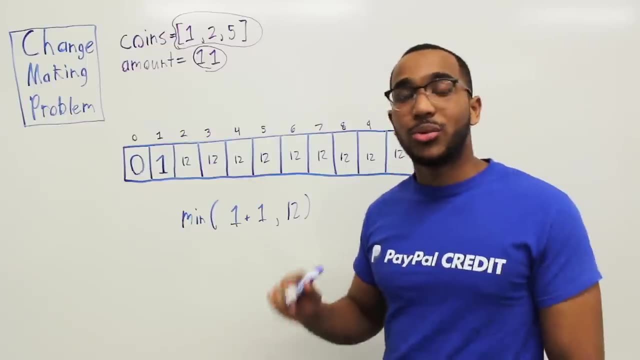 the answer to this sub problem: plus 1,, 1 plus 1, the minimum of 1 plus 1 and 12.. Who wins 2. 2 is the winner, So that becomes our new best answer. Okay, we tried the 1.. Now we have to try the rest. 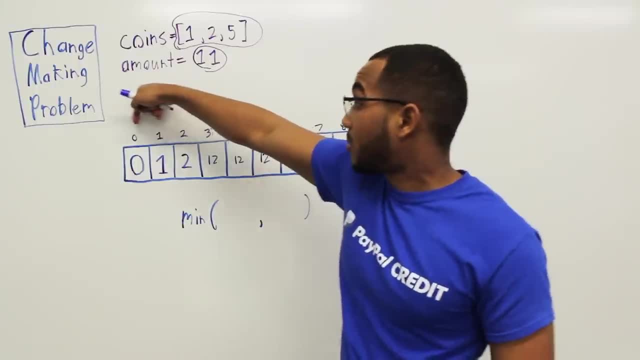 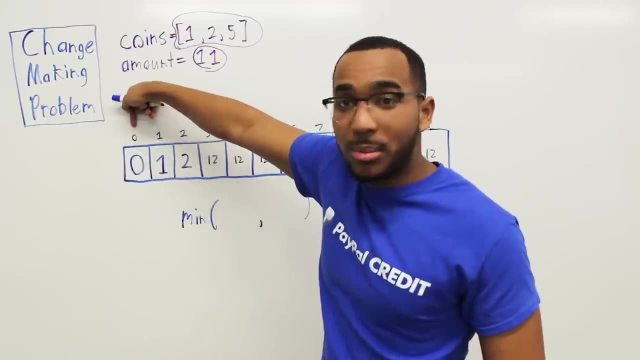 of our coins. If we try 2,, 2 minus 2 is 0.. If I use 2 as my last coin, I do the answer to the sub problem minus my coin, which is the sub problem 0.. The best answer is 0.. 0 plus 1? 0 plus 1 versus. 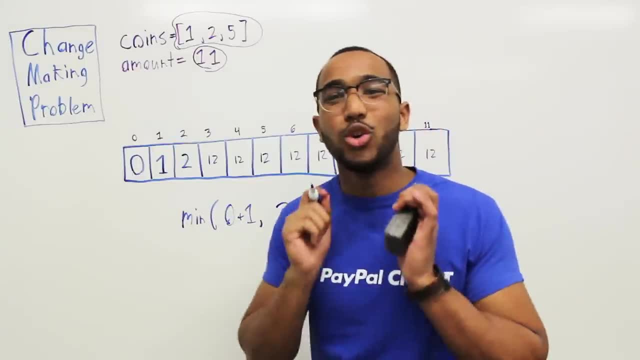 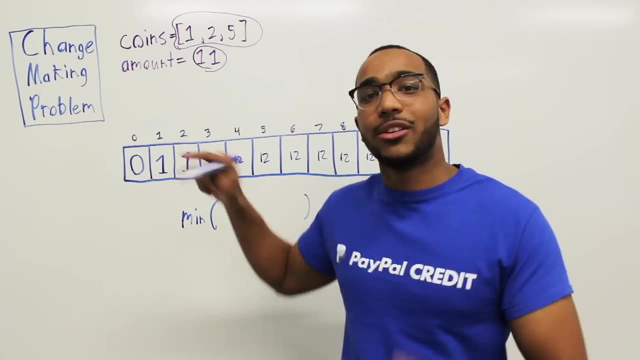 our best answer so far: 1 wins. 1 is our new best answer. So now we try the 5.. Can we try 5?? We cannot. 5 is greater than 2.. We cannot subtract 5 without going negative. 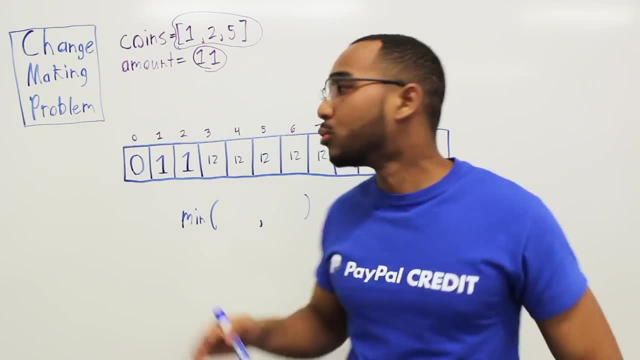 So 1 is greater than 2.. We cannot subtract 5 without going negative, So 1 is greater than 2.. So what is the answer to our sub-problem for the amount 2? The minimum amount of coins, given our coins, to make change for 2 is 1.. 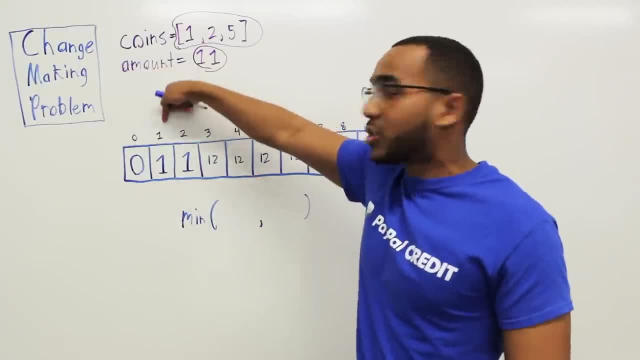 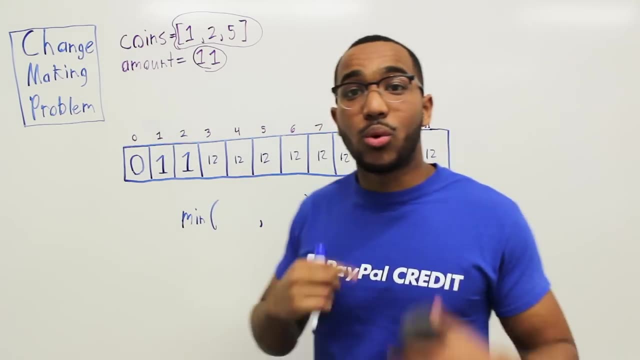 We use the 2 coin. So we have solved sub-problem, sub-problem, sub-problem, And now we're going to continue like this and solve all of these sub-problems And by the time we get here we are going to finish the problem. 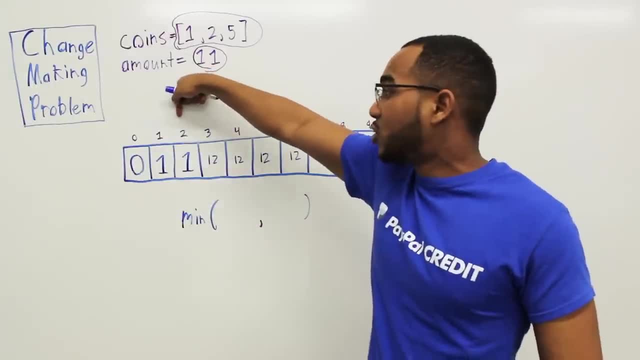 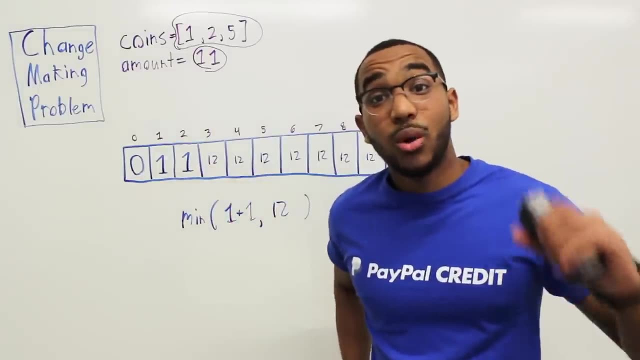 So now let's try coin 1.. 3 minus 1 is 2.. We have 1,, so this is what we do: 1,, which is the best answer, at 2, plus 1,, because we just used the 1 coin. 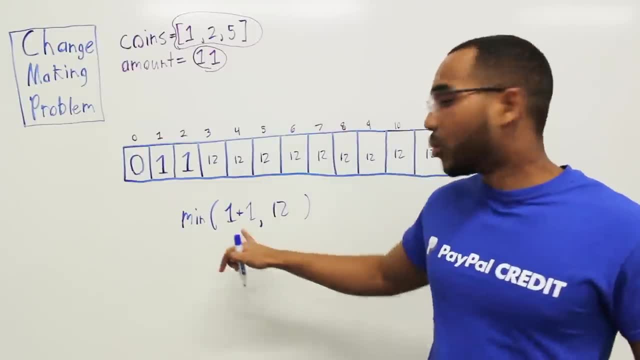 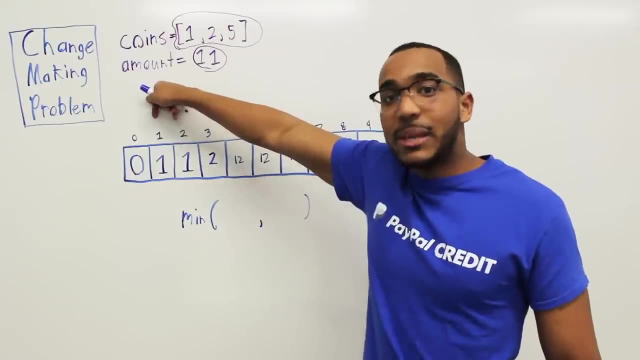 versus the best answer 12.. 2 wins. 1 plus 1 is 2.. So now we try the 1 coin, Let's try the 2 coin. So 3 minus 2 is 1.. The best answer at 1 is 1 coin. minimum coins to make change. 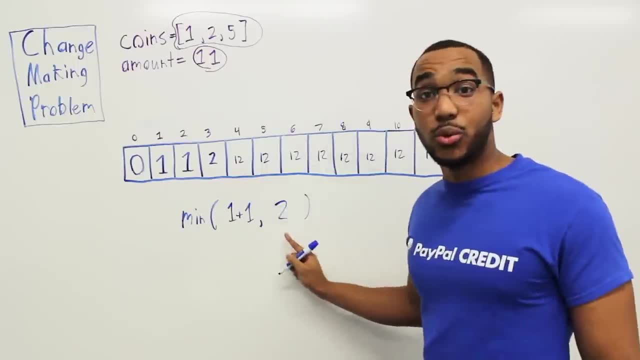 So we do 1 plus 1.. 1 plus 1 versus 2.. 1 plus 1 is 2.. 2 is not less than 2.. It's less than or equal to 2. It is actually equal to 2.. 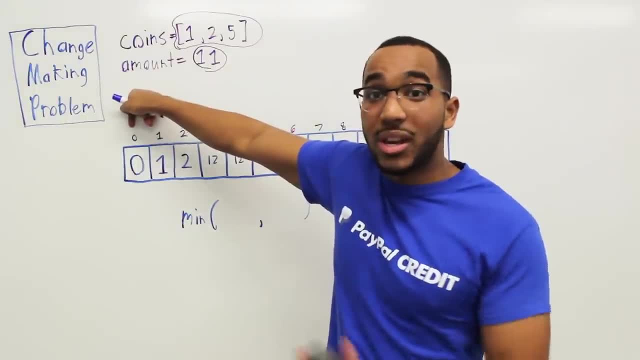 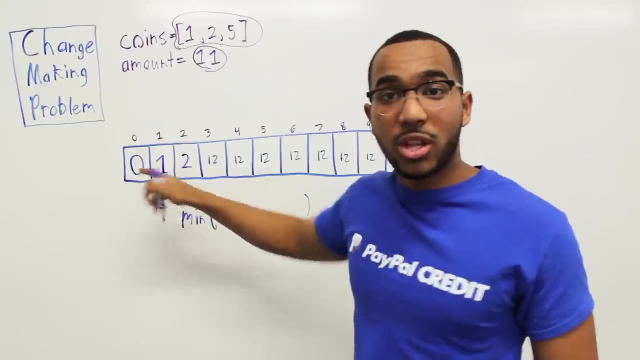 If I use 2 as my last coin, I do the answer to the subproblem minus my coin, which is the subproblem 0.. The best answer is 0.. 0 plus 1?. 0 plus 1 versus our best answer so far. 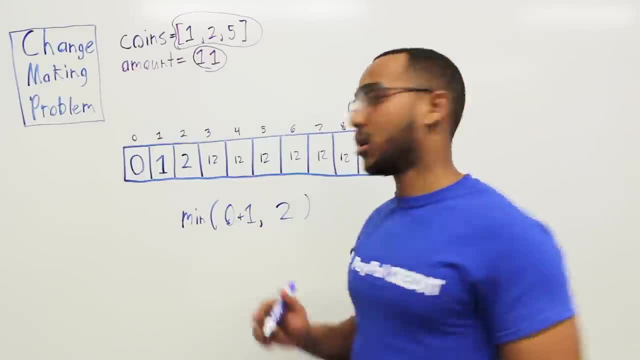 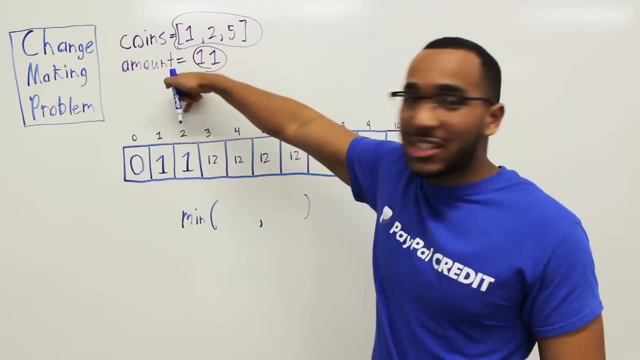 1 wins 1 is our new best answer. So now we try the 5.. Can we try 5?? We cannot. 5 is greater than 2.. We cannot subtract 5 without going negative. So what is the answer to our subproblem for the amount 2?? 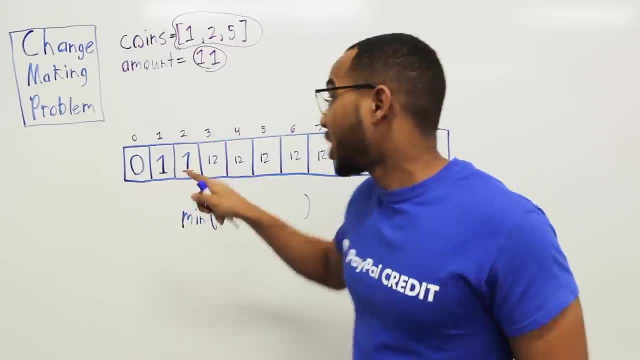 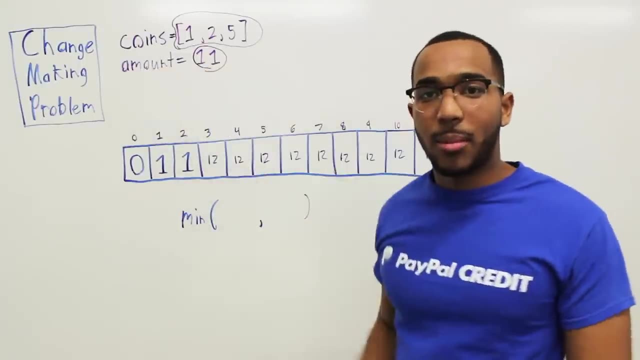 The minimum amount of coins, given our coins, to make change for 2 is 1.. We use the 2 coin. So we have solved subproblem, subproblem, subproblem, And now we're going to continue like this and solve all of these subproblems. 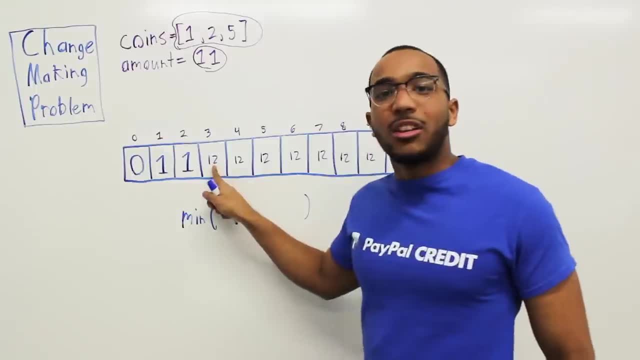 And by the time you get here, we are going to finish the problem. So now let's try coin 1.. 3 minus 1 is 2.. We have 1.. So this is what we do: 1, which is the best answer. 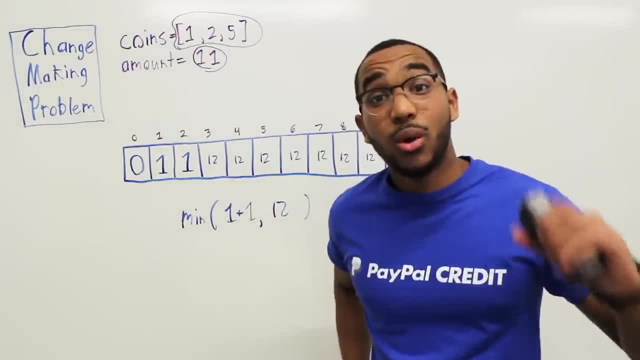 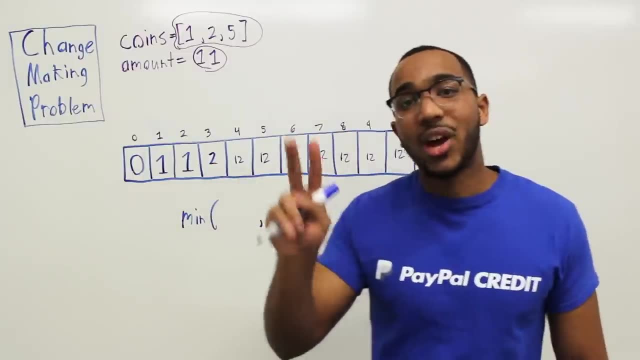 2 plus 1, because we just used the 1 coin versus the best answer 12.. 2 wins. 1 plus 1 is 2.. So now we try the 1 coin, Let's try the 2 coin. 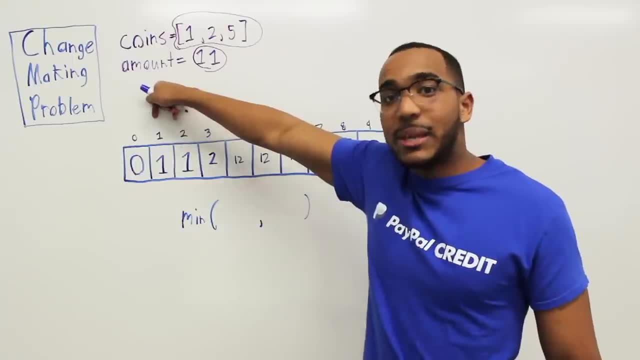 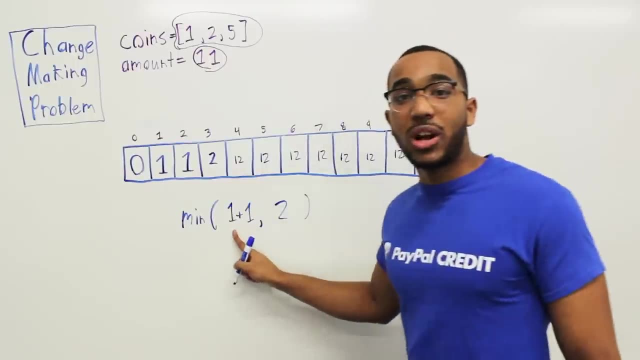 So 3 minus 2 is 1.. The best answer at 1 is 1 coin, minimum coins to make change. So we do 1 plus 1.. 1 plus 1 versus 2.. 1 plus 1 is 2.. 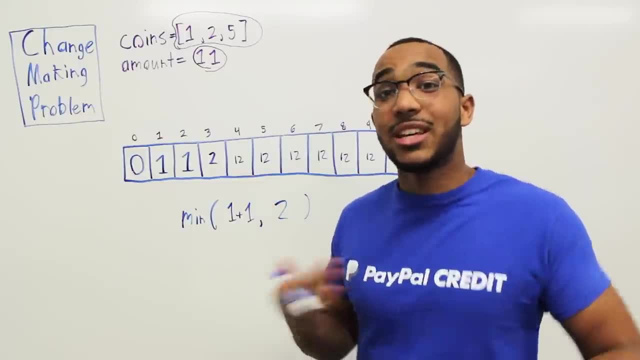 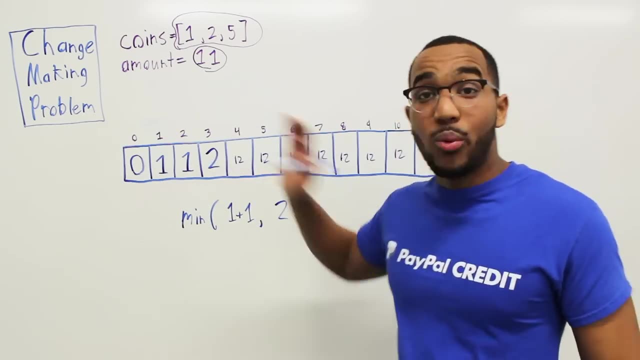 2 is not less than 2.. It's less than or equal to 2.. It is actually equal to 2.. But that won't change our answer. Our answer stays 2.. So can we use 5?? No, we can't. 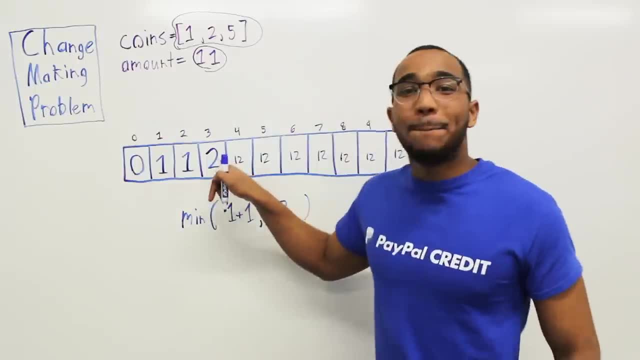 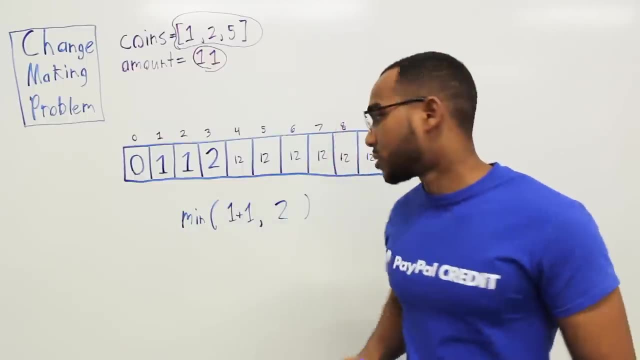 We've tried all our coins. We are finished. The best answer to our subproblem is using 2 coins To make change for the amount 3, we use 2 coins And so now we move on. We try the coin with a value of 1.. 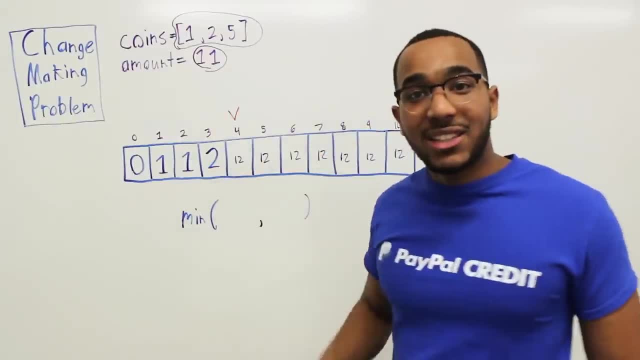 4 minus 1 is 3.. 3, our best answer was 2.. So 2 plus 1.. And again we're adding 1 because we're using a coin. The best answer at 3 was 2.. 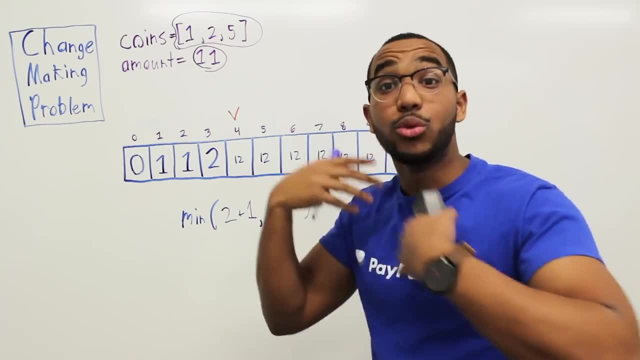 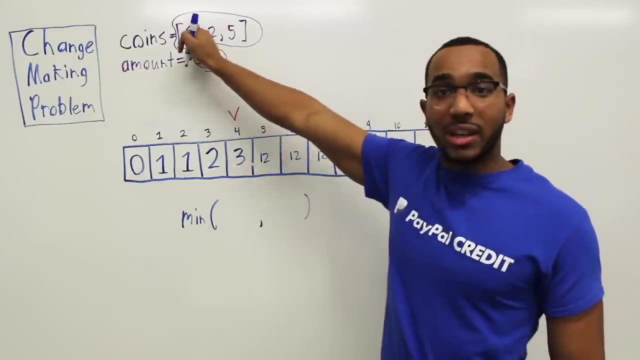 We add 1 to that because we're using a coin. So now 2 plus 1 versus 12.. 3 is the winner. It is less, And so now we've tried the 1.. Let's try the 2.. 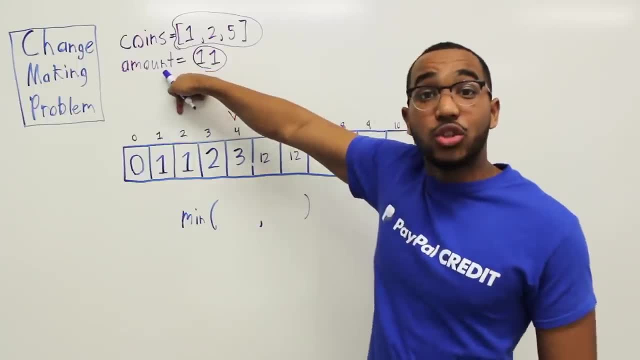 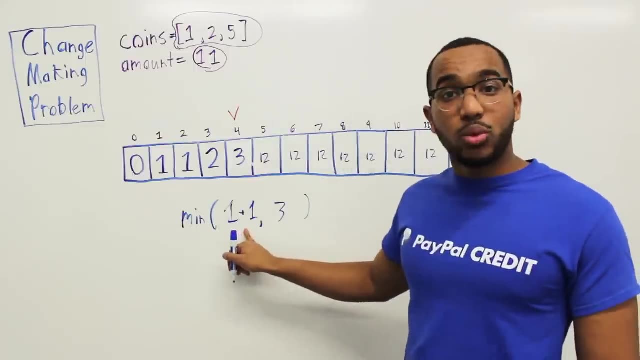 4 minus 2. It is 2.. The best answer at 2 is 1.. 1 plus 1 versus 3.. 1 plus 1 is 2.. 2 is less than 3.. 2 is the winner. 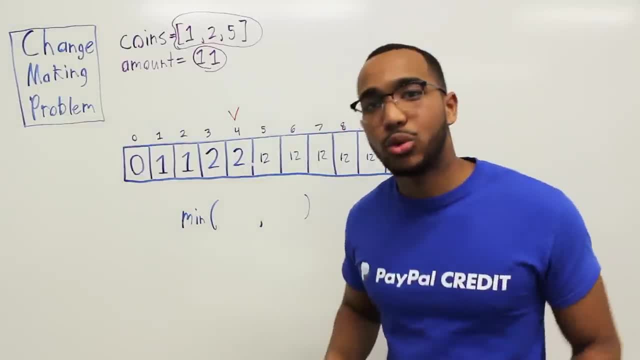 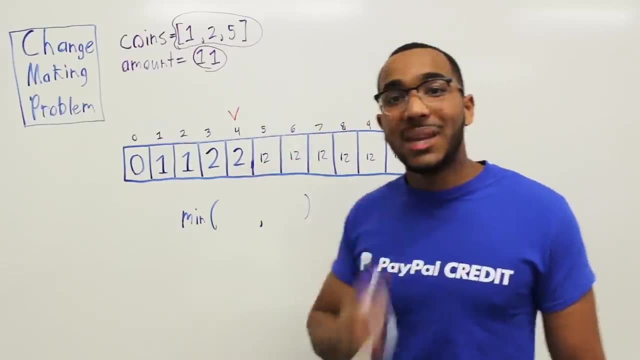 Can we use coin 5?? We cannot use coin 5.. 5 is greater than 4.. So the winner, The winner to our sub-problem, is 2.. The minimum amount of coins to make change for the amount 4, given these coins, is 2.. 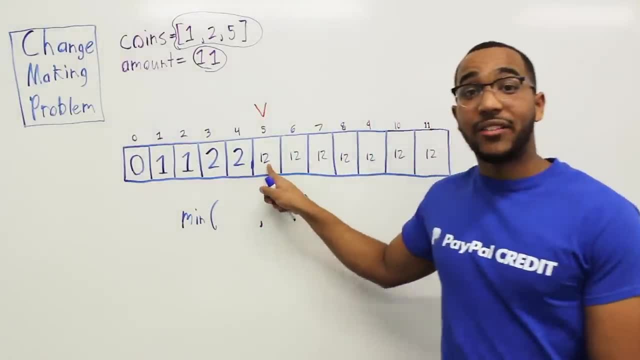 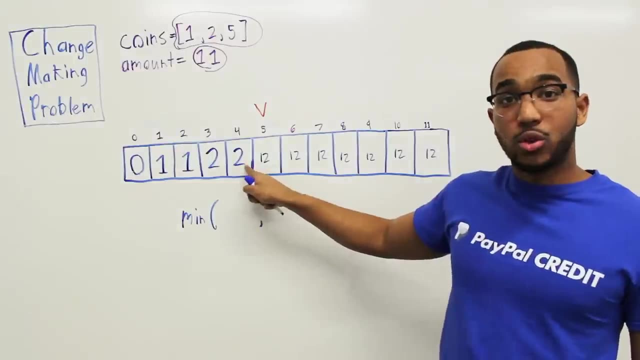 We use a 2 and a 2.. That is our answer. And so now 5.. If we use 1 as our last coin, our best answer is going to be right there. We do 2 plus 1.. 2 plus 1 versus 12.. 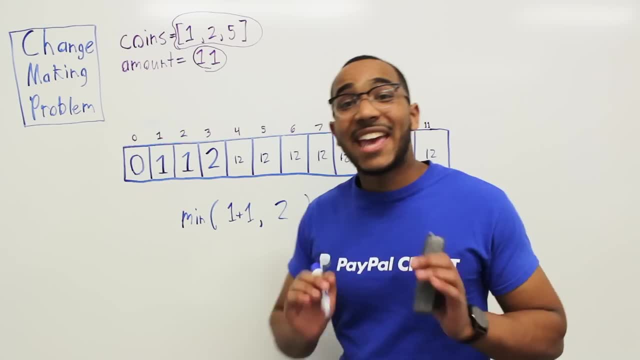 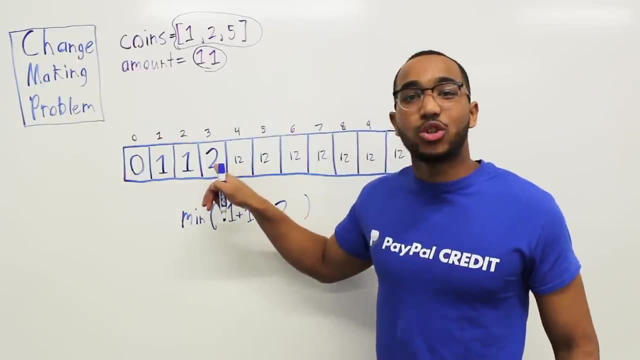 That won't change our answer. Our answer stays 2.. So can we use 5?? No, we can't. We've tried all our coins. We are finished. The best answer to our sub-problem is using 2 coins. 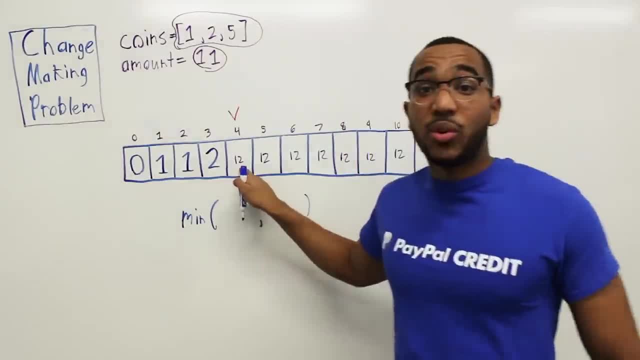 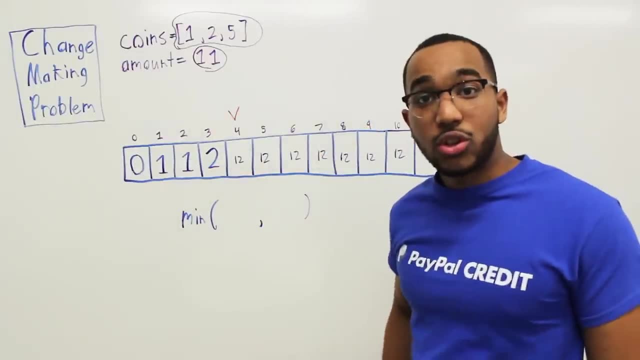 To make change for the amount. 3, we use 2 coins, And so now we move on. We try the coin with a value of 1.. 4 minus 1 is 3. 3,. our best answer was 2.. 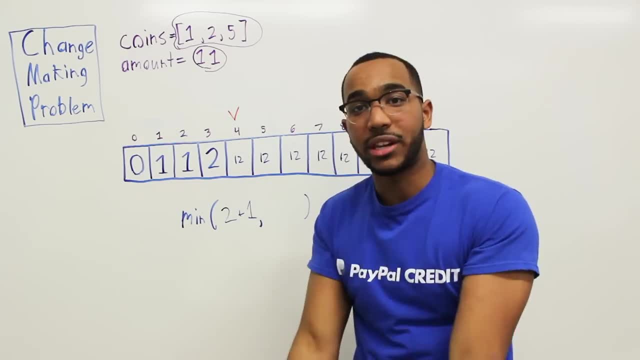 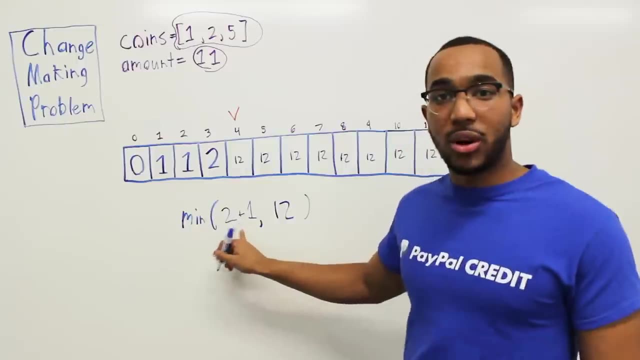 So 2 plus 1.. And again we're adding 1 because we're using a coin. The best answer at 3 was 2.. We add 1 to that because we're using a coin. So now 2 plus 1 versus 12.. 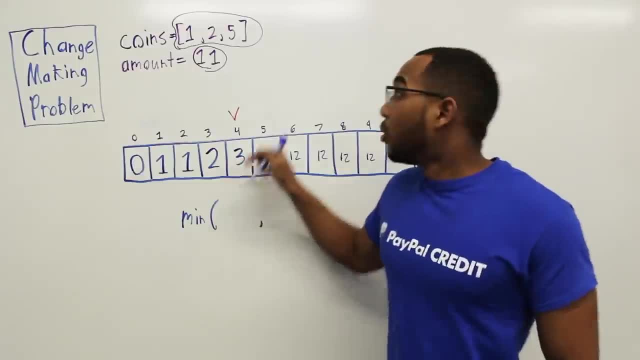 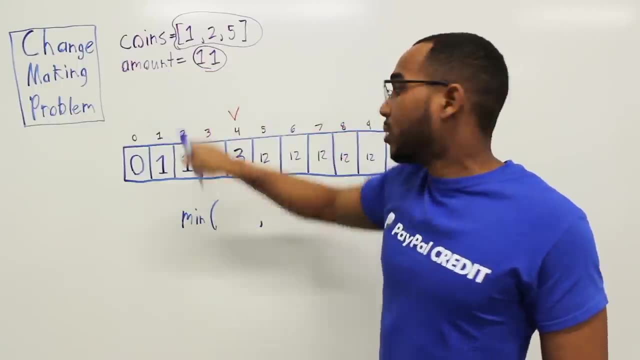 3 is the winner, It is less, And so now we've tried the 1.. Let's try the 2.. 4 minus 2. It is 2.. The best answer at 2 is 1.. 1 plus 1 versus 3.. 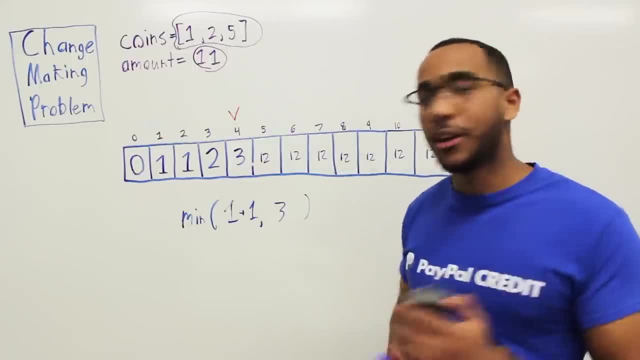 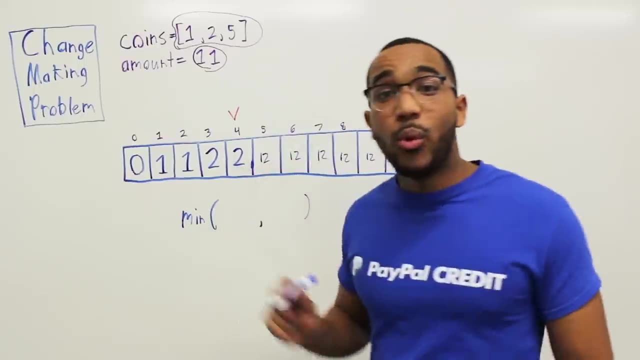 1 plus 1 is 2.. 2 is less than 3.. 2 is the winner. Can we use coin 5?? We cannot use coin 5.. 5 is greater than 4.. So the winner, the winner to our sub-problem, is 2.. 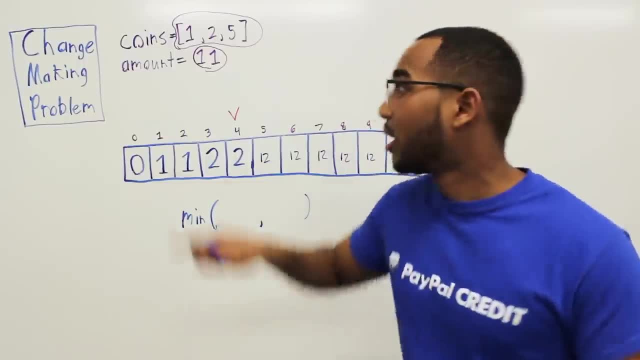 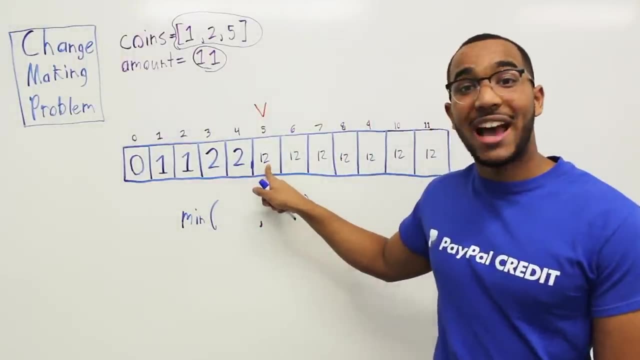 The minimum amount of coins to make change for the amount 4, given these coins, is 2.. We use a, 2 and a 2.. That is our answer, And so now 5. If we use 1 as our last coin, our best answer is going to be right there. 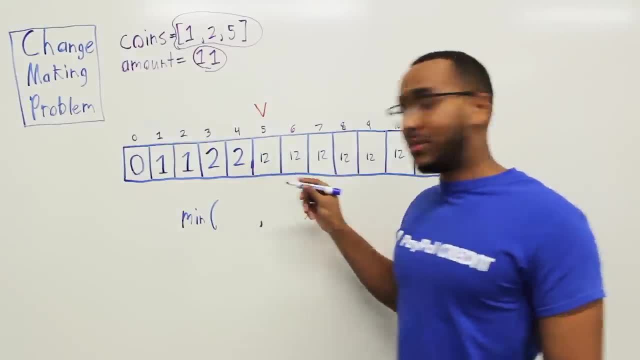 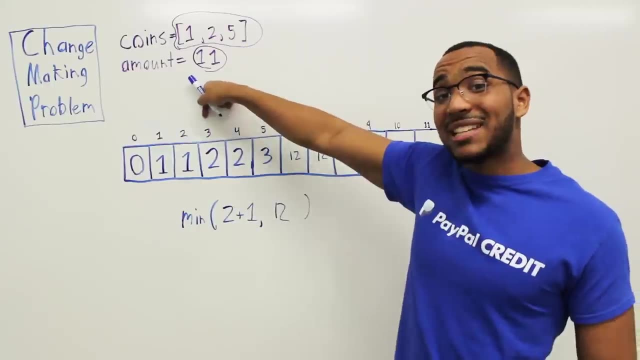 We do 2 plus 1.. 2 plus 1 versus 12.. 3 versus 12. 3 is the winner? Now, if I use 2 as the last coin, 5 minus 2.. The best answer at 3 is 2.. 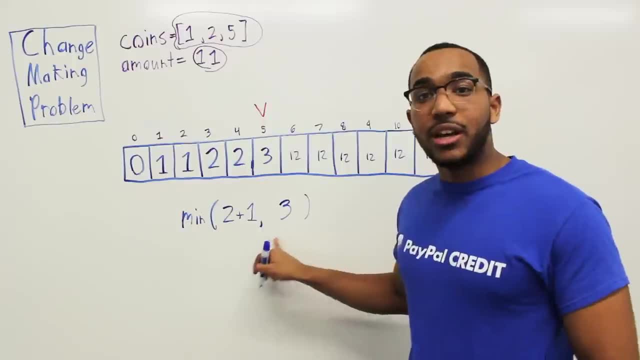 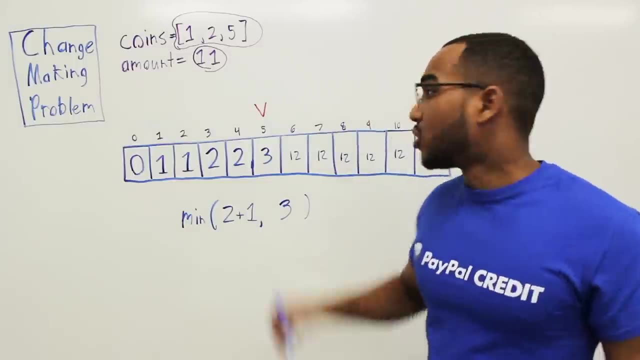 So 2 plus 1.. And then we have that against 3.. 2 plus 1 versus 3 is 3 versus 3. So nothing changes. So now we can use the 5. So 5 minus 5 is 0.. 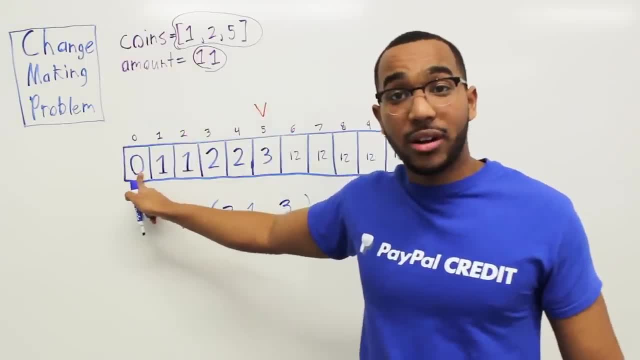 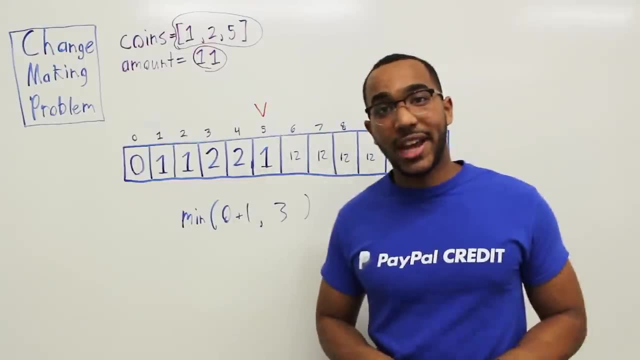 The best answer at 0 is 0.. 0 plus 1 versus 0 plus 1 versus 3.. 1 is the winner. The best way to make change at 5, given these coins is just to use the 5 coin. 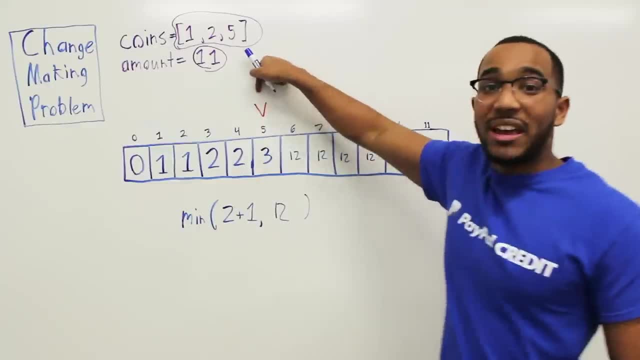 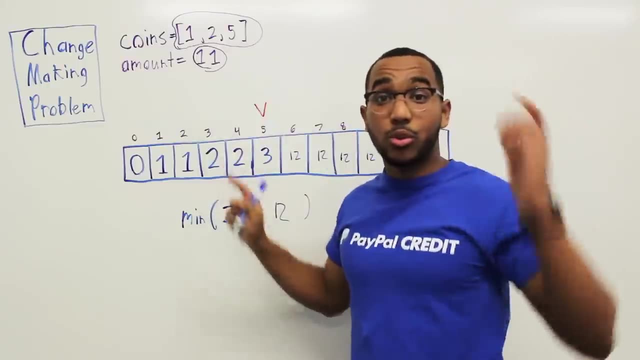 3 versus 12.. 3 is the winner. Now, if I use 2 as the last coin: 5 minus 2.. 5 minus 2.. The best answer at 3 is 2.. So 2 plus 1.. 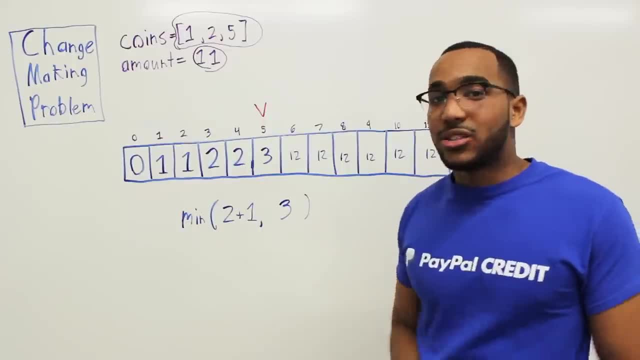 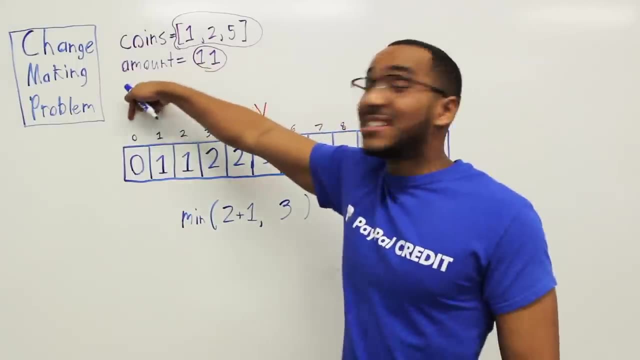 And then we have that against 3.. 2 plus 1 versus 3 is 3 versus 3.. So nothing changes. So now we can use the 5.. So 5 minus 5 is 0.. The best answer at 0 is 0.. 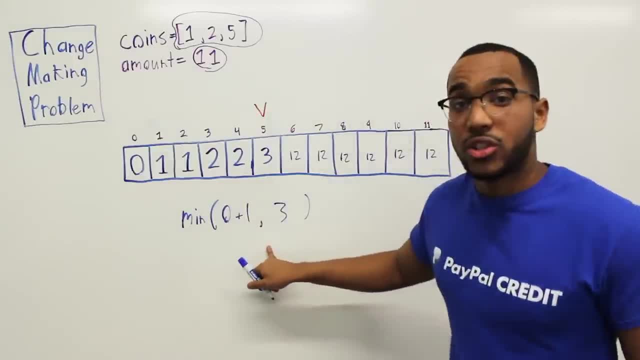 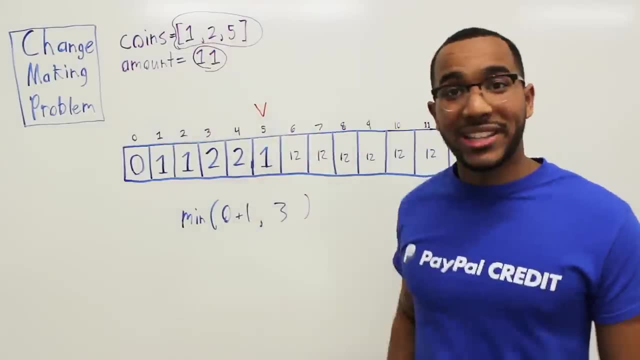 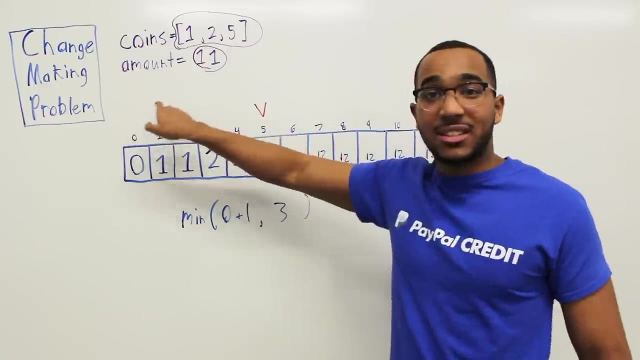 0 plus 1 versus 0 plus 1 versus 3.. 1 is the winner. The best way to make change at 5. given these coins is just to use the five coin. It is one. That is the answer to our sub problem. We have solved this, this, this, this and this We have solved. 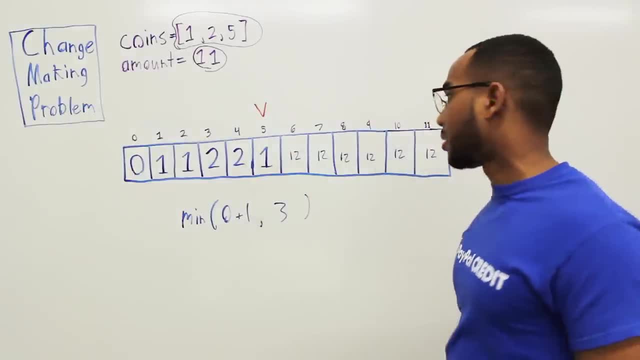 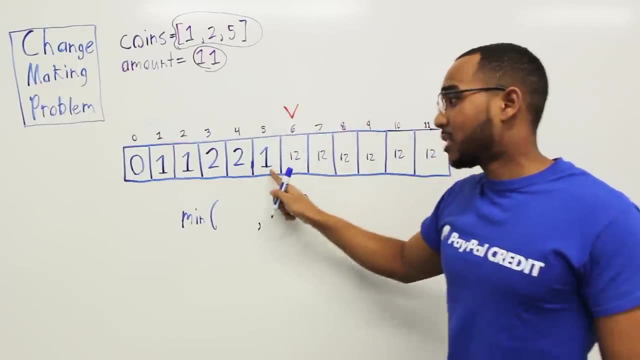 six sub problems and now we're going to continue on. So now I am at sub problem six. So if I try the one coin, six minus one is five. The best answer at five is one, One plus one. One plus one versus twelve. Two is the winner, And I want to. 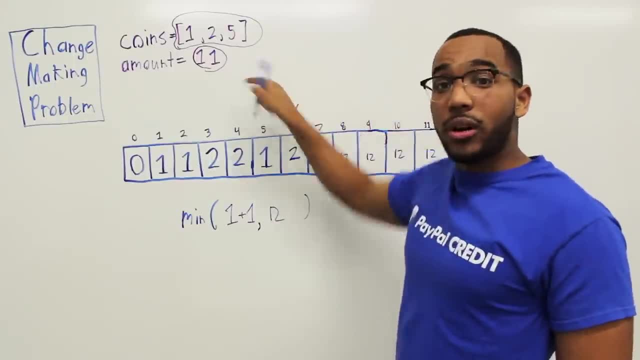 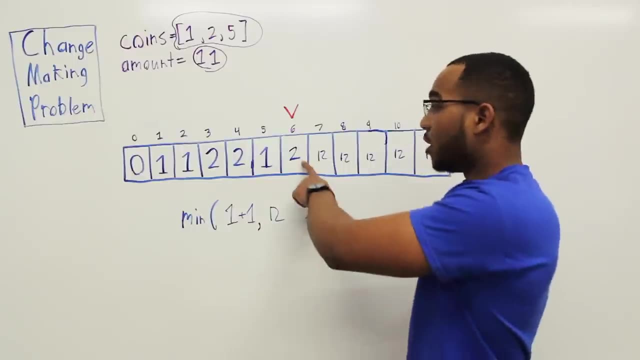 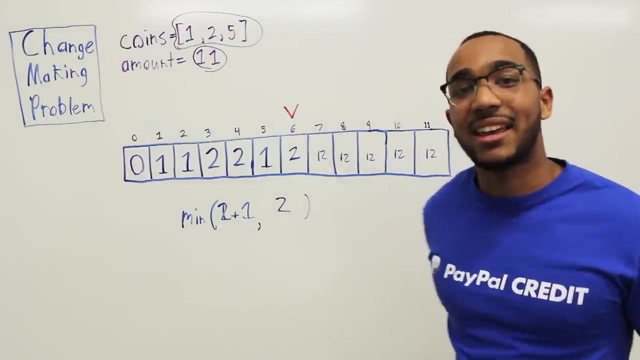 try coin: two, Six minus two is four, Four. the best answer is two. Two plus one is three, Three versus the best answer we have so far, which is two, Two plus one is three. Three is greater than two. It does not be our best answer, so we do not take. 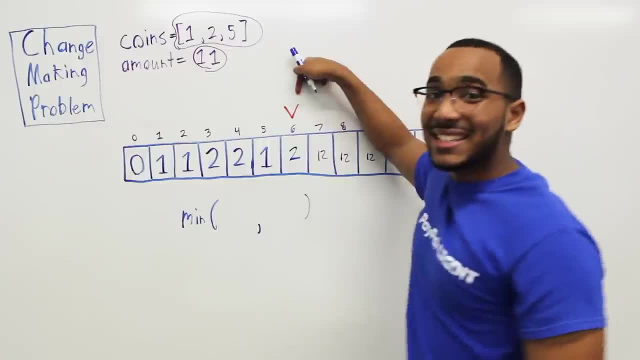 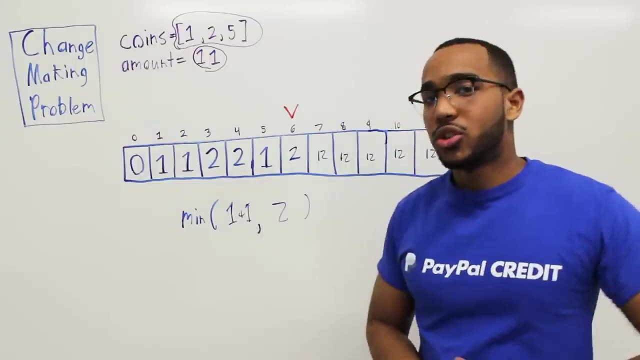 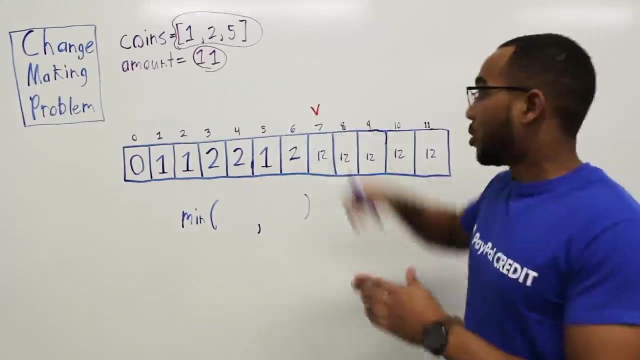 it. Now we try our final coin. We try the five. Six minus five is one, One, One plus one, One plus one versus two, Two versus two. It does not change your answer. the best answer for our sub problem at six is two coins. So now we're at seven. 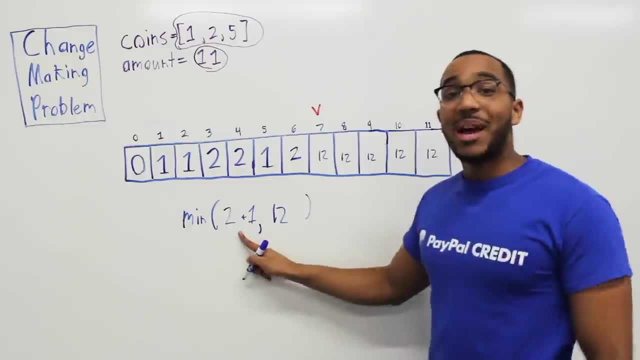 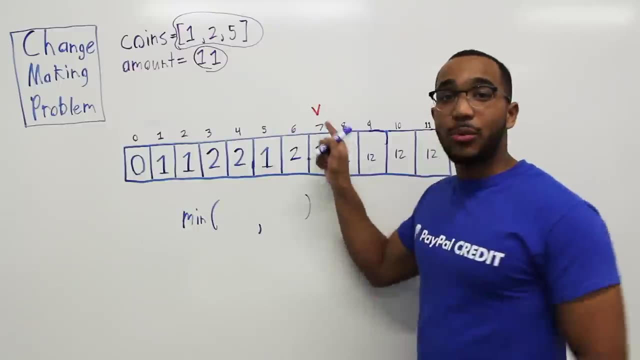 Seven minus one is six. Two, Two plus one. The best answer we had was to add one to that, versus twelve. The best answer is three now. And so now we tried the one coin, Let's try the two coin. Seven minus two is five, Now five. the best answer is: 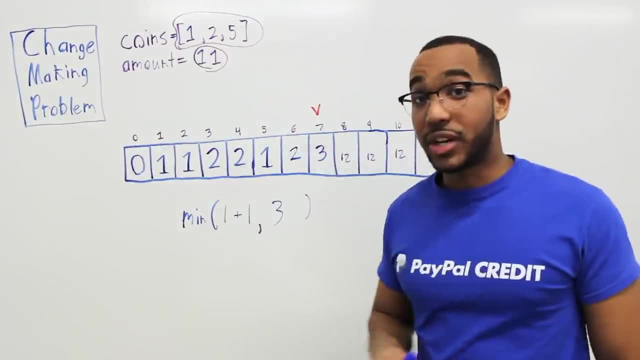 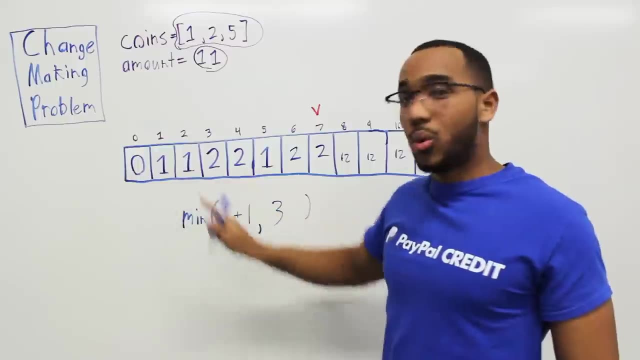 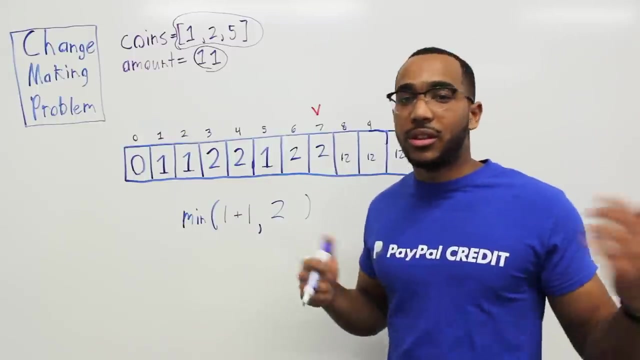 one, And one plus one is two. One plus one versus three: Two is the winner. And so now let's try the five, Five coins. Seven minus five is two. One plus one. One plus one stays versus two. One plus one versus two: The winner is still two. Nothing happens. So the best answer at seven: 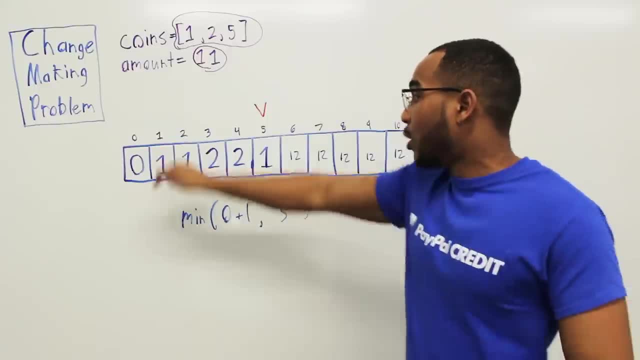 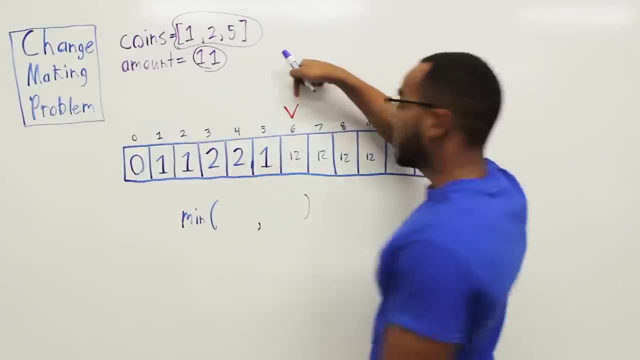 It is 1.. That is the answer to our sub-problem. We have solved this, this, this, this and this. We have solved 6 sub-problems And now we're going to continue on. So now I am at sub-problem 6.. 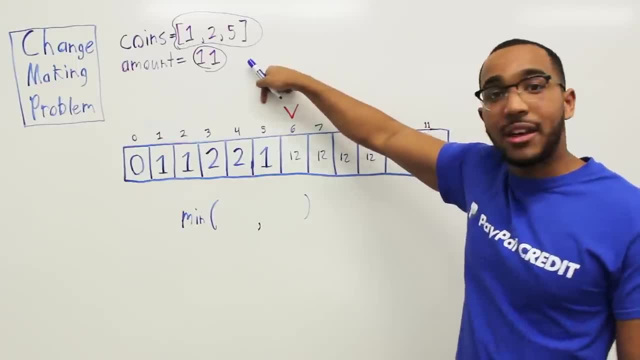 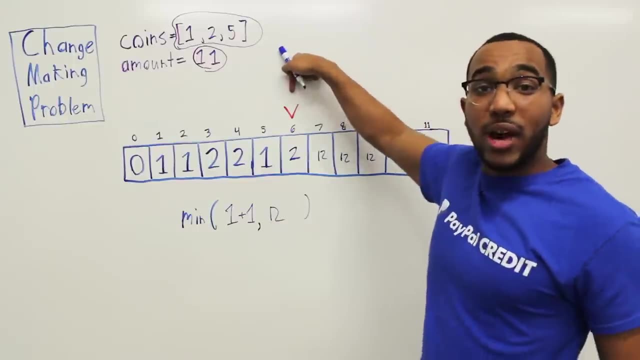 So if I try the 1 coin, 6 minus 1 is 5.. The best answer at 5 is 1. 1 plus 1.. 1 plus 1 versus 12. 2 is the winner And I want to try coin 2.. 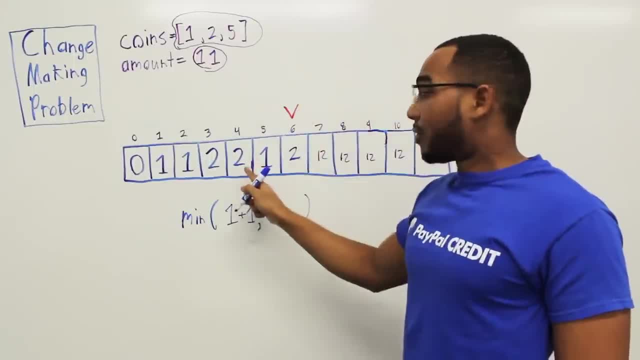 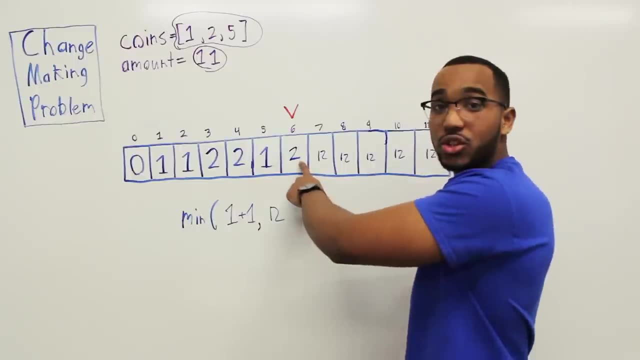 6 minus 2 is 4. 4.. The best answer is 2.. 2 plus 1 is 3. 3, versus the best answer we have so far, which is 2. 2 plus 1 is 3.. 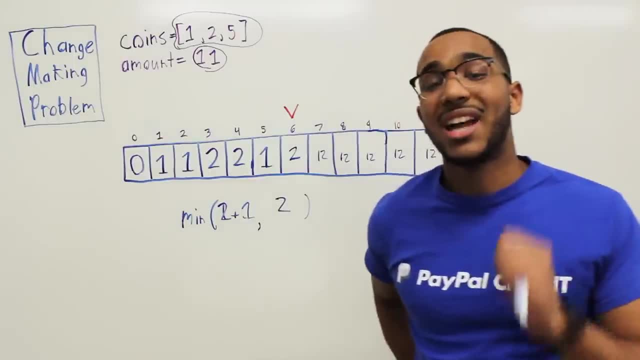 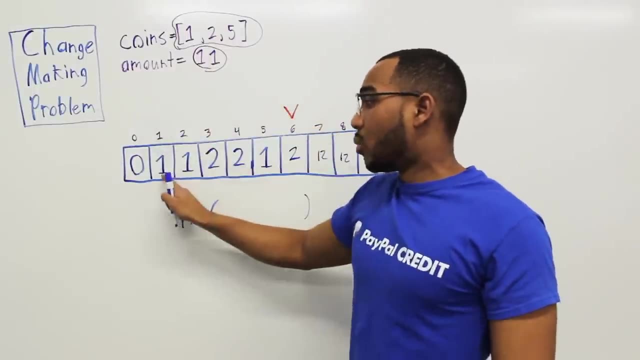 3 is greater than 2.. It does not beat our best answer, So we do not take it. Now we try our final coin. We try the 5.. 6 minus 5 is 1.. 1.. 1 plus 1.. 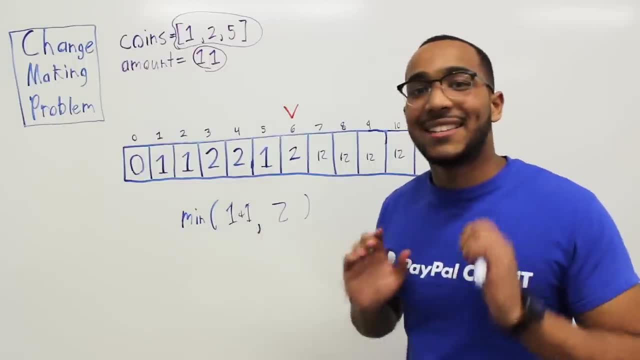 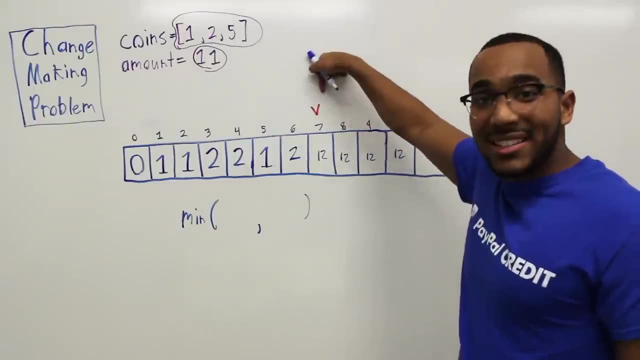 1 plus 1 versus 2.. 2 versus 2.. It does not change our answer. The best answer for our sub-problem at 6 is 2 coins. So now we're at 7.. 7 minus 1 is 6.. 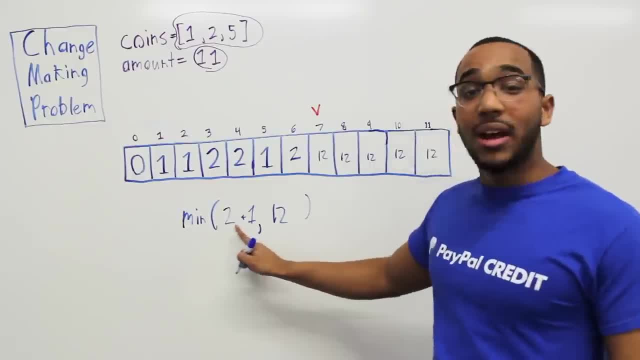 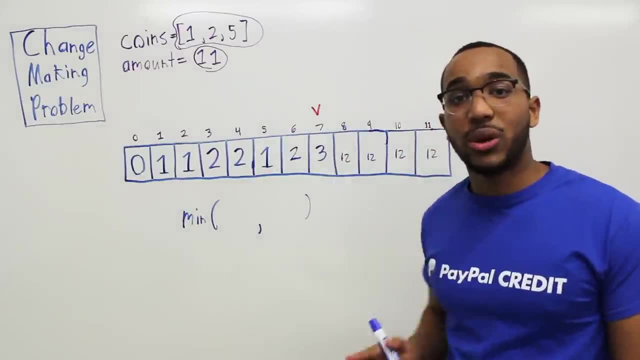 2. 2 plus 1. The best answer we had was 2. Add 1 to that versus 12.. The best answer is 3 now. And so now we try the 1 coin, Let's try the 2 coin. 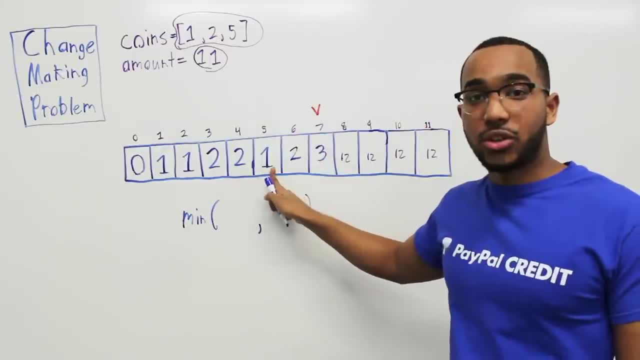 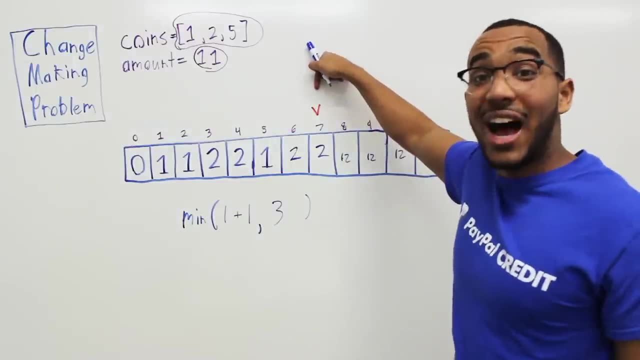 7 minus 2 is 5.. Now 5.. The best answer is 1. And 1 plus 1 is 2.. 1 plus 1 versus 3. 2 is the winner. And so now let's try the 5 coin. 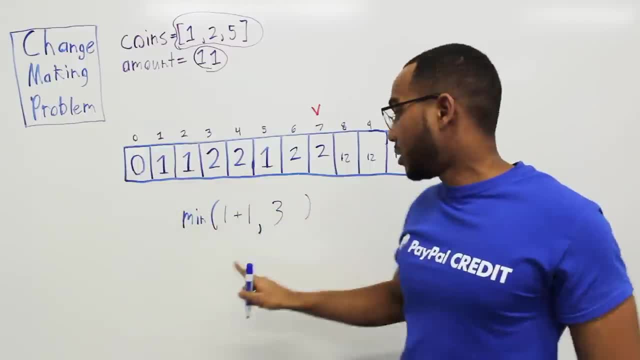 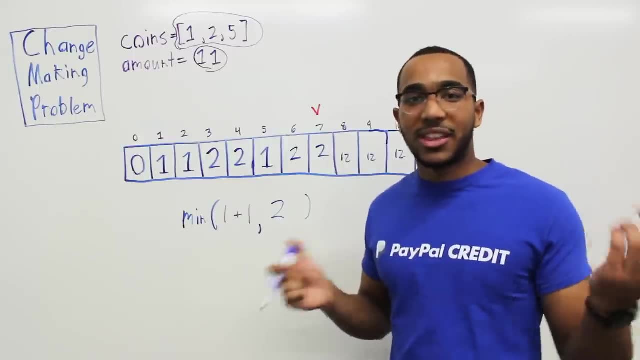 7 minus 5 is 2. 1 plus 1.. 1 plus 1 stays versus 2. 1 plus 1 versus 2. The winner is still 2. Nothing happens, So the best answer at 7.. 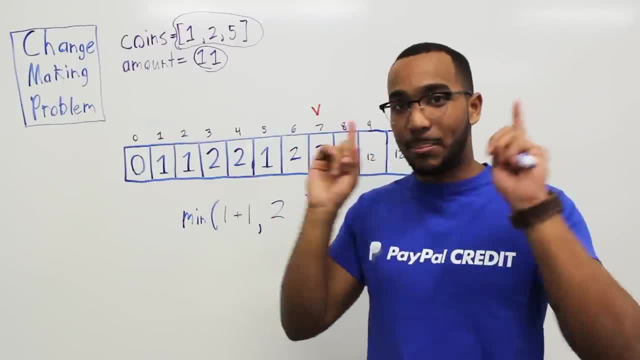 We've tried 1,, 2, and 5.. We've tried all our coins. The best answer at 7 is going to be using 2 coins. If we notice, it's going to be the 5 coin and the 2 coin. 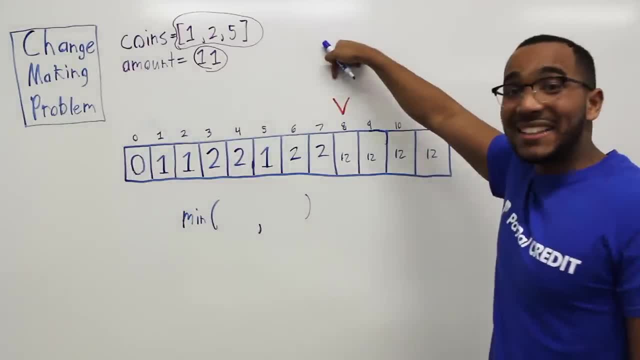 Those add up to 7.. So let's move on. So now we're at 8.. So if I use 1, the best answer is 2.. So 2 plus 1. 3 versus 12.. 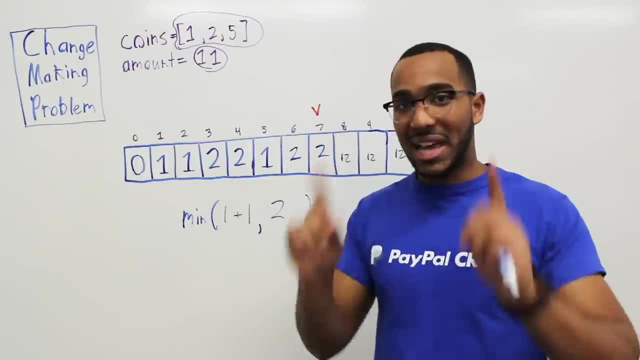 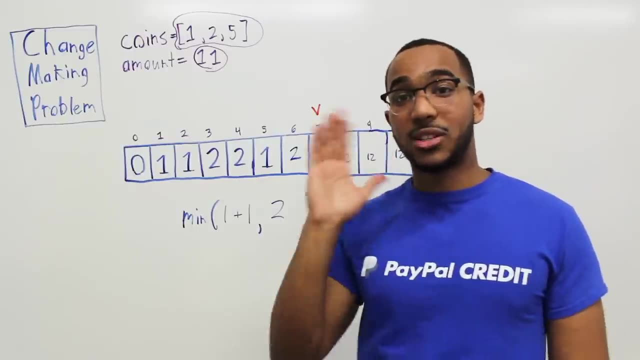 We've tried one, two and five. We've tried all our coins. The best answer at seven is going to be using two coins. If we notice, it's going to be the five coin and the two coin. Those add up to seven, So let's move on. So now we're at eight. So if I use one, 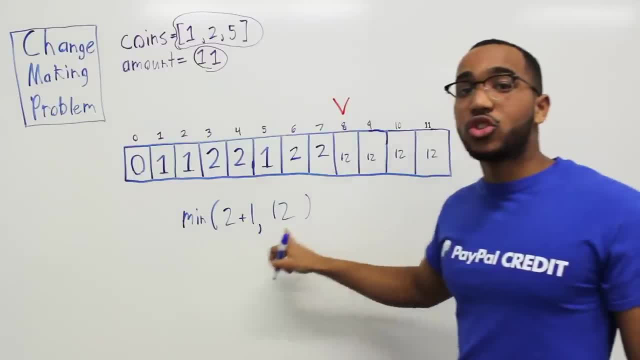 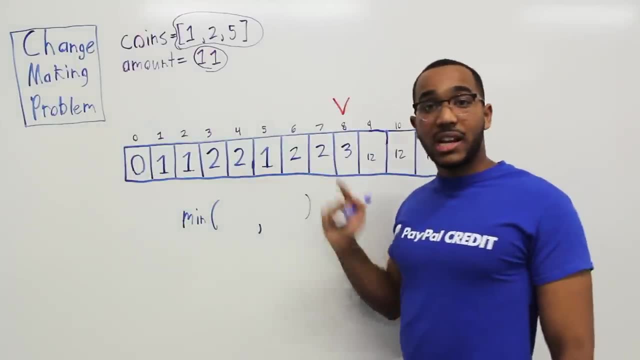 the best answer is two, So now we're at eight. So if I use one, the best answer is two. So two plus one, Three versus twelve, Three wins. So now, if I try the two coin, Eight minus two is six, Two plus one is three, Three versus three, nothing happens. 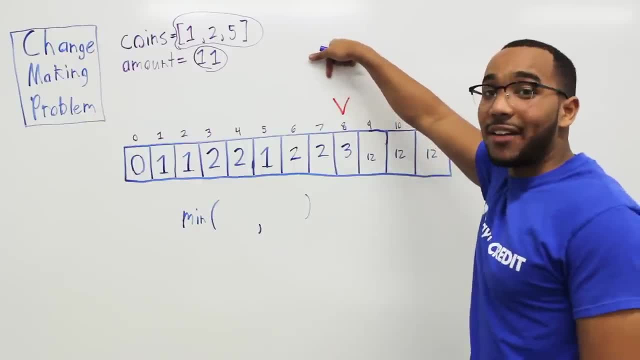 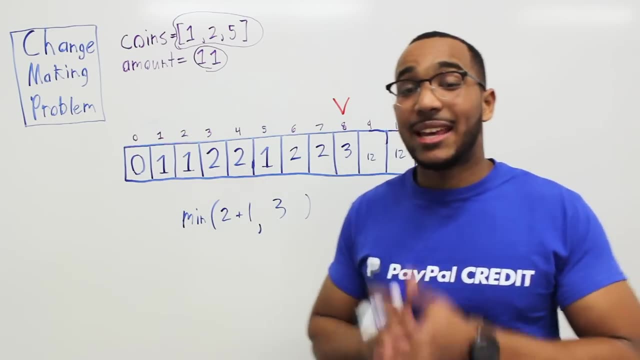 Let's try our next coin. Let's try the five. Eight minus five is three. Two plus one is three. Three versus three. None of the coins we tried improved our sub-problem. So now the best answer: we have The minimum amount of coins to make change. at eight It's going. 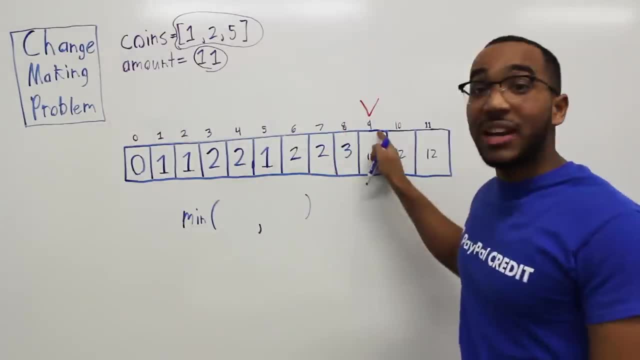 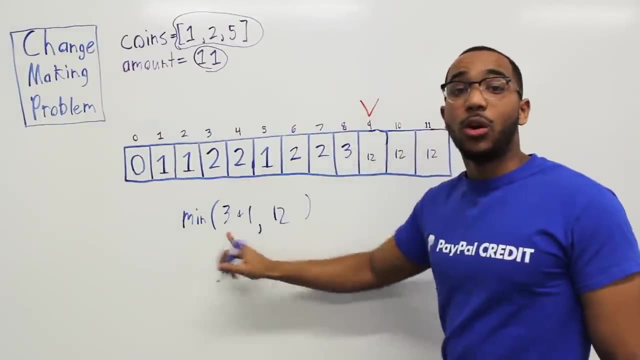 to make change. at 8 is going to be 3 coins. So now, if we use the 1 coin, we reach the 8, and now we do 3 plus 1.. 4 versus 12,, 4 wins. So now we try the 2 coin: 9 minus 2 is 7.. The best answer is 2 at our 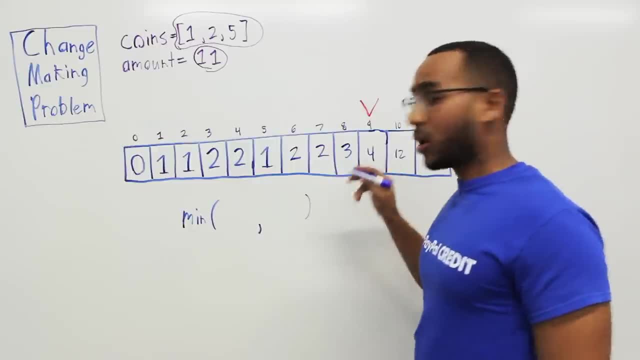 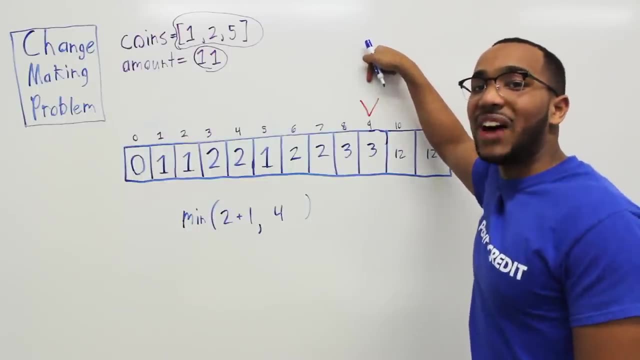 place 7.. So we do 2 plus 1 versus 4.. So now 3 beats 4, so 3 is our new best answer. So we tried the 1 coin, We tried the 2 coin. Now let's try the 5 coin. 9 minus 5 is 4.. So now 2 plus 1 is 3.. We have 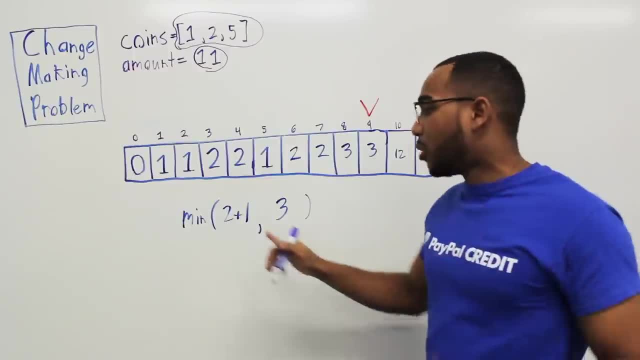 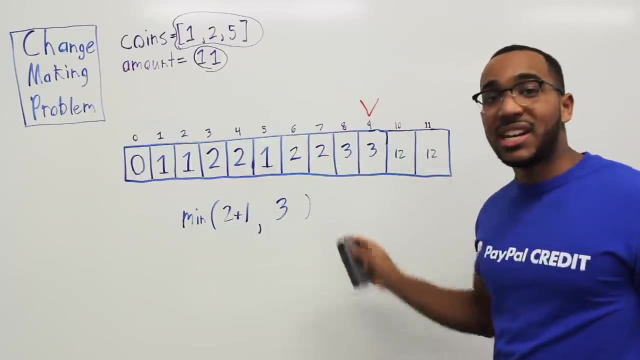 2 plus 1 versus 3.. So what we do is we won't do anything because 3 will not beat 3.. So now we tried 1,, 2, and 5. The answer to our sub problem at 9 is 3 minimum coins. So now we're almost to. 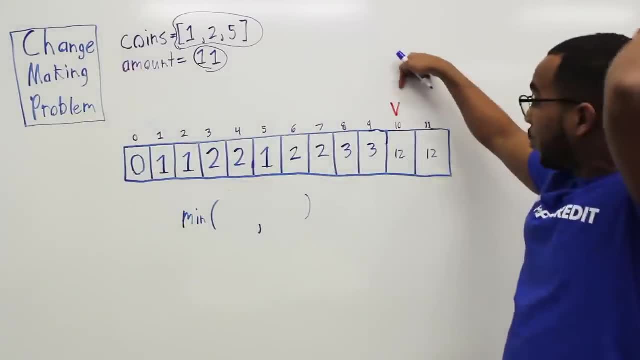 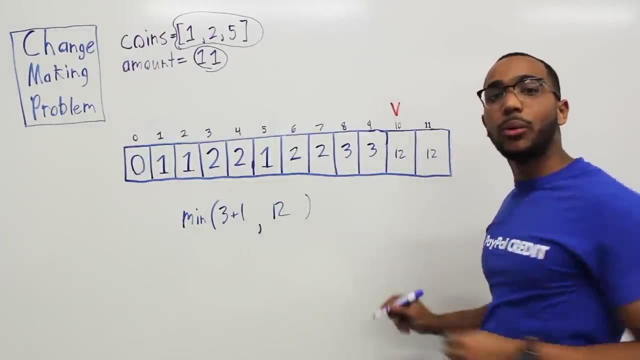 the final solution, which is going to be a 12.. So we try the 1 coin: 3 plus 1.. We do 10 minus 9.. Better, The best answer at 9 is 3.. 3 plus 1 versus 12. 4 wins, So now 4.. So we've tried the 1 coin. Let's. 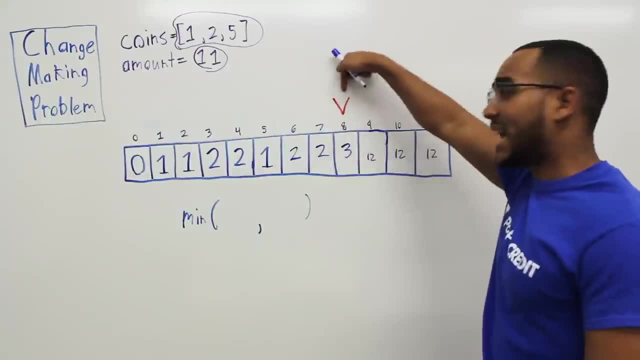 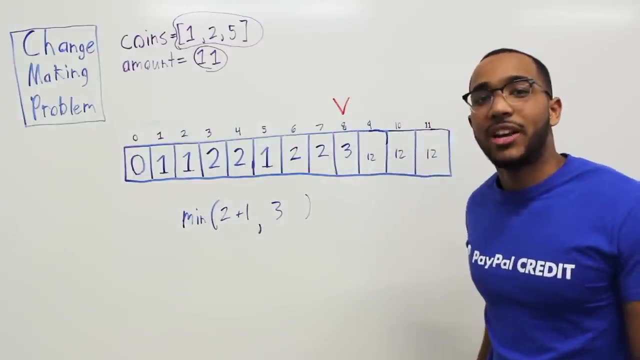 3 wins. So now, if I try the 2 coin, 8 minus 2 is 6.. 2 plus 1 is 3.. 3 versus 3. Nothing happens. Let's try our next coin, Let's try the 5.. 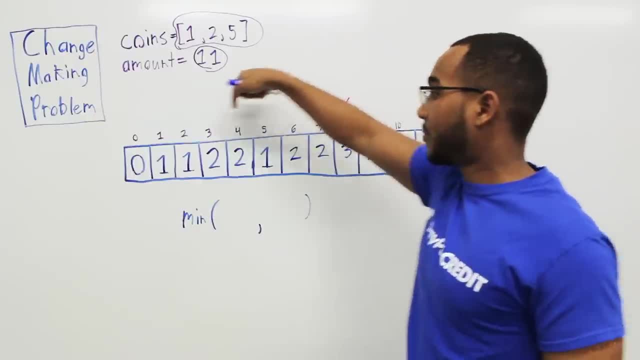 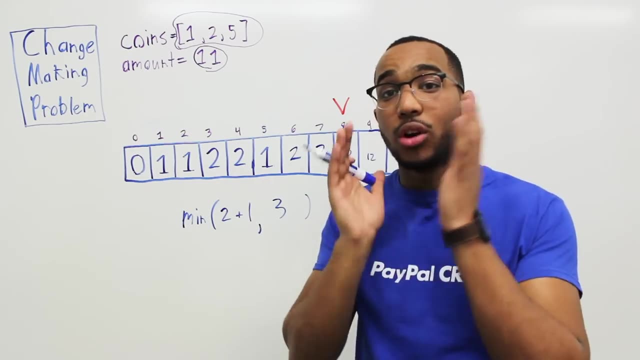 8 minus 5 is 3.. 2 plus 1 is 3.. 3 versus 3.. None of the coins we tried improved our sub-problem. So now the best answer: we have The minimum amount of coins to make changes. 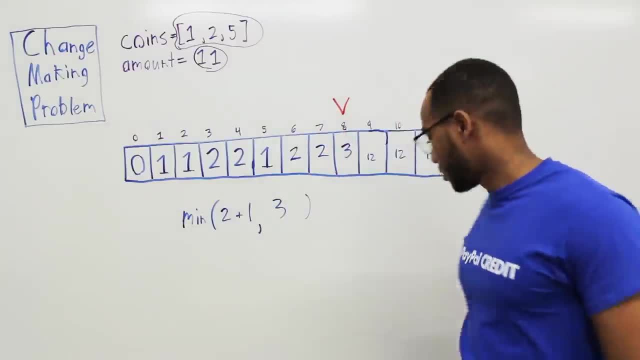 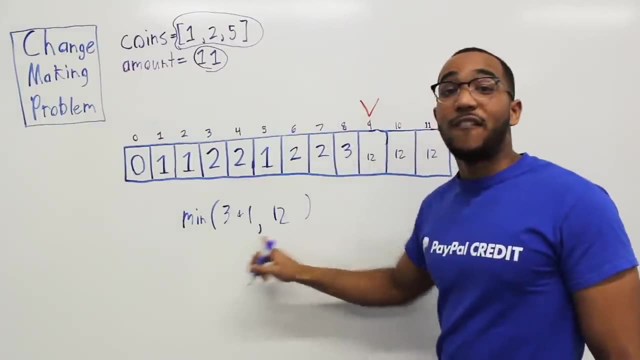 The minimum amount of coins to make change at 8 is going to be 3 coins. So now, if we use the 1 coin, we reach the 8. And now we do 3 plus 1.. 4 versus 12.. 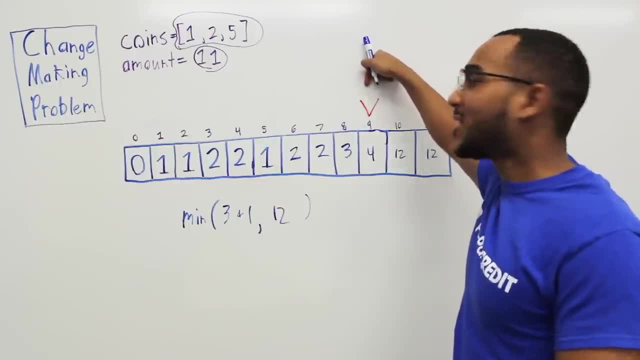 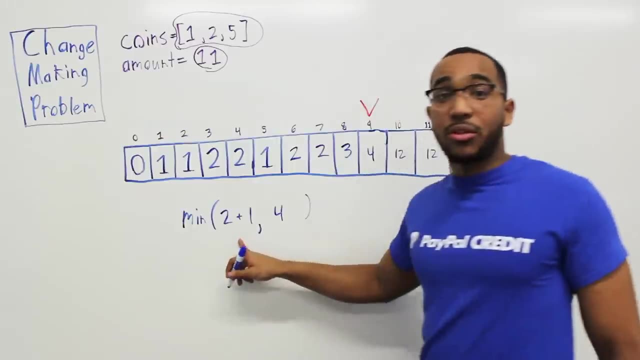 4 wins. So now we try the 2 coin: 9 minus 2 is 7.. The best answer is 2 at our place 7.. So we do 2 plus 1 versus 4.. So now 3 beats 4.. 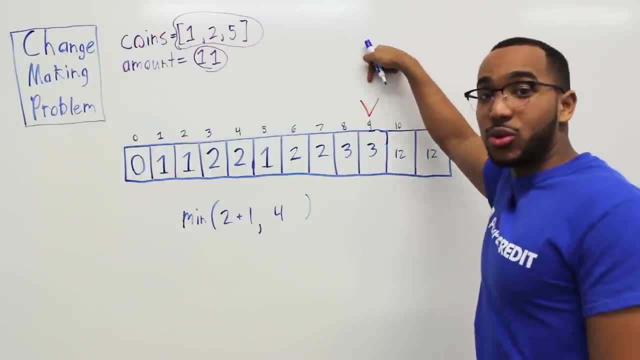 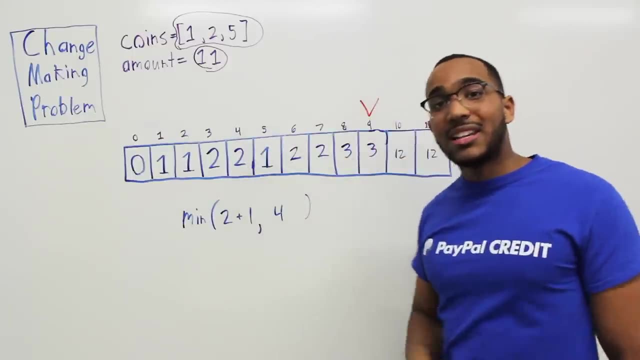 So 3 is our new best answer. So we tried the 1 coin, We tried the 2 coin, Now let's try the 5 coin. 9 minus 5 is 4.. So now 2 plus 1 is 3.. 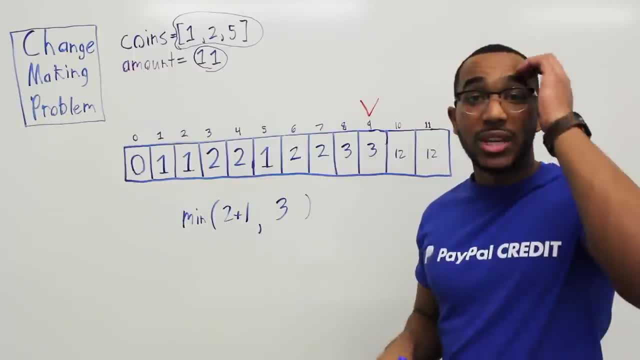 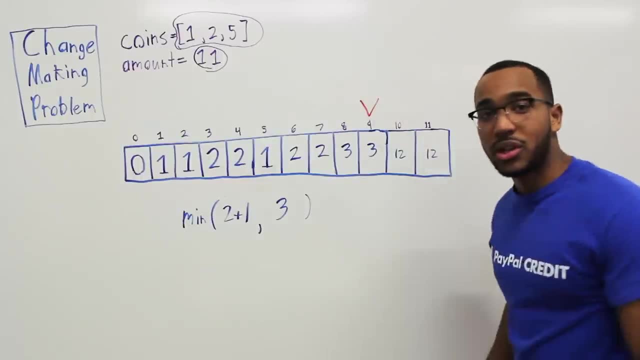 We have 2 plus 1 versus 3.. So what we do is we won't do anything, because 3 will not beat 3.. So now we tried 1,, 2, and 5.. The answer to our sub-problem at 9 is 3 minimum coins. 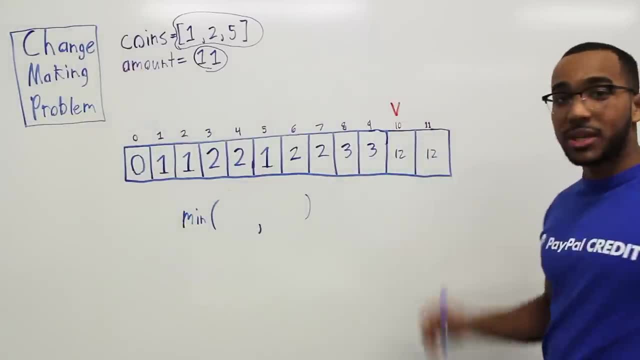 So now we're almost to the final solution, which is going to be a 12.. So we try the 1 coin: 3 plus 1.. We do 10 minus 9.. Best answer at 9 is 3.. 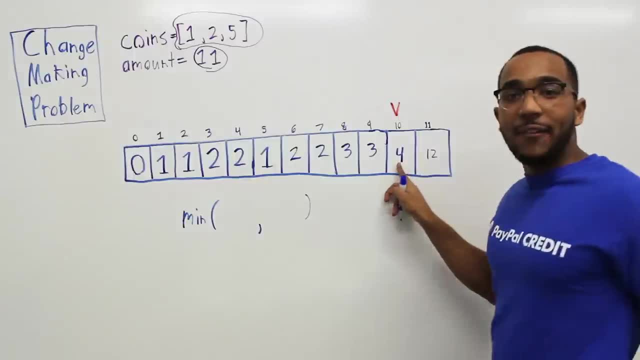 3 plus 1 versus 12.. 4 wins. So now 4.. So we've tried the 1 coin. Let's try the 2 coin. 10 minus 2 is 8.. The best answer is 3.. 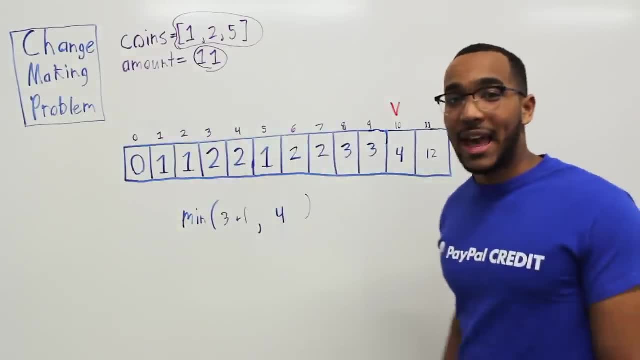 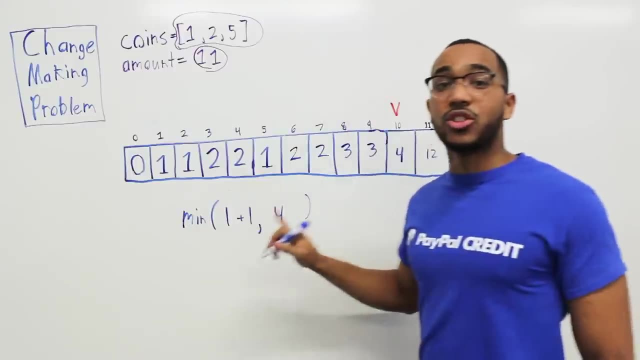 3 plus 1.. 3 plus 1 versus 4. Nothing happens. Let's try the 5 coin. 10 minus 5 is 5. 5. The best answer at 5 was 1.. 2 versus 4.. 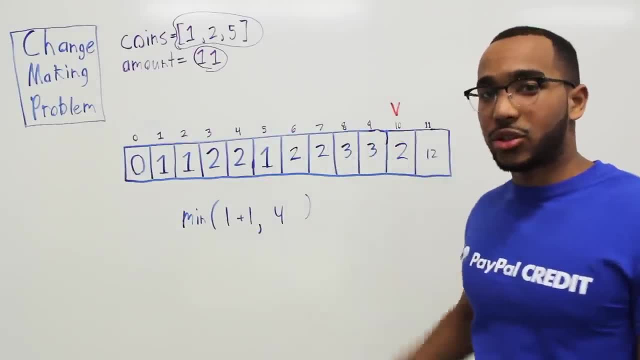 2 is the winner. We've tried all our coins and the best answer is 2.. If we have a mount 10, we can use a 5 and a 5.. We can use a 5 and then a 5.. 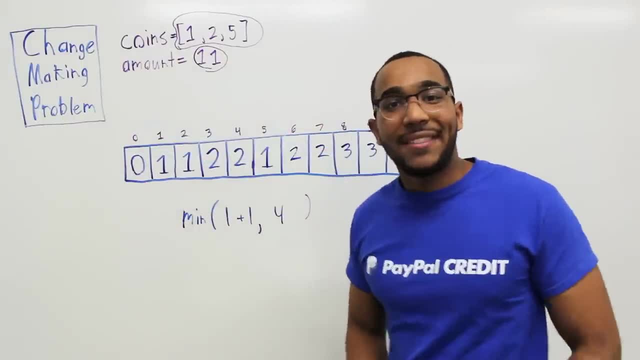 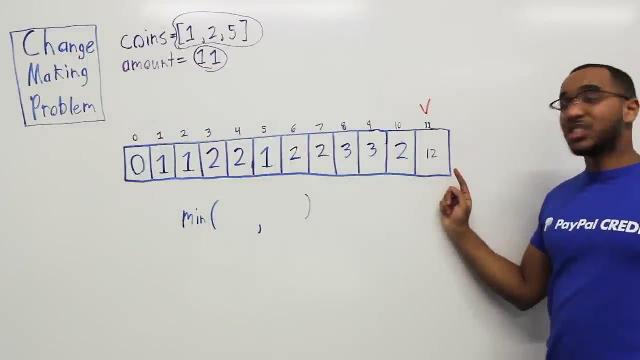 A 5 to get change, take us to 0, and that is the answer to our subproblem. So now we've reached our final subproblem. This is the answer we want, And now we try making change with a 1.. 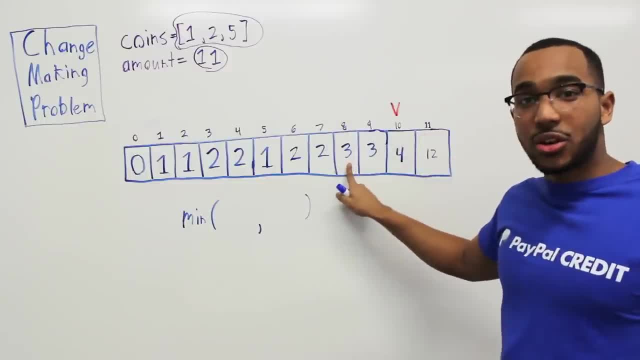 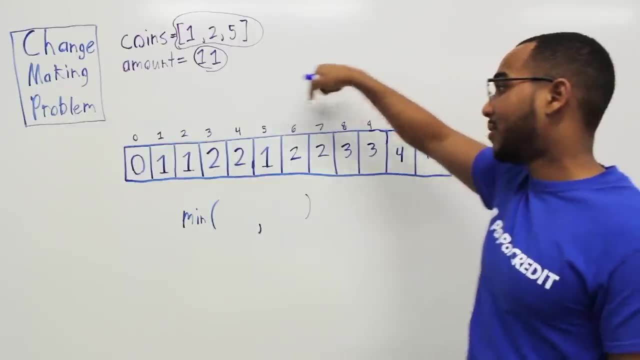 try the 2 coin: 10 minus 2 is 8.. The best answer is 3. 3 plus 1.. 3 plus 1 versus 4.. Nothing happens. Let's try the 5 coin: 10 minus 5 is 5. 5. The best answer at 5 was 1. 2 versus 4. 2 is the winner. 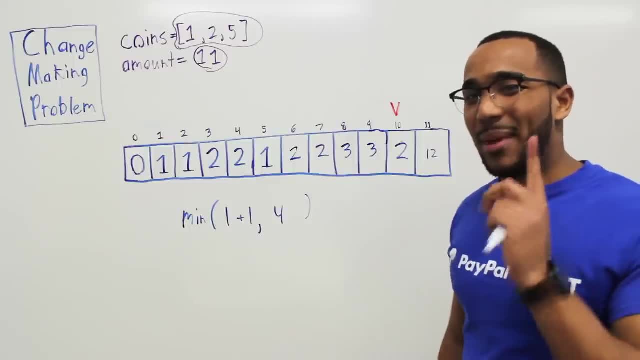 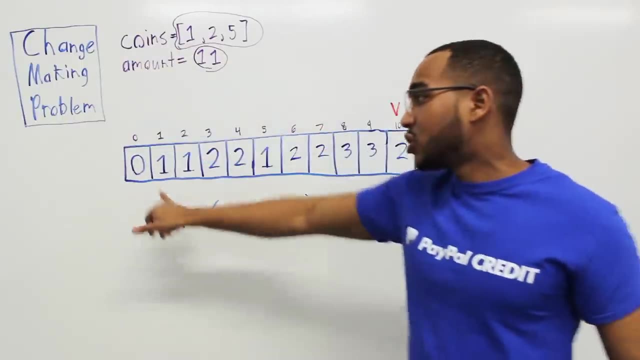 We've tried all our coins and the best answer is 2.. If we have a mount 10, we can use a 5 and a 5.. We can use a 5 and then a 5 to get change. Take us to 0 and that is the answer to our sub problem. So 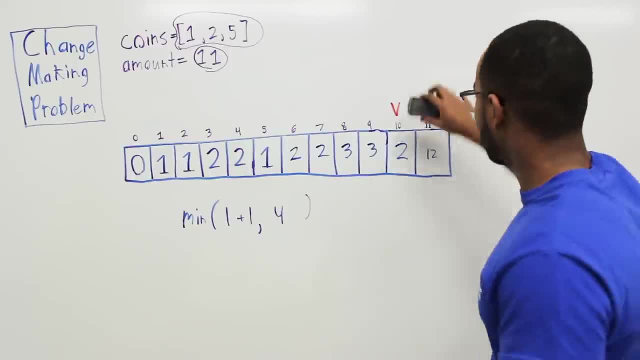 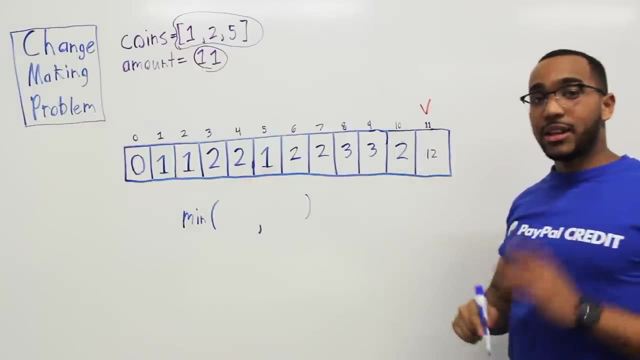 now we've reached our final sub problem. This is the answer we want, And now we try making change with a: 1. We do 11 minus 1 is 10.. The best answer at 10 is 2. We do 2 plus 1. 3 versus 12.. 3 is the. 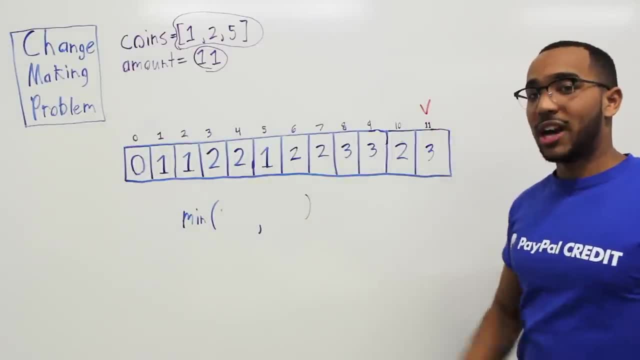 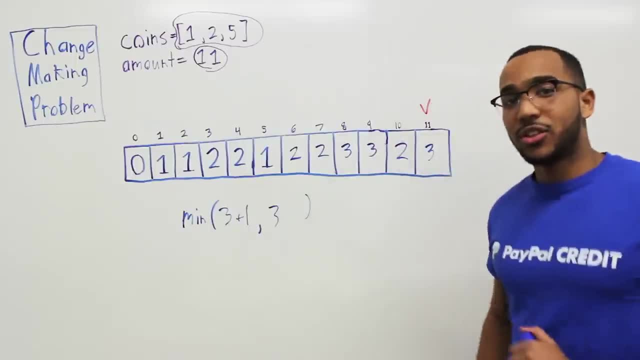 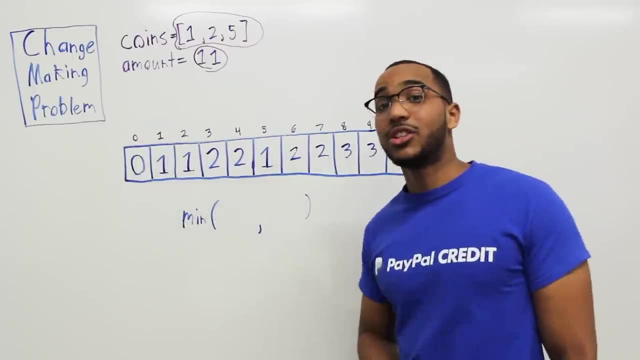 2. 9. Best answer at 9 is 3. 3 plus 1 versus 3. 4 does not beat 3.. We do not take it. We choose not to use 2 as the last coin to make change to 11.. That is a path we don't want to follow, because 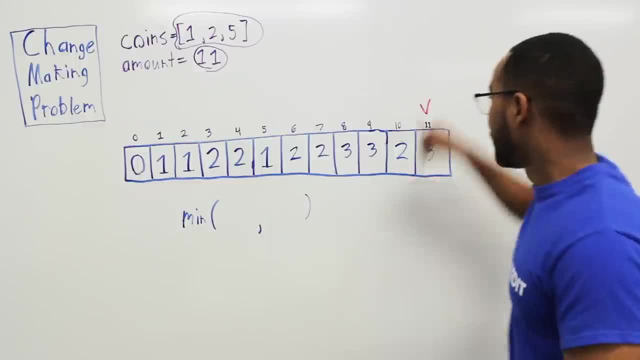 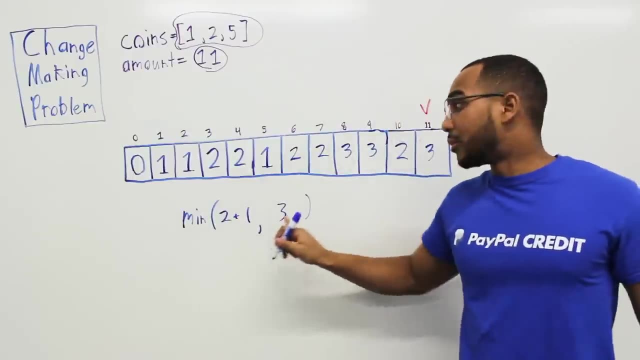 we will not get the best answer, So now we try 5.. 11 minus 5 is 6.. Our best answer is 2.. So now, 2 plus 1 is 3.. 3 does not beat 3.. It does not matter whether we take the path of subtracting. 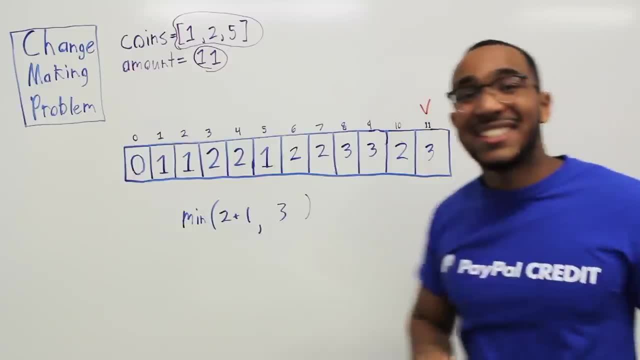 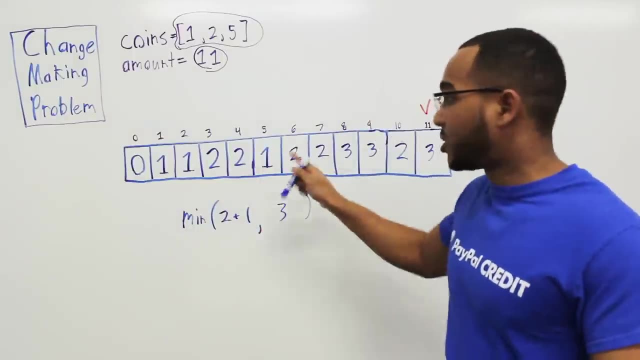 the 5 coin or the 1 coin From 11,, we will still be able to get our best answer: 3.. So each time the reason we're adding 1 to these best sub-problems is because we're using a coin. So this is the bottom-up approach. 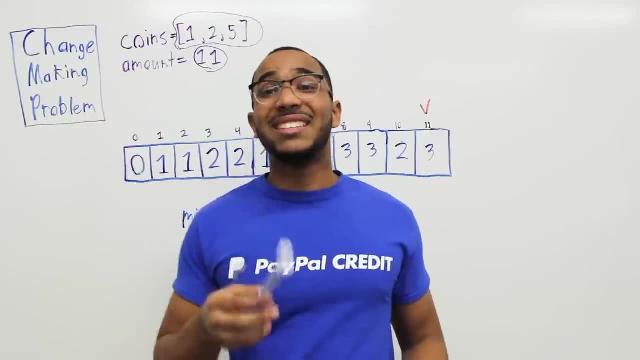 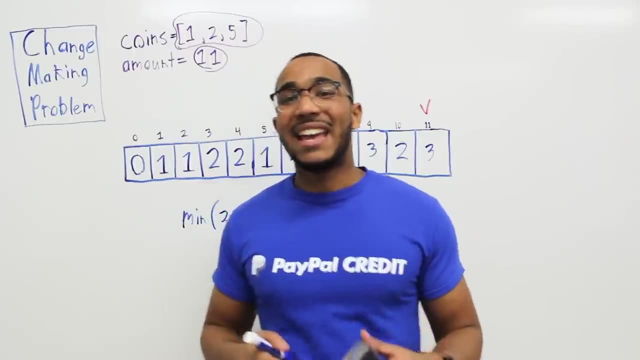 I wanted you to see the top-down and the bottom-up approach, because these dynamic programming problems often can be done both ways. whichever you are more comfortable with. Personally, I would say: get comfortable with both, Be proficient in both. But sometimes the iterative approach is a. 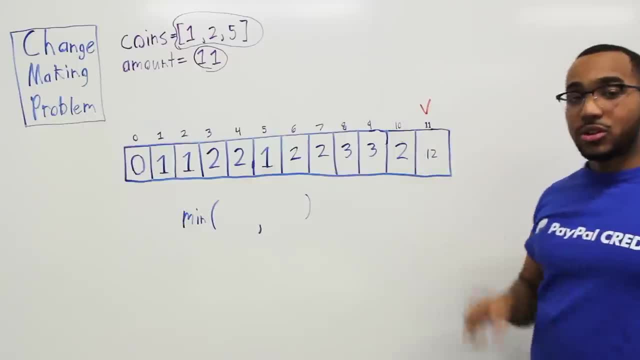 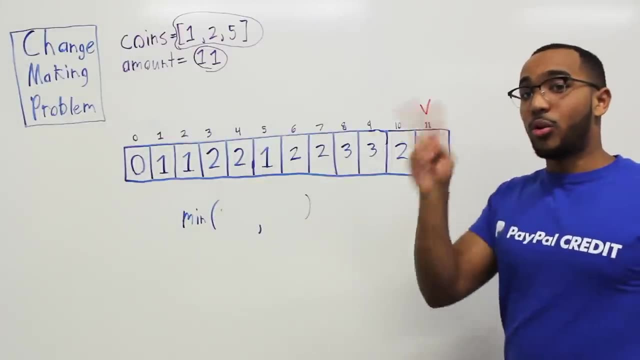 We do 11 minus 1 is 10.. The best answer at 10 is 2.. We do 2 plus 1.. 3 versus 12.. 3 is the winner. So what we do now is we try coin 2.. 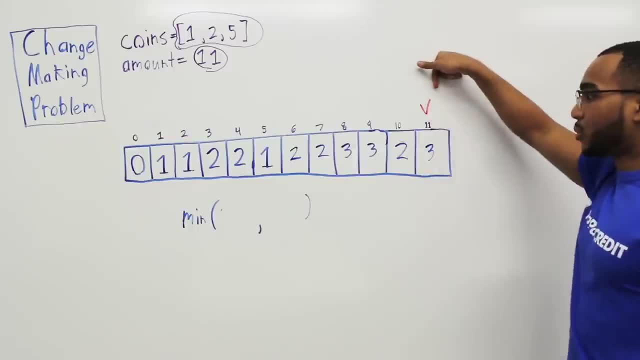 We just tried coin 1.. Let's try coin 2. So what we do is we do 11 minus 2, 9.. Best answer at 9 is 3. 3 plus 1 versus 3.. 4 does not beat 3.. 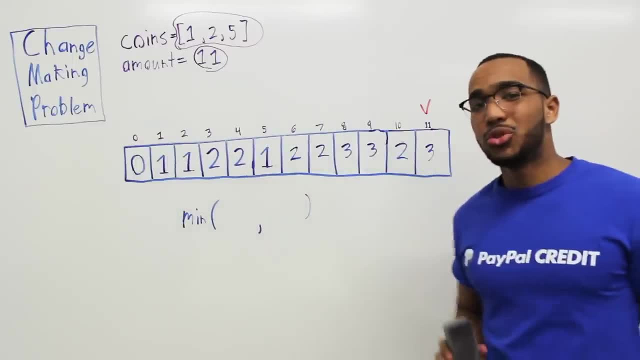 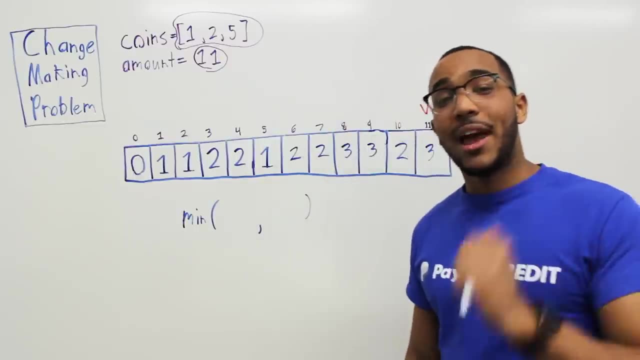 We do not take it. We choose not to use 2 as the last coin to make change to 11.. That is a path we don't want to follow because we will not get the best answer. So now we try 5.. 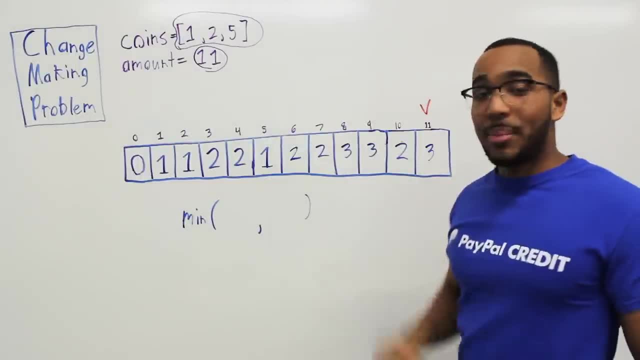 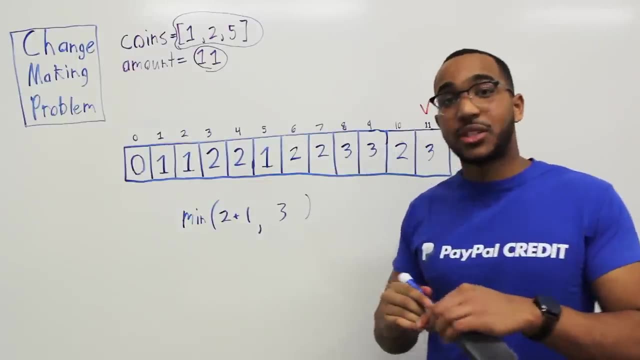 11 minus 5 is 6.. Our best answer is 2.. So now, 2 plus 1 is 3.. 3 does not beat 3.. It does not matter whether we take the path of subtracting the 5 coin or the 1 coin. 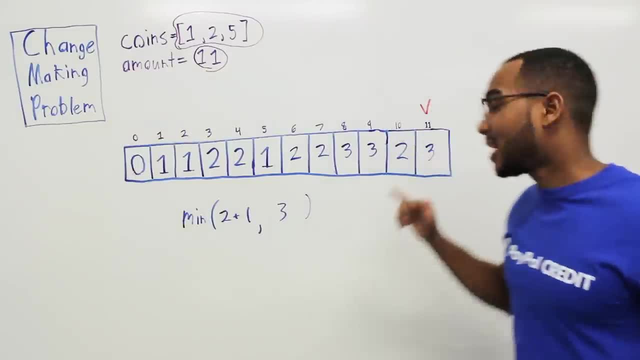 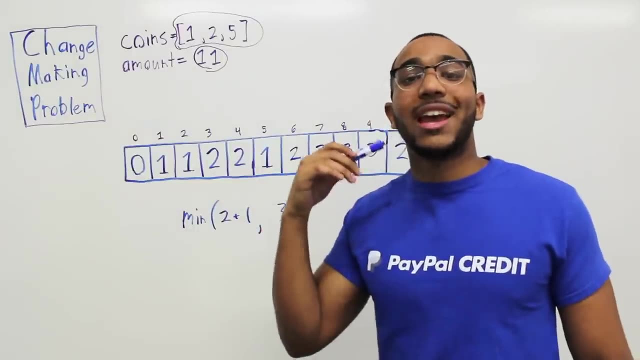 From 11,, we will still be able to get our best answer 3.. So each time, the reason we're adding 1 to these best subproblems is because we're using a coin. So this is the bottom-up approach. 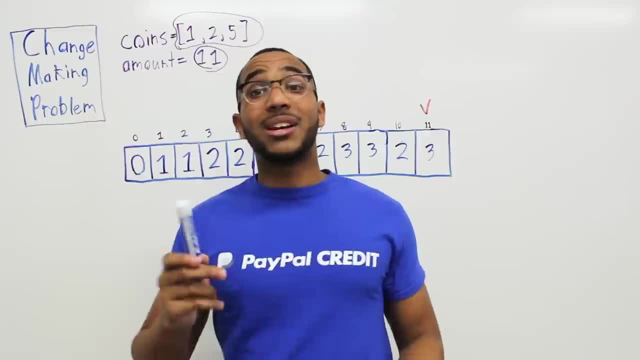 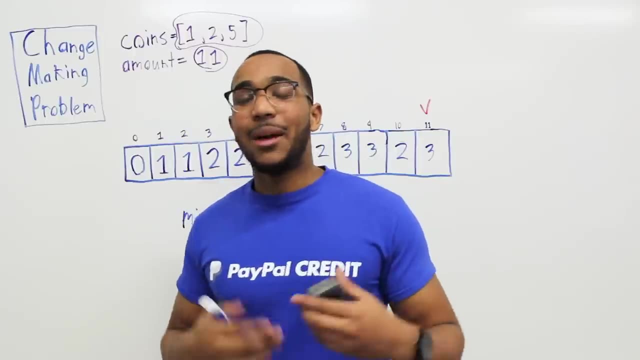 I wanted you to see the top-down and the bottom-up approach, because these dynamic programming problems often can be done both ways. whichever you are more comfortable with. Personally, I would say: get comfortable with both, Be proficient in both, But sometimes the iterative approach is a lot easier. 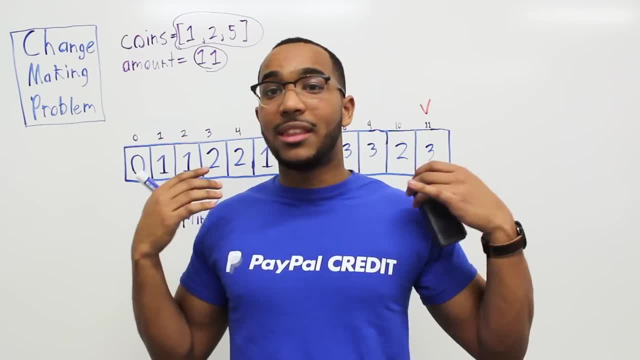 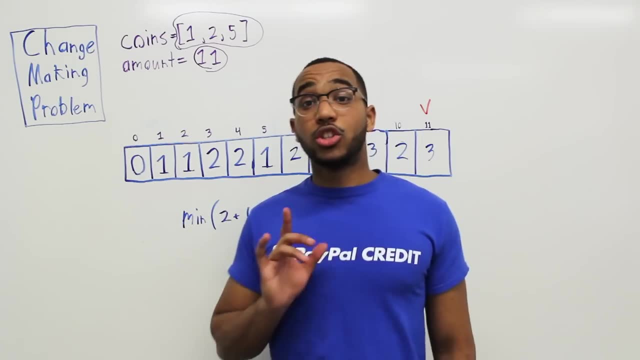 It's easier to implement because it's very more straightforward and you just need to know the pattern of the table. You don't so much need to know how the decisions get made and how all of that stuff pans out. So let's look at the time and space complexities. to wrap this thing up, 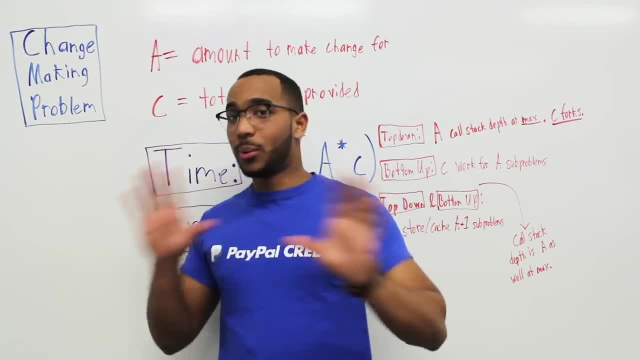 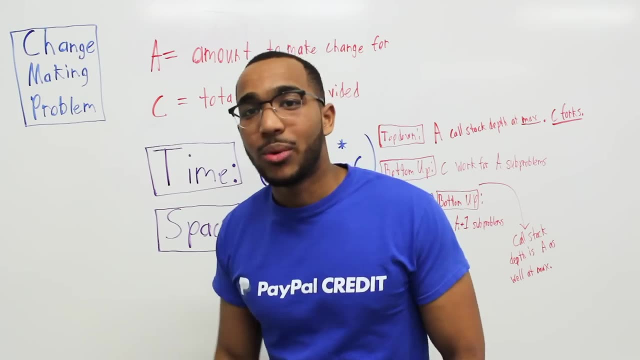 We're going to need to first declare our variables before we analyze complexity. So A is the amount we're given. If we're given to make change for an amount of 11, we need to make change for 5.. That is A. 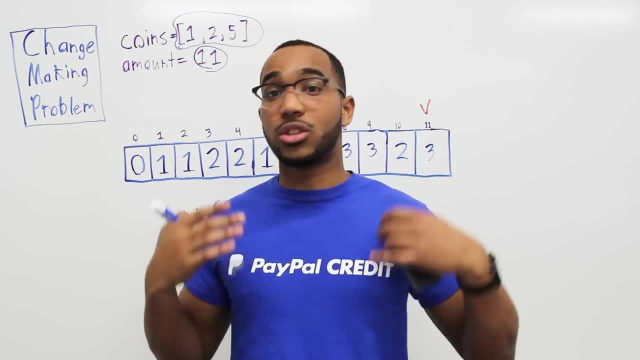 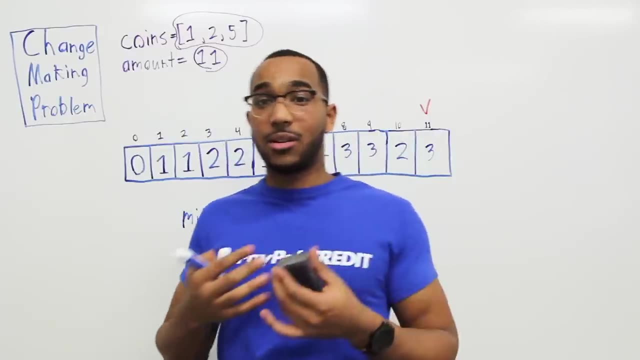 lot easier to implement because it's very more straightforward and you just need to know the pattern of the table. You don't so much need to know how the decisions get made and how all of that stuff pans out. So let's look at the time and space complexities to wrap this thing up. 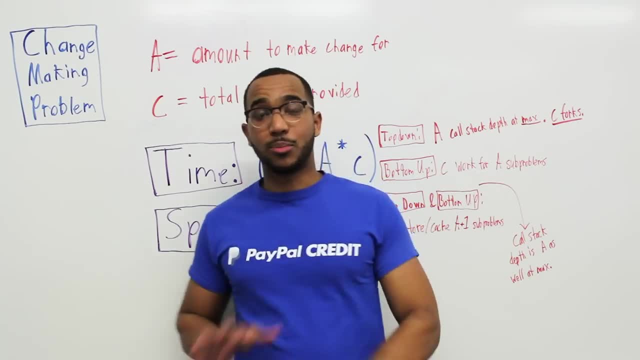 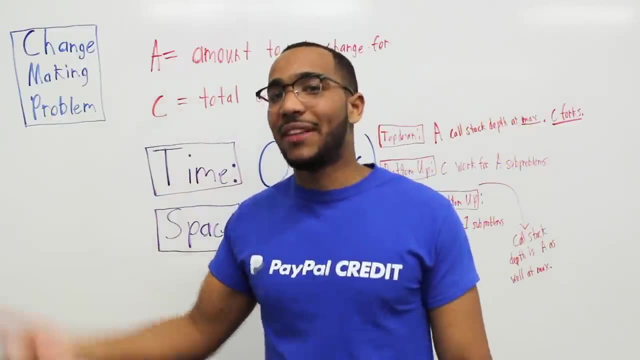 We're going to need to first declare our variables before we analyze complexity. So A is the amount we're given. If we're given to make change for an amount of 11, we need to make change for 5.. That is A. 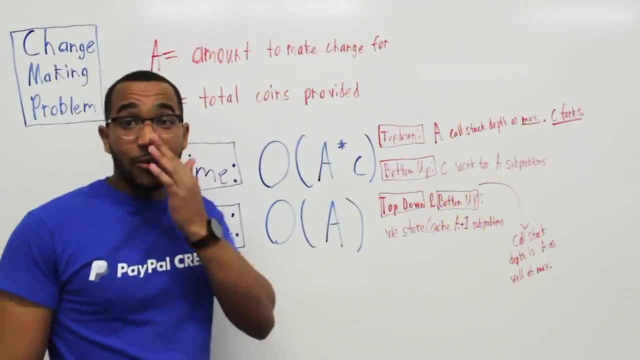 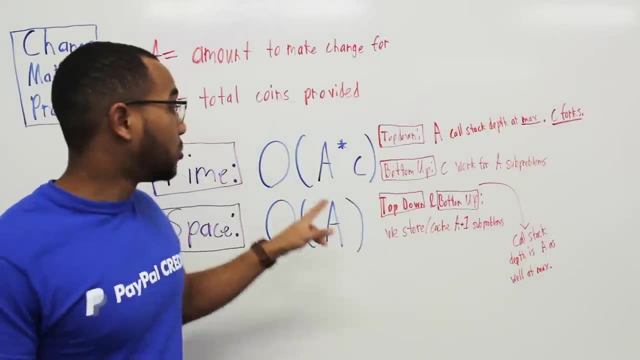 For the total denominations, the total coins we are given. If we're given a 1,, 2, and a 5, then C is going to be 3.. We're given 3 coins. Our time complexity is going to be A times C For the top-down approach. our 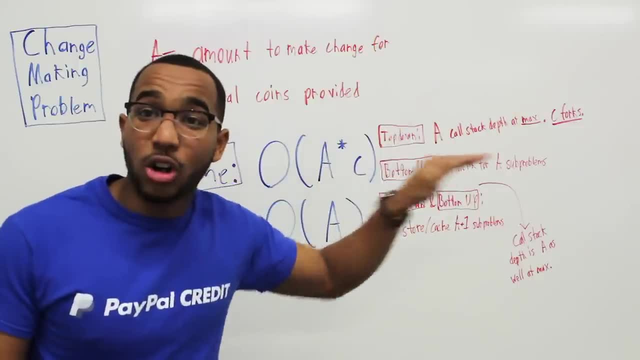 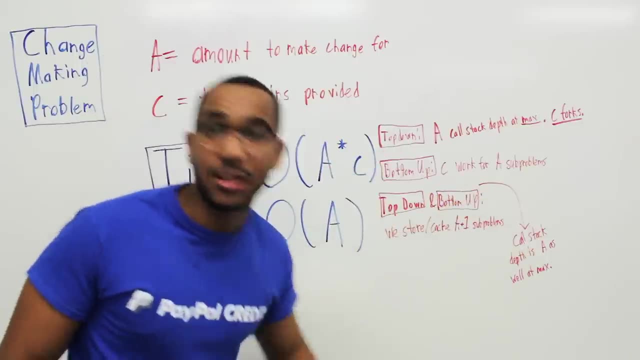 call stack at maximum is going to go 8 calls deep. If I subtract 1 from 11,, 1 from 10,, 1 from 9,, 1 from 8,, 1 from 7, then my call stack is going to be as deep as the amount that I'm given. 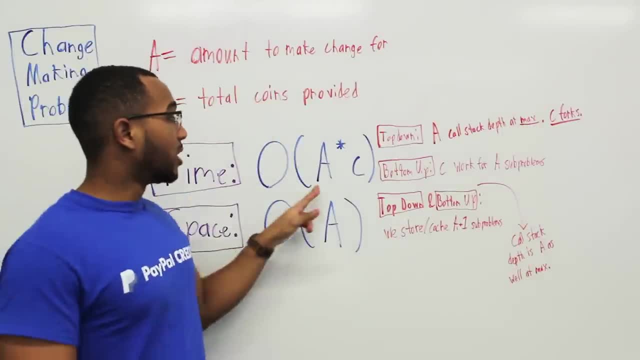 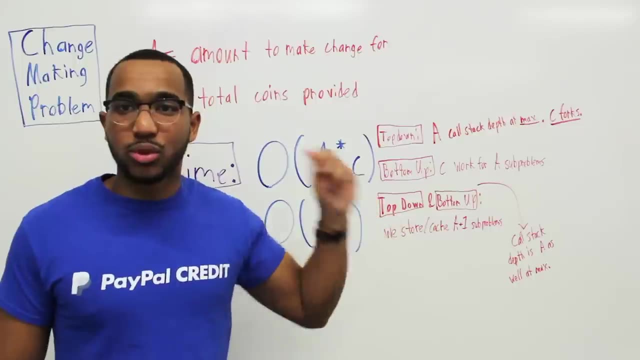 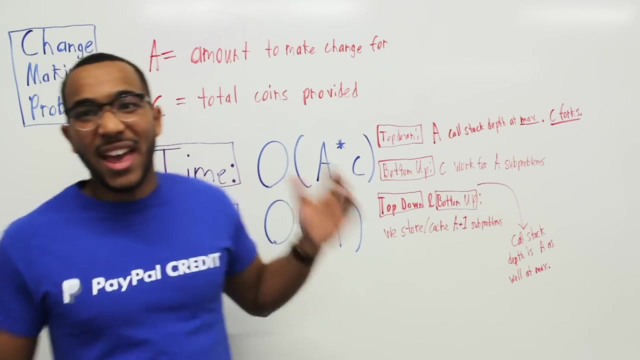 If we are caching answers on the way downwards, we are going to have a maximum, a depth of A. We are going to be doing at maximum C iterations. We're going to check C denominations, We're going to check all of our coins from each of those sub-problems that we solve and we're going to only solve A sub-problems. 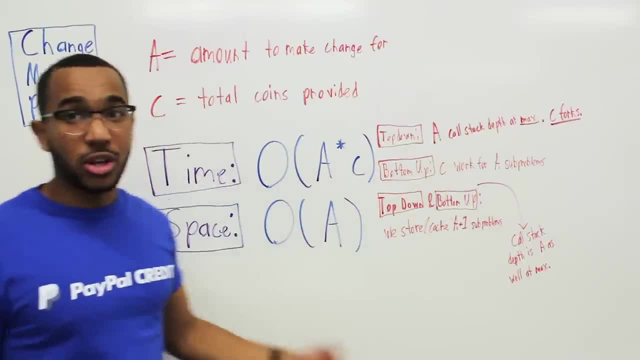 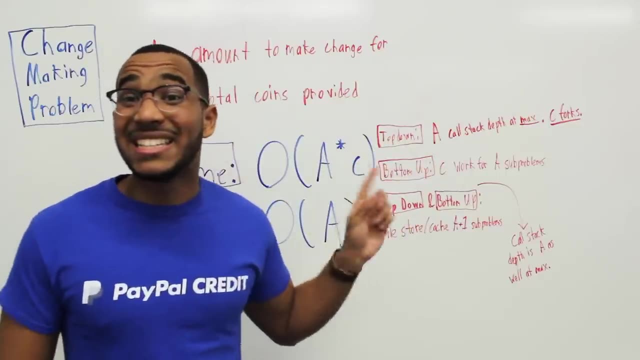 at max, because we are remembering the answers For the bottom-up approach. then we're just going to be iterating through our table and at each of the points in the table, we're going to be trying at maximum C coins. We're going to be trying at maximum C coins. We're going to be trying at maximum C coins. We're going to be doing. 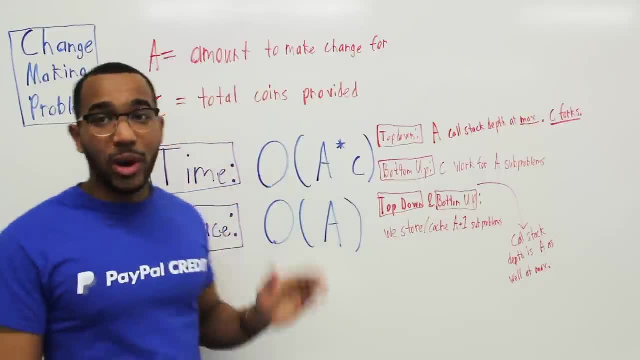 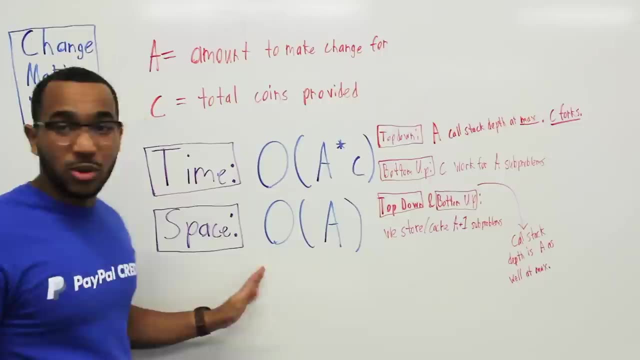 try at maximum all the coins we have, as you saw in our example. That is why it is A times C for both the bottom-up and the top-down approach. So let's look at the top-down, bottom-up for space. For space, we're going to be using O of A For both. 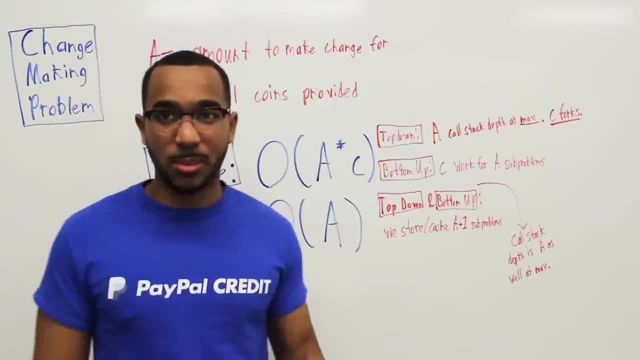 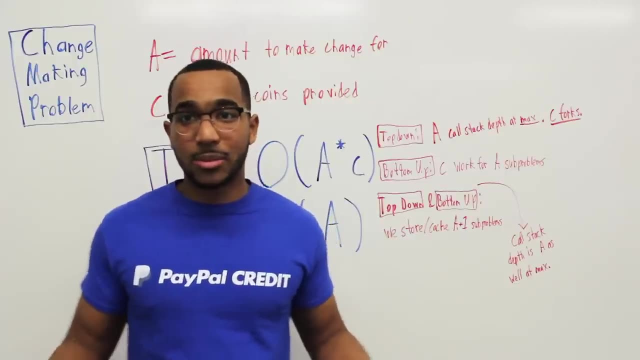 approaches. we're going to be caching the answers to A plus 1 subproblems. We're going to keep the answer to the 0 subproblem. You could count that in, count that out. but it's going to be about A subproblems For the top-down and bottom-up. 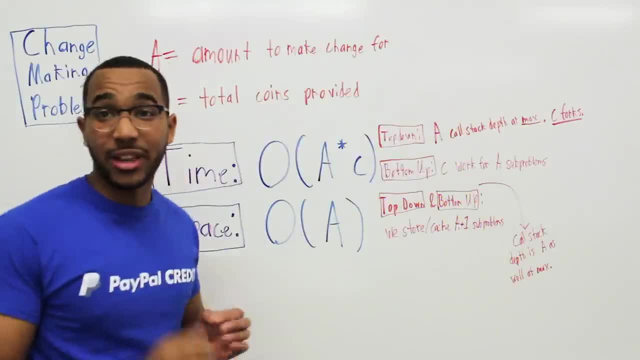 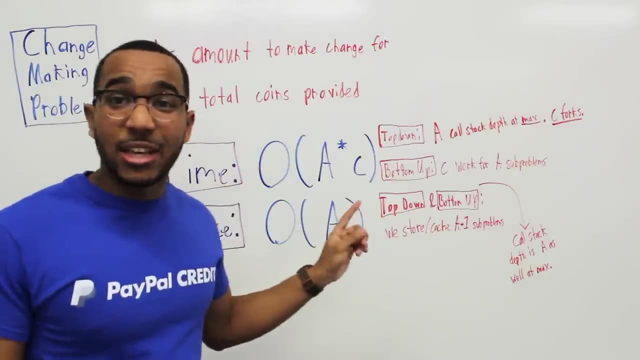 That is the total denominations, the total coins we are given. If we're given a 1,, 2, and a 5, then C is going to be 3.. We're given 3 coins. Our time complexity is going to be A times C. 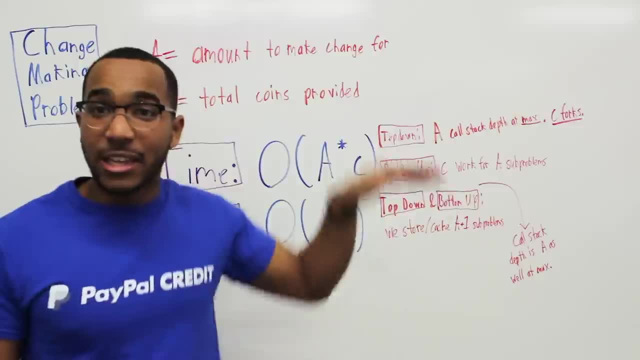 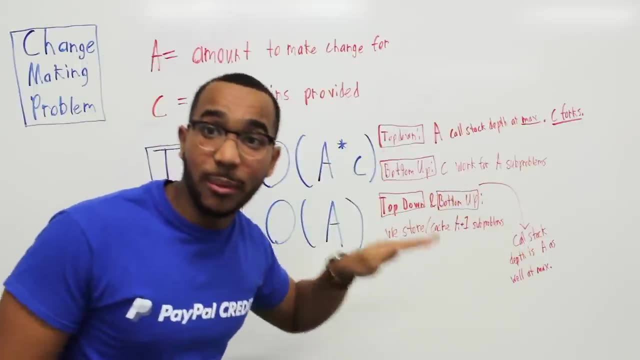 For the top-down approach, our call stack at maximum is going to go 8 calls deep If I subtract 1 from 11,, 1 from 10,, 1 from 9,, 1 from 8,, 1 from 7,. 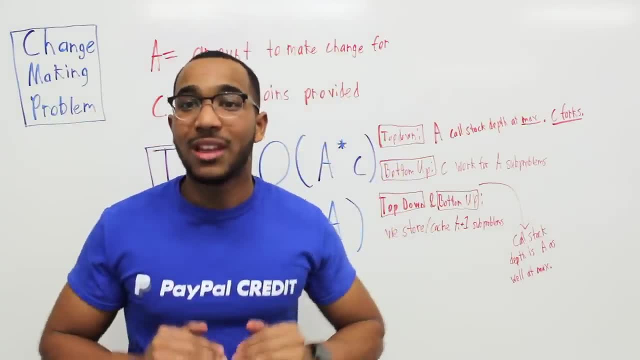 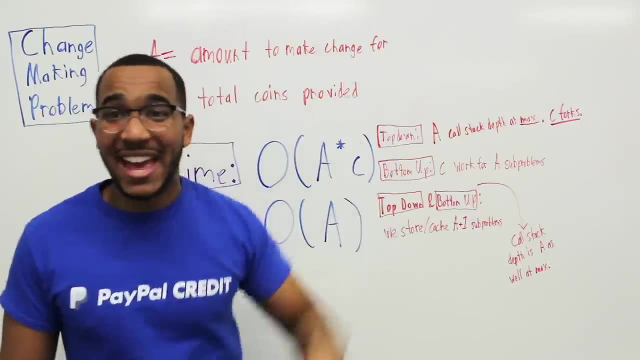 then my call stack is going to be as deep as the amount that I'm making change for I'm giving. If we are caching answers on the way downwards, we are going to have at maximum a depth of A. We are going to be doing at maximum C iterations. 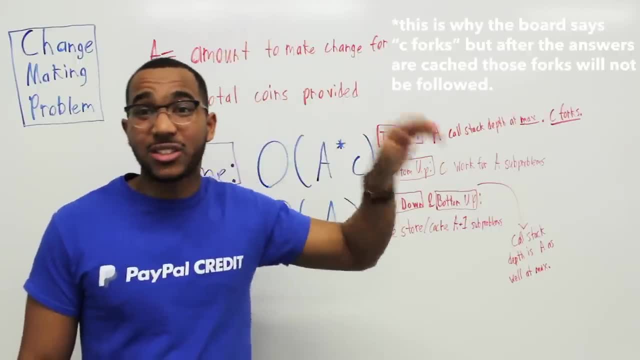 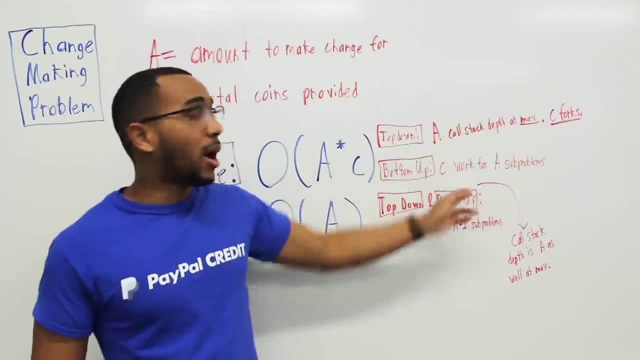 We're going to check C denominations, We're going to check all of our coins from each of those subproblems that we solve- And we're going to only solve A subproblems at max because we are remembering the answers For the bottom-up approach. then we're just going to be iterating through our table. 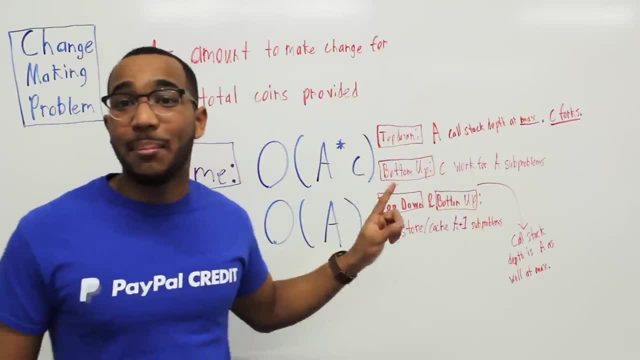 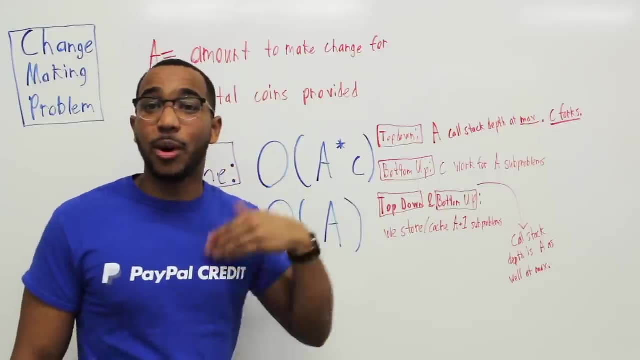 And at each of the points in the table, we're going to be trying at maximum C coins. We're going to try at maximum all the coins we have, as you saw in our example. That is why it is A times C for both the bottom-up and the top-down approach. 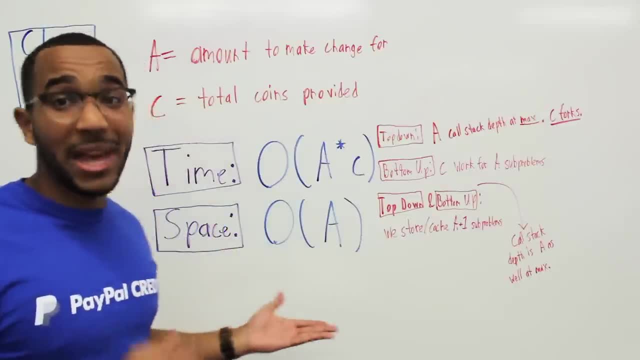 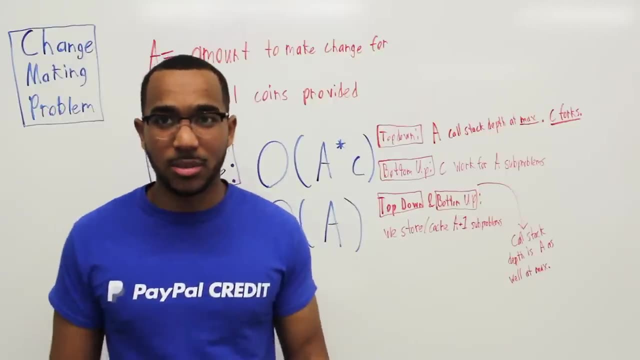 So let's look at the top-down, bottom-up for space. For space, we're going to be using O of A For both approaches. we're going to be caching the answers to A plus 1 subproblems. We're going to keep the answer to the 0 subproblem. 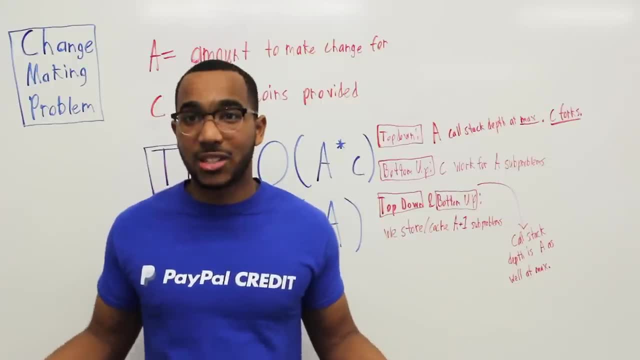 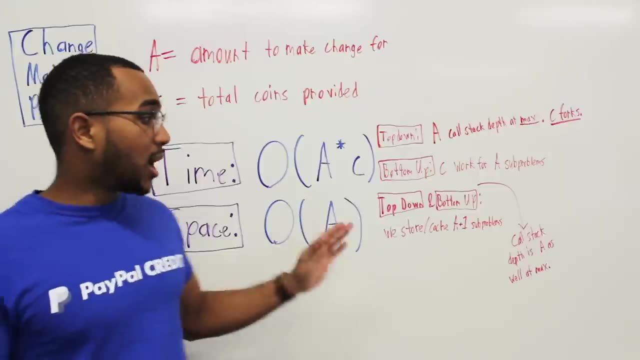 You could count that in, count that out, But it's going to be about A subproblems For the top-down and bottom-up. we're going to have this dynamic programming table that caches A answers, But the call stack for the top-down approach, which is recursive, is going to have at max a depth of A. 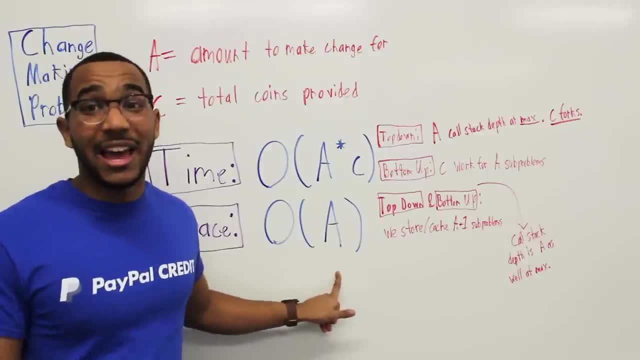 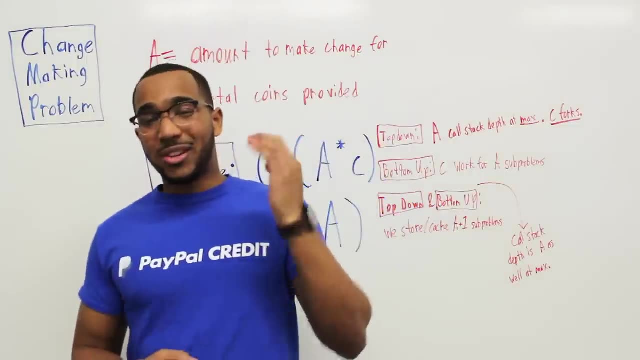 That does not change our space complexity. That still keeps it at O of A. So this is the time and space to this problem. So that is all for this problem. If you like this video, if this was a clear explanation, subscribe to the channel and like this video. 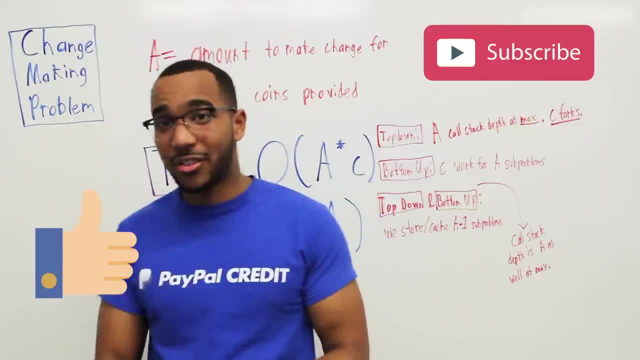 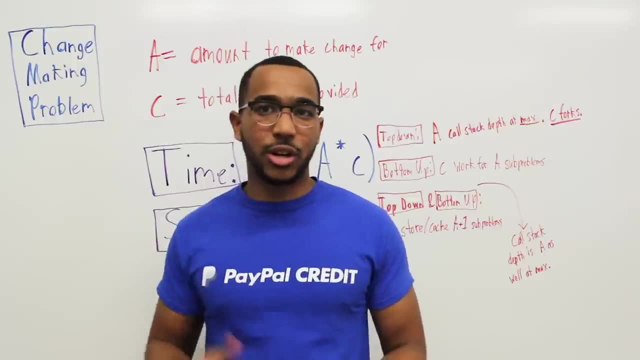 I want to do videos like this every day to help engineers prepare for the interview. Questions like this on a day-to-day basis are not really that practical For someone who's in industry or working, So I really want this channel to be a resource to refresh people's minds. 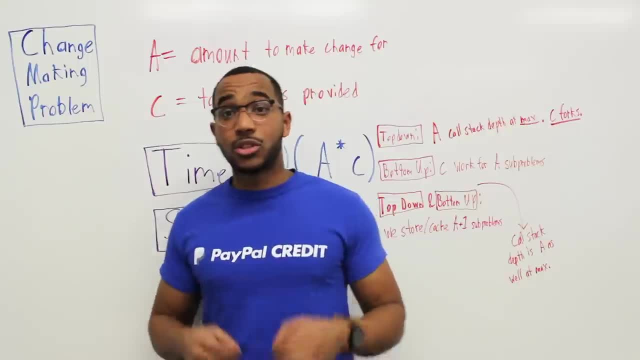 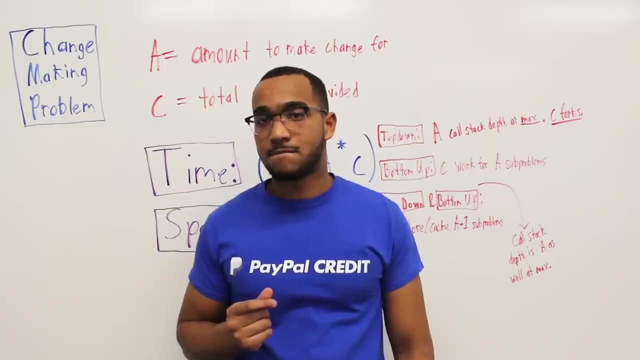 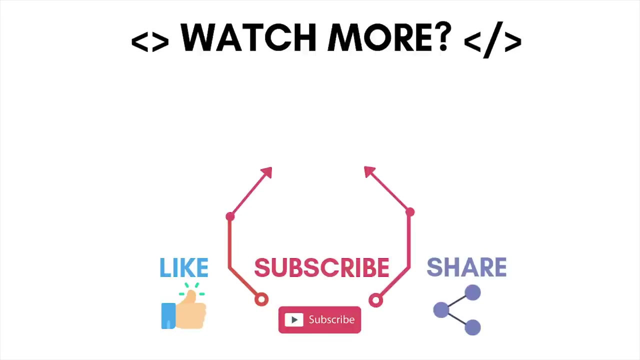 And help them prepare for this process of interviewing. So that's all for this video and See you in the next video. Bye. 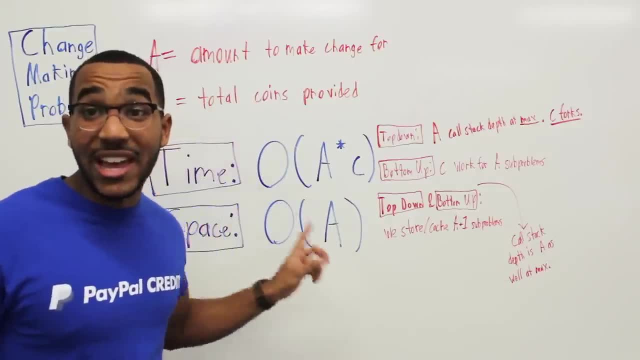 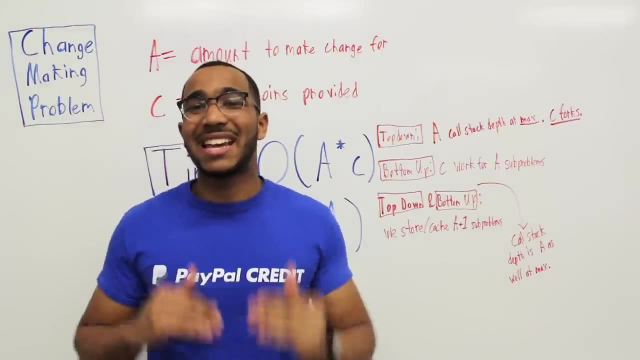 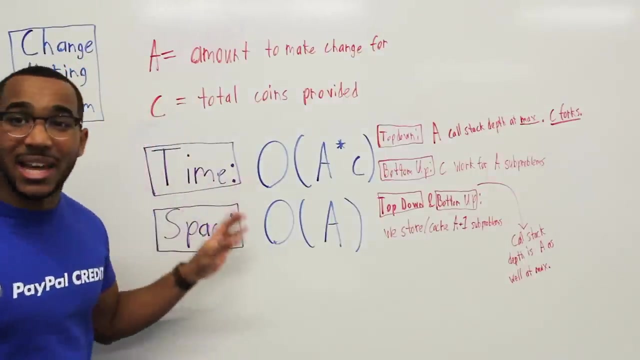 we're going to have this dynamic programming table that caches A answers, But the call stack for the top-down approach, which is recursive, is going to have at max a depth of A. That does not change our space complexity. That still keeps it at O of A. So this is the time and space to this problem. So that is all. 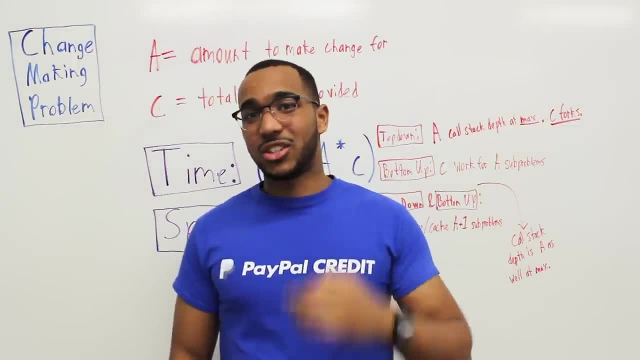 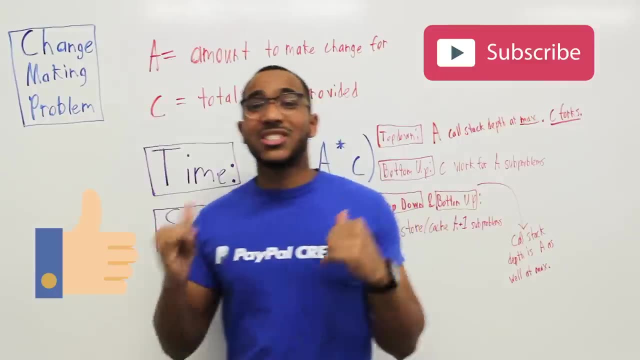 for this problem. If you like this video, if this was a clear explanation, subscribe to the channel and like this video. I want to do videos like this every day to help engineers prepare for this. After the interview. questions like this on a day-to-day basis are not really that. 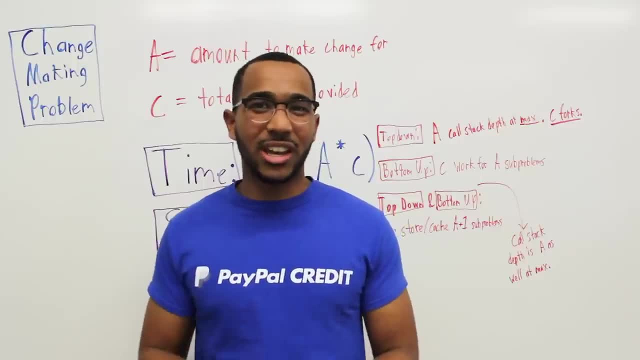 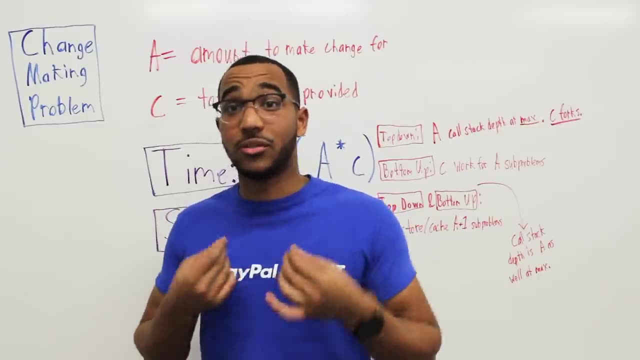 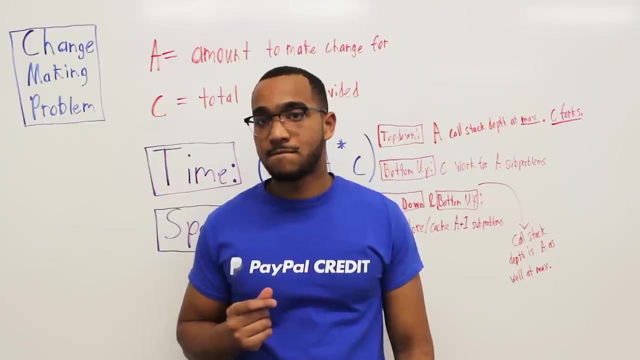 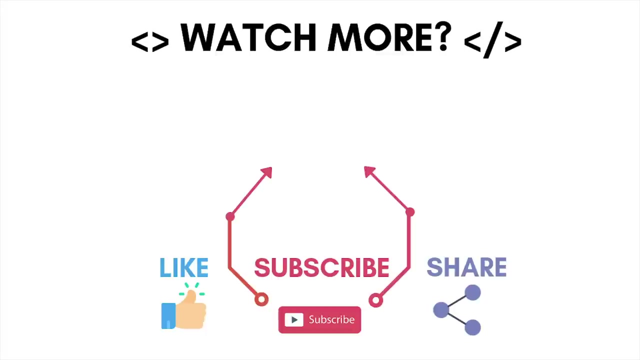 practical for someone who's in industry or working. So I really want this channel to be a resource to refresh people's minds and help them prepare for this process of interviewing. So that's all for this video and I'll see you in the next one.